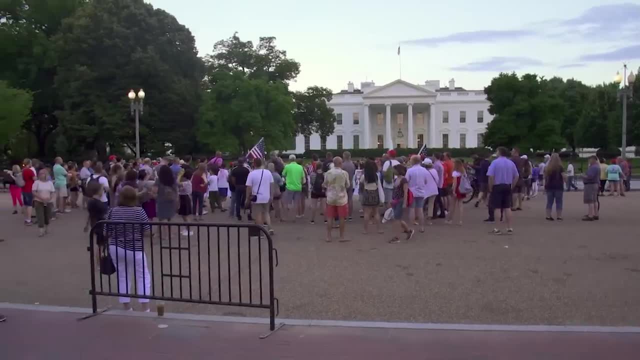 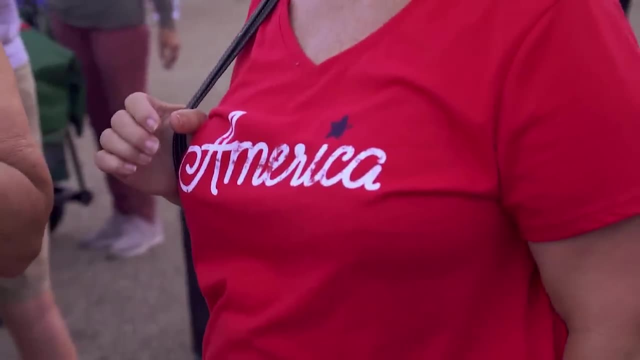 said you. you're the fighter that I need and you're going to save the soul of this nation that I inspired the founding, and God bless him for that. Seventy percent of Americans are Christians. The majority of them voted for Trump. 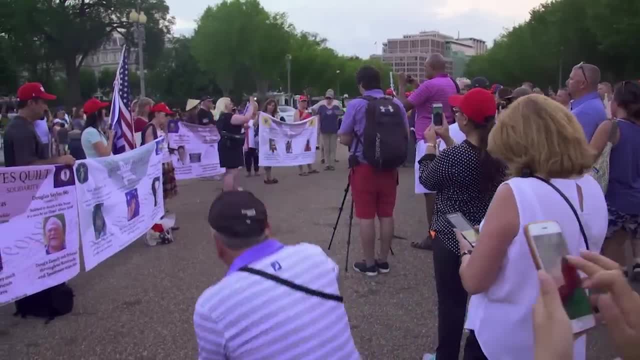 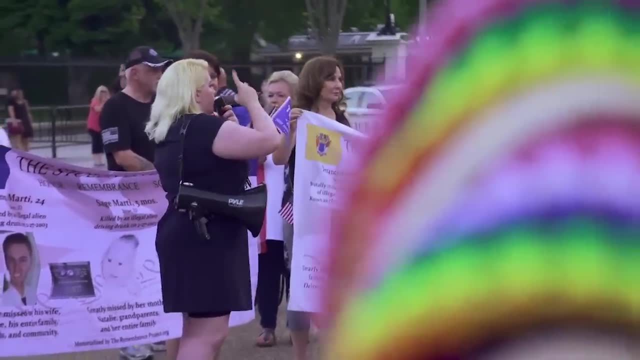 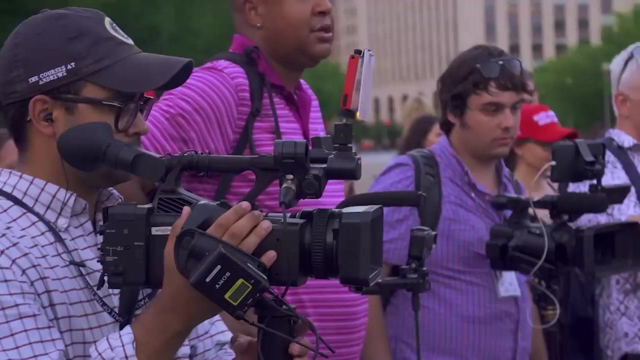 But I will say in the name of God, In the name of Jesus Christ of Nazareth, that we plead the precious blood of Jesus to put a hedge of protection around Donald J Trump, the president of the United States of America, to put a hedge of protection around First Lady Melania and all the socialists. be damned. 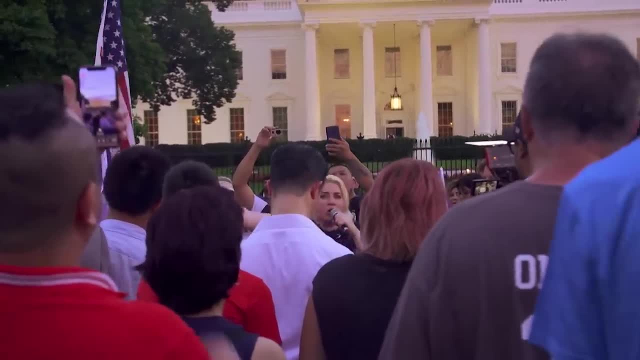 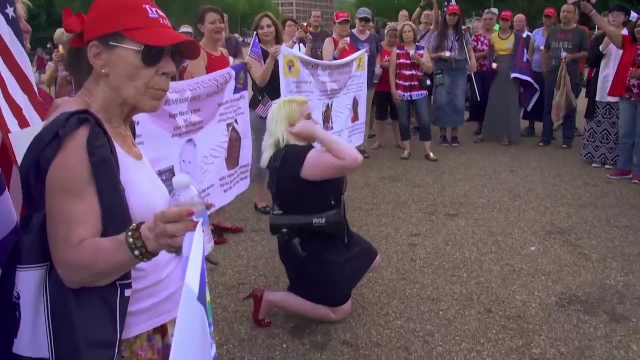 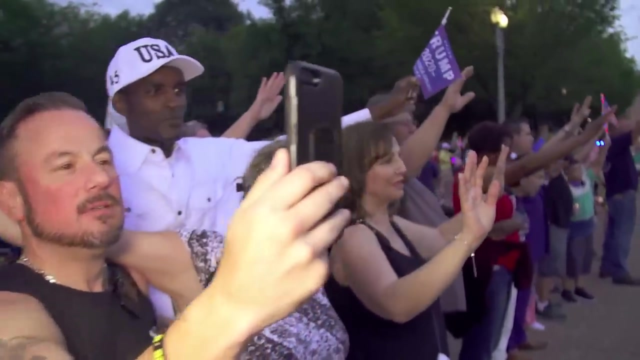 and all the evildoers be damned. God made this country. Donald Trump is protecting what God created. We can get down on our knees and say thank you, Thank you, Thank you Jesus, Thank you Amen. Donald Trump, the Republican president, has announced that he will run again in 2020.. 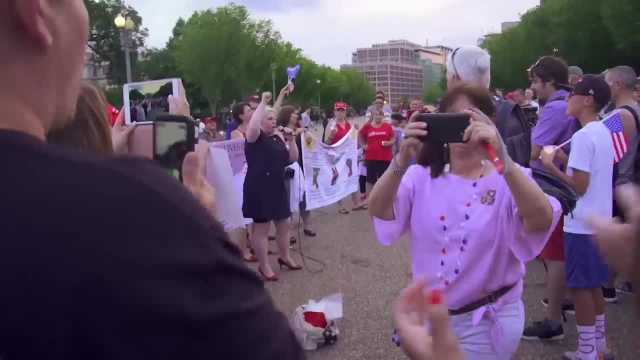 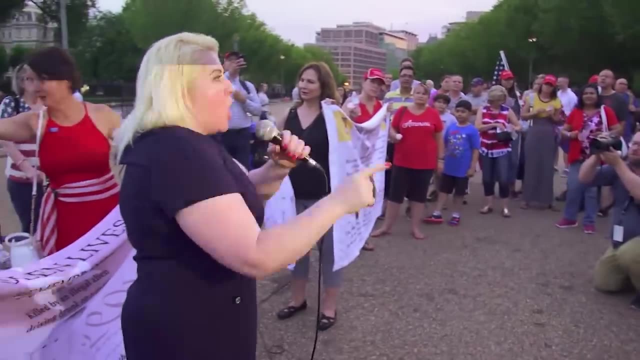 The Christians are already mobilizing for his campaign. Trump 2020!, Trump 2020!. We either fall into darkness and the rest of the world goes with us, or we re-elect Donald Trump in 2020 and save the rest of the world by saving America. 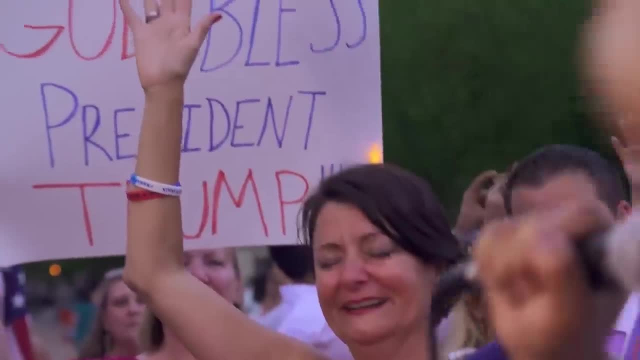 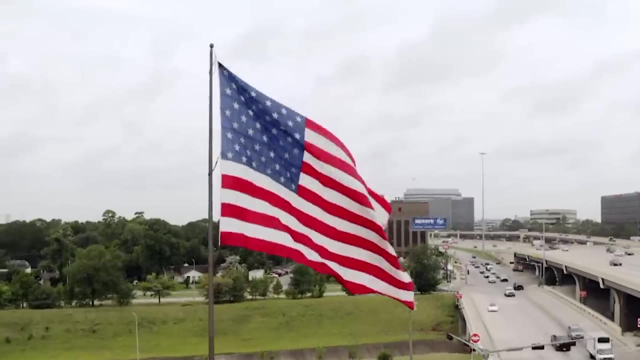 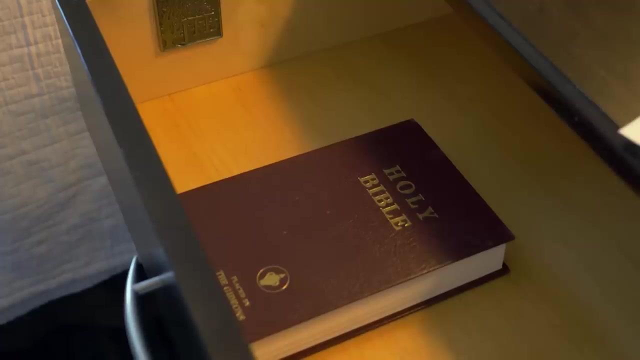 Yay, He is gone. He is gone. Praise God. Praise God. Despite officially being in a secular country with no mention of God in the constitution, religion is everywhere in the United States, In every hotel room, On every dollar bill. 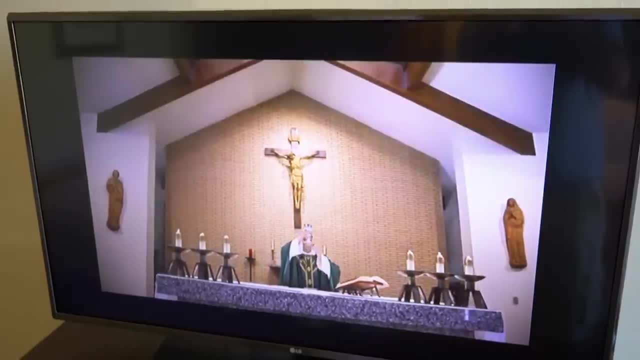 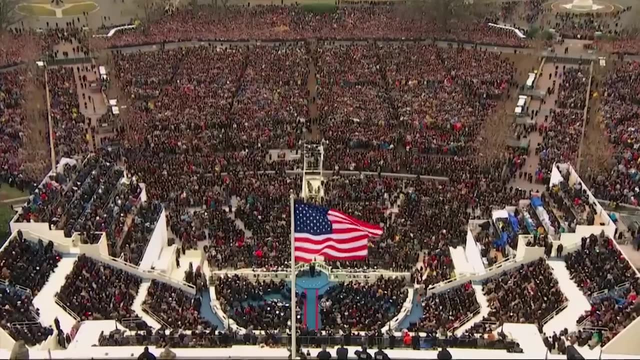 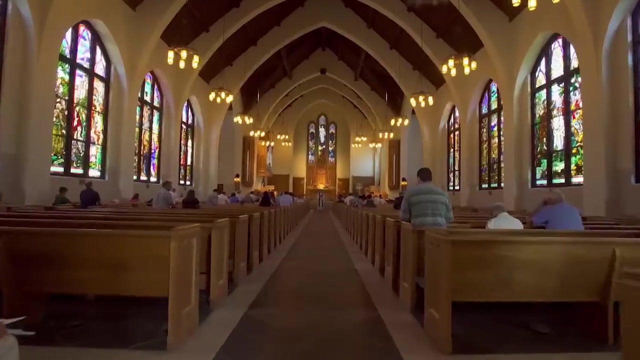 On the radio, On TV, Thousands of Christians take Cruises for their vacations. On billboards, boards and in political speeches. God bless you, God bless America. In today's society, evangelists are the most powerful amongst the Christians. 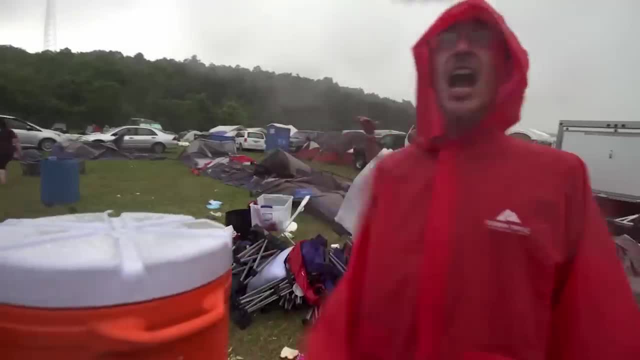 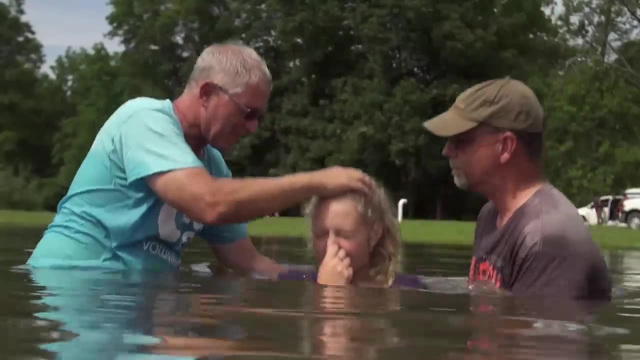 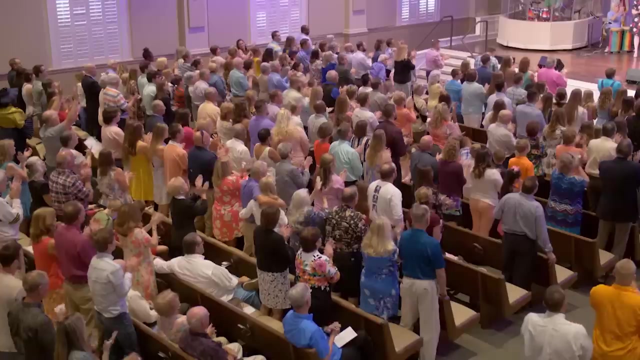 with almost 90 million of them living in the US alone. Jesus Followers in this Protestant sector are also known as born-again Christians. For the first time in American history, they mobilized in their masses to get Donald Trump elected, And they are now gearing up to do. 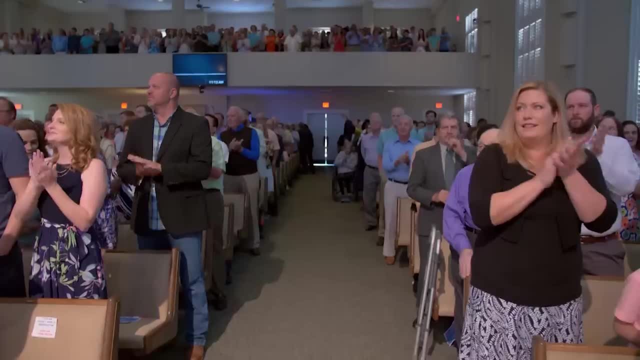 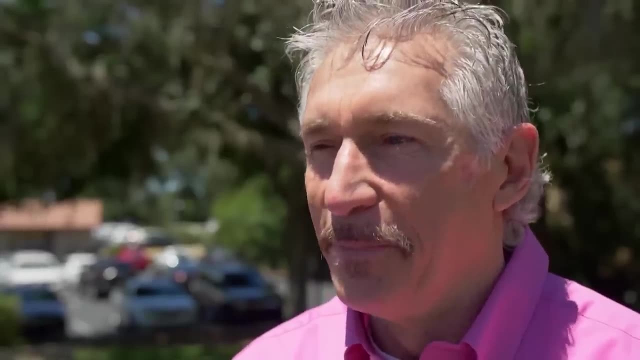 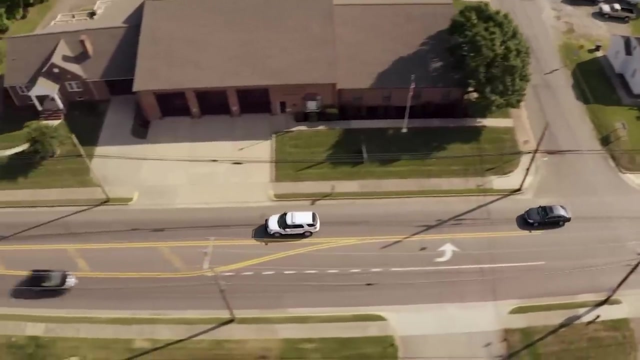 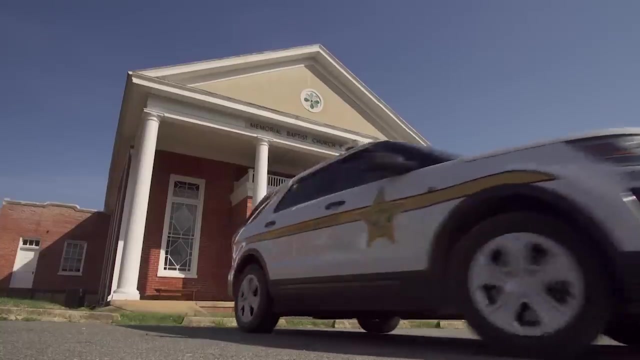 the same for the next election. I voted for Trump. I have no question that I believe he's an instrument of God. Religion has found its way into every part of society, even in law enforcement. Mark is a pastor. Hey, Daniel, let's go. 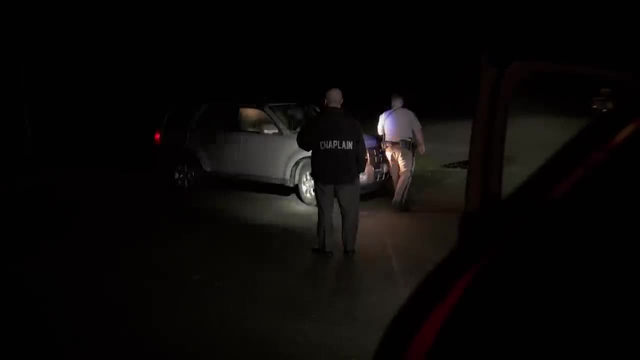 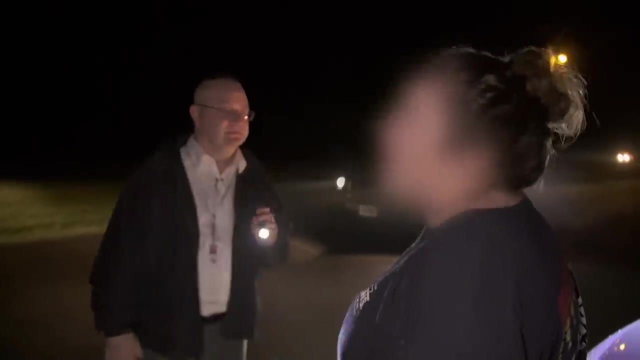 He is heading out with the local sheriff to preach to the suspects during their arrest. We get to pick the sin that we want to do, but we don't get to pick the consequence or when it comes. I'm so scared. Evangelists have even created. 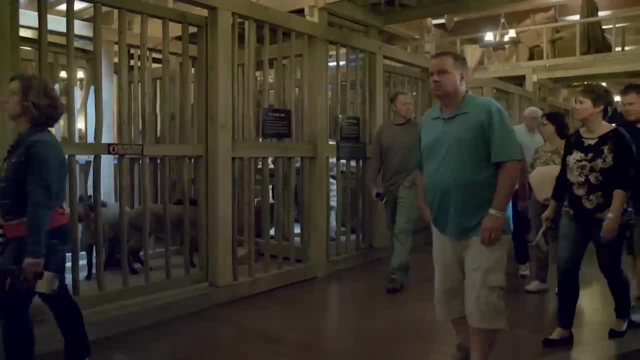 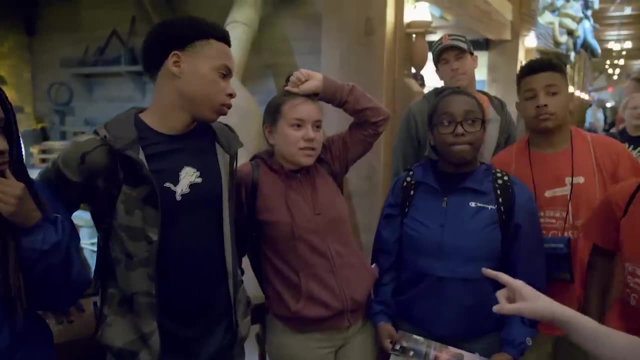 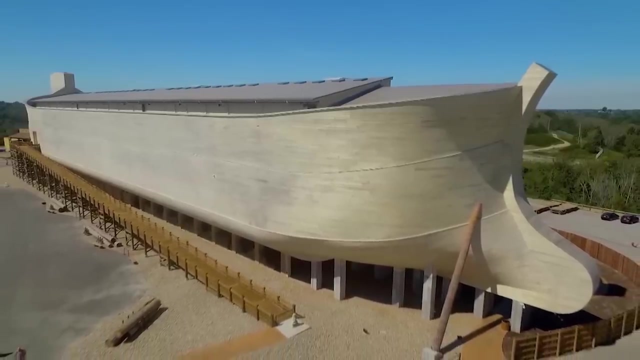 their own Bible-themed attractions, boldly rewriting the science books to educate their children How old Noah was when he entered the ark: 600 years old, It's just the body, aged differently back then. In Kentucky, a life-size Noah's Ark has been built, along with a museum that supports the ark. 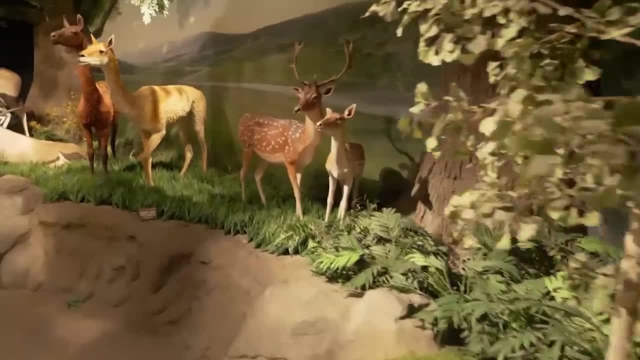 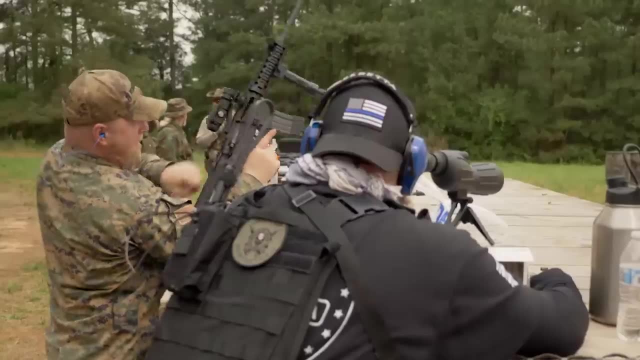 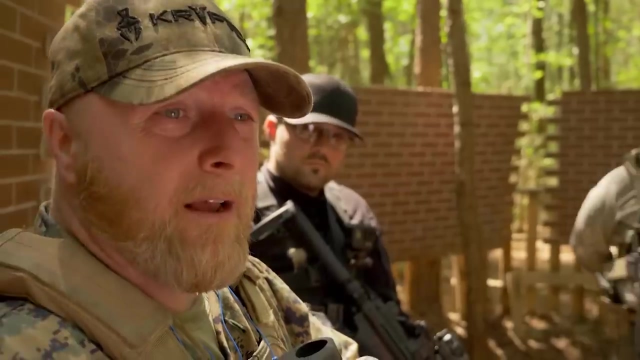 It's a big ark. It supports the theory that the universe was created in just six days, attracting tens of thousands of visitors. Over in Georgia are militia who dream of an entirely Christian nation. These men are ready to use force if necessary. I would die for my God. 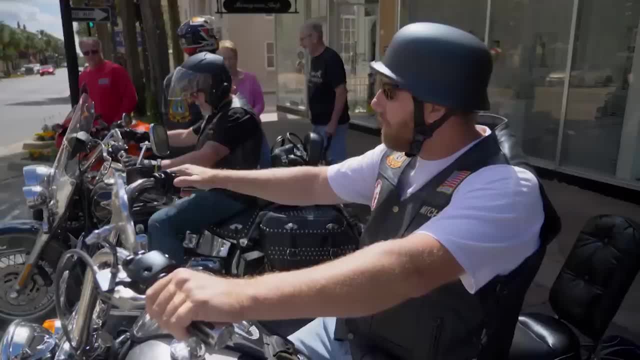 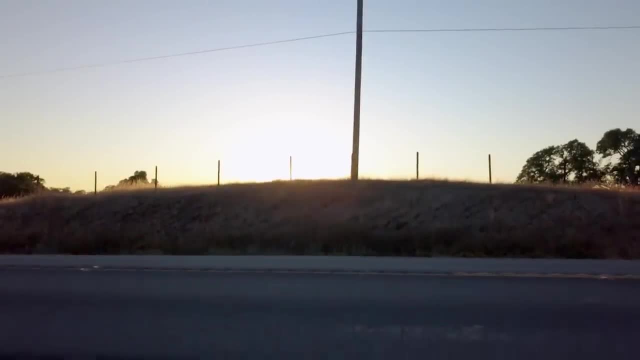 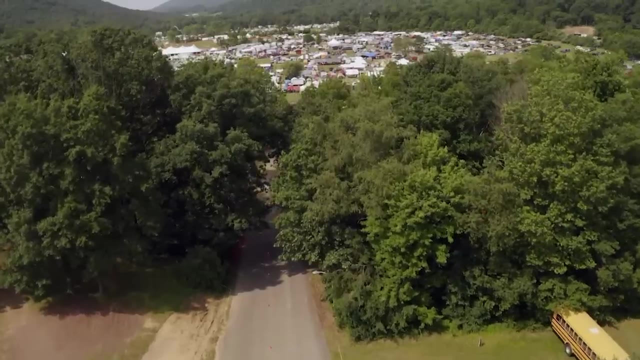 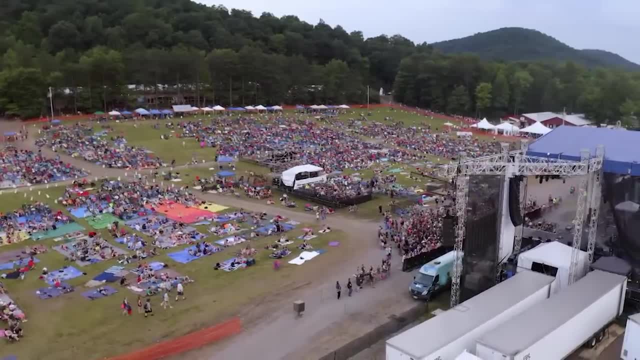 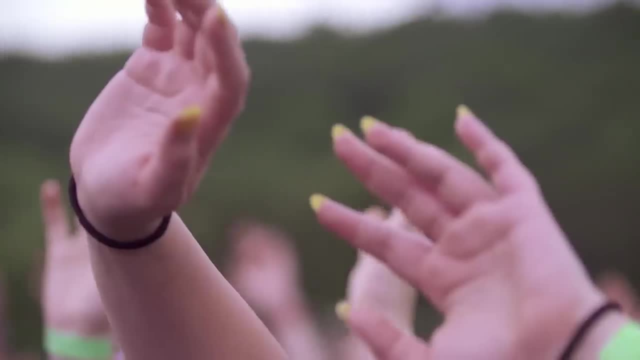 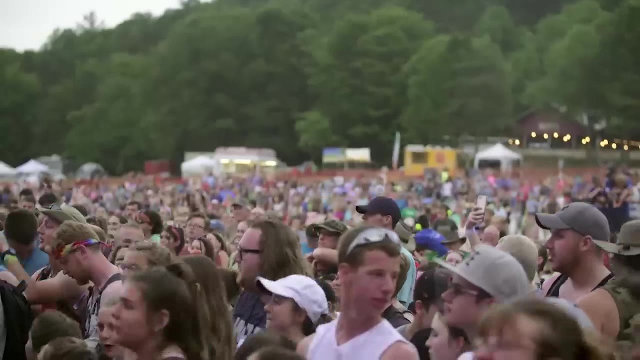 every year for a rather different music festival. Here the songs are only about one thing: Oh Oh. Nicknamed the Christian Woodstock Creator's Unlikely. Nicknamed the Christian Woodstock Creator's Unlikely is the biggest Christian music festival in the US. 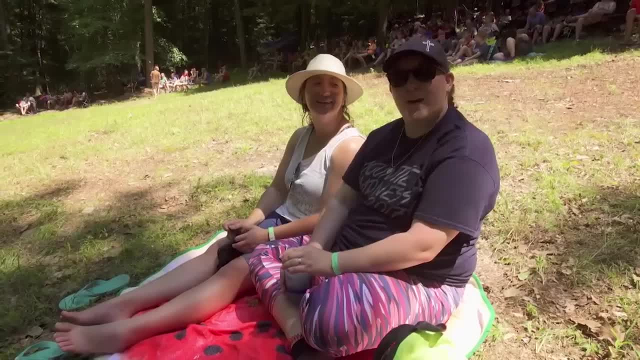 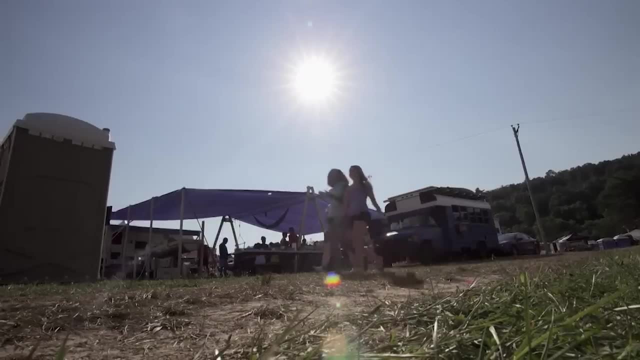 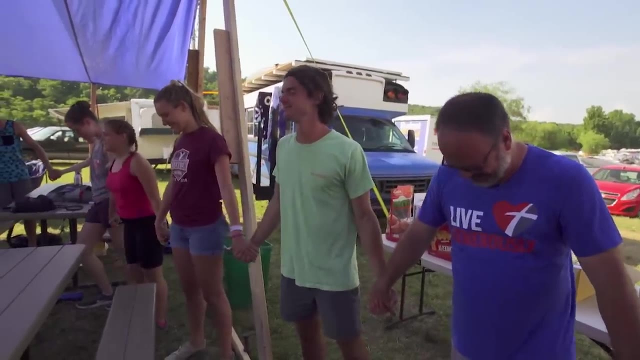 We love creation. It's very godly. You can't show up and not cry. Most of the festival goers are less than 25.. Thank you, Jesus. just for these past couple weeks, A lot of these young people are here with their church. 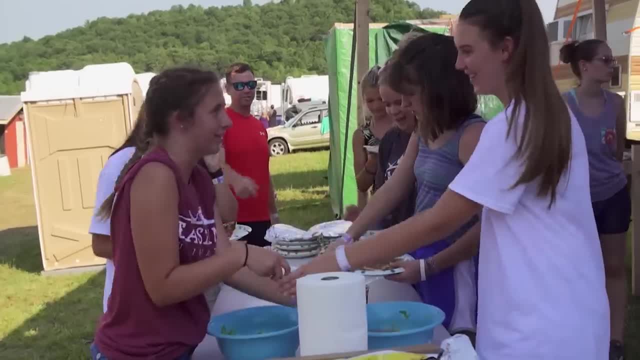 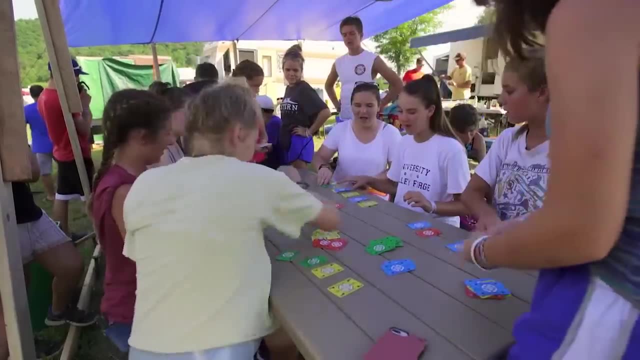 to pray and party. This is the case with 18-year-old Zoe. Her group have traveled for 17 hours by bus from Florida. Ah, I need a fork Here. young people are encouraged to have fun, but within reason, The festival has very strict rules. 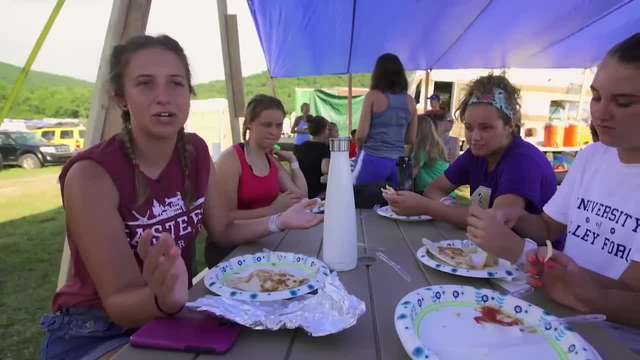 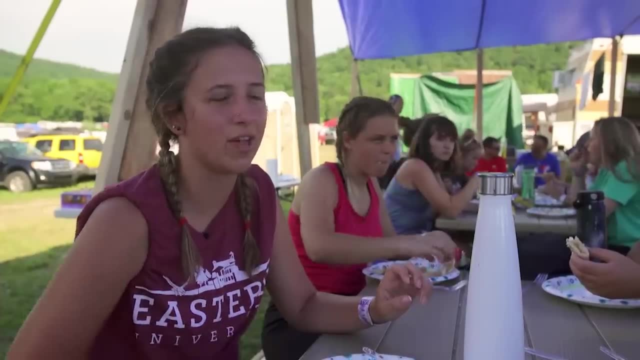 You're not allowed to be drinking or doing drugs and there is like a dress code like no, really short shorts, I don't think. yeah, spaghetti straps, you're not supposed to have cover your stomach, Okay, so, ladies, you guys having fun. 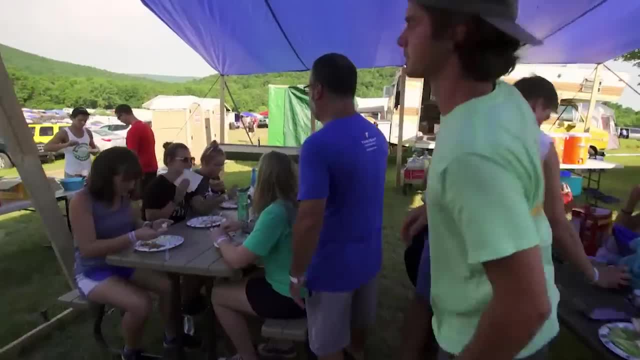 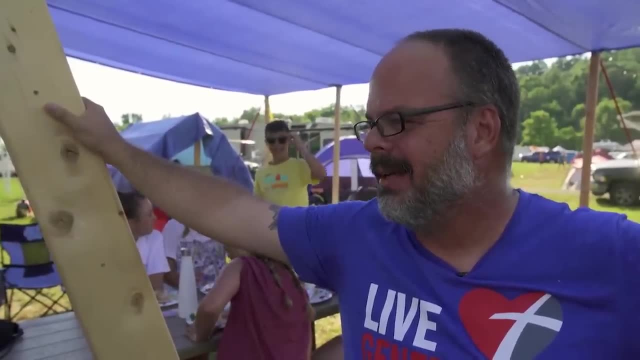 You got a little something right here. Zoe and her group are here with their pastor, Mike. The music that's out there now is definitely engaging, you know, the young people and it's you know it reaches them on a whole new level. 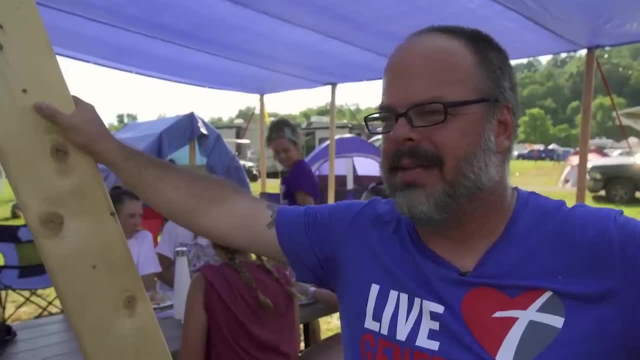 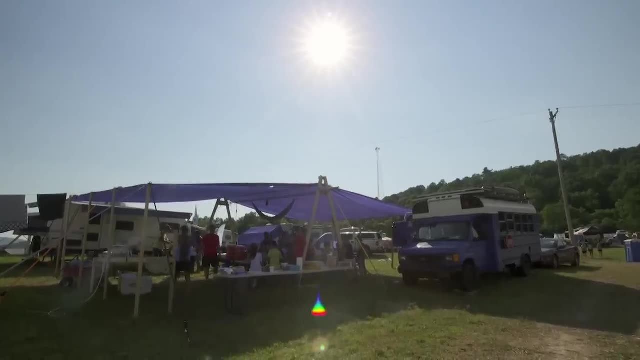 You know it gets into their world a little bit and they can understand. you know what they're saying, They can hear the words that God is, you know, speaking through the artists. Zoe has only just arrived and before the music has even begun. 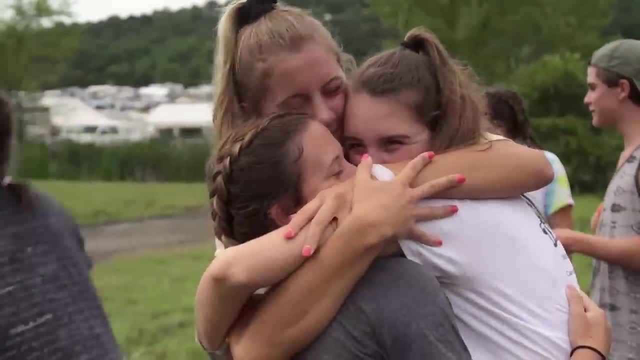 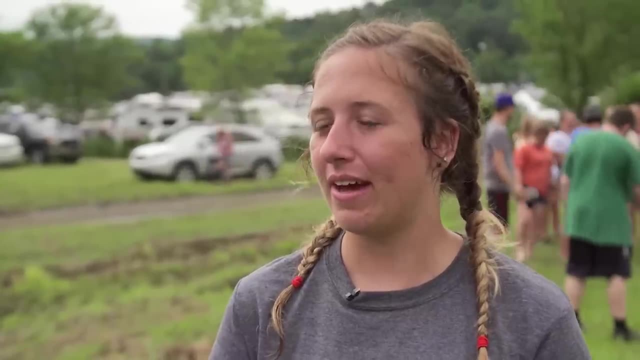 she's made a huge decision: She's going to get baptized. I decided to get baptized when I was about seven years old, but I don't remember it. and also recently I've kind of walked away from Christ and now I'm coming back into it. 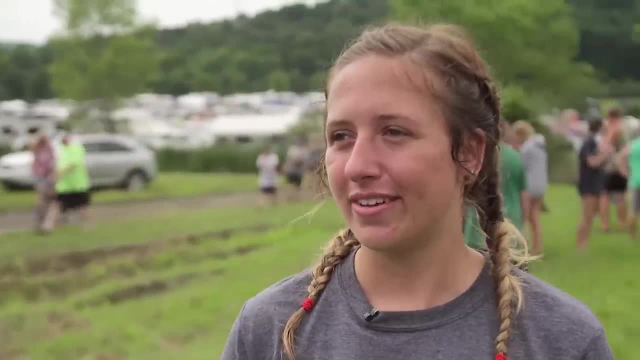 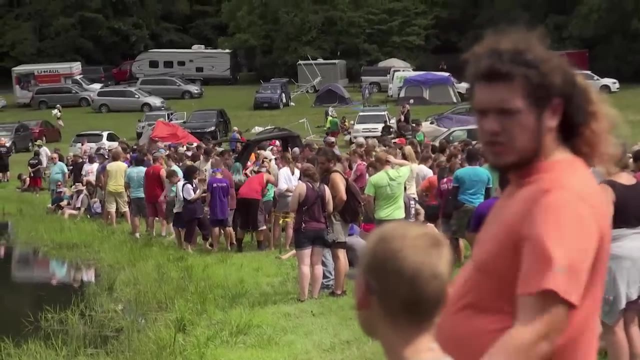 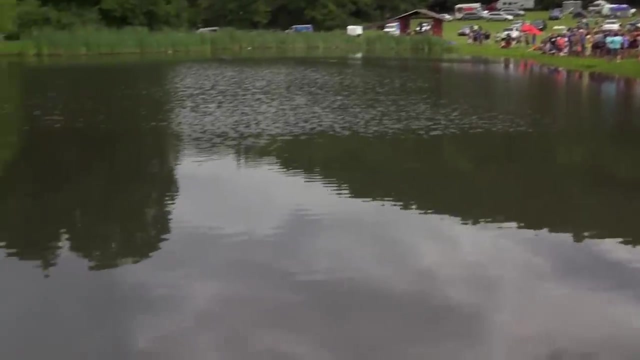 and I just want it to be a public declaration of: I'm giving my life to Christ. This is who I am Born-again. Christians can be baptized several times. Zoe has strayed from the path over recent years, partying, drinking alcohol and taking drugs. 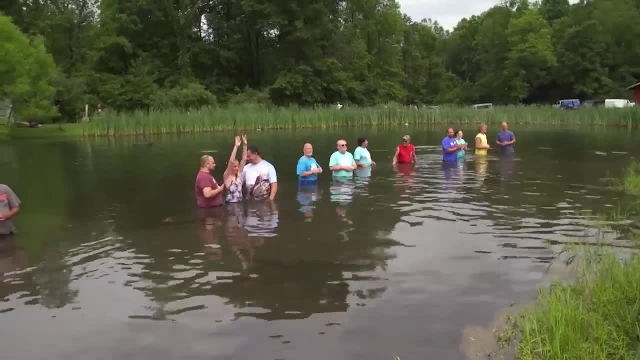 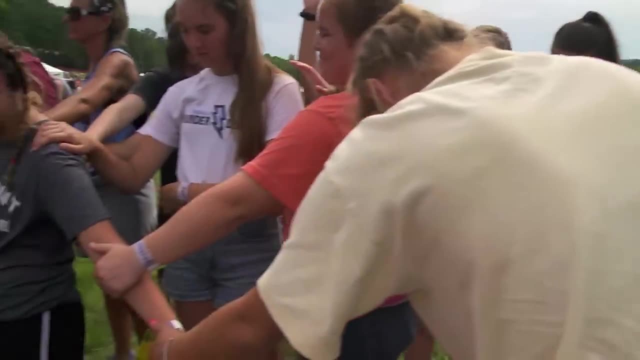 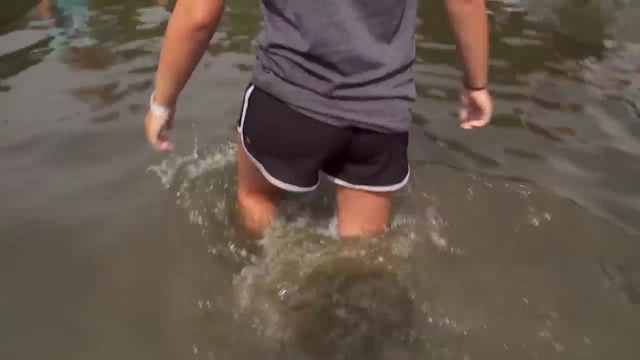 Raise your hand if you're here because you want to be baptized right now. Where are you at? For Zoe? her second baptism is a rebirth, a way for her sins to be forgiven. This is the born-again philosophy. Zoe, do you desire to be baptized? 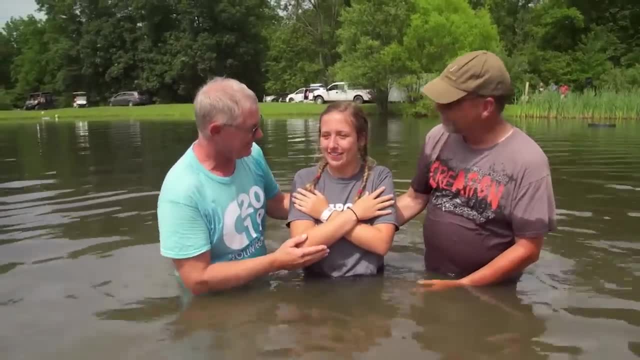 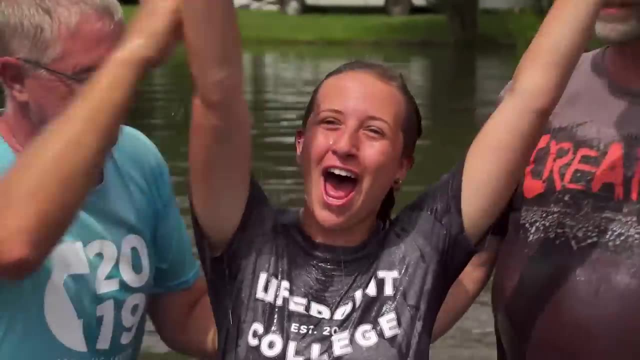 Yes, please Do you believe in Jesus as your Lord and Savior. Yes, Amen, Ready, Yes, Baptize your heart. Son and Holy Spirit, Whoo, Whoo, Whoo. That's cool, That's cool, That's cool. 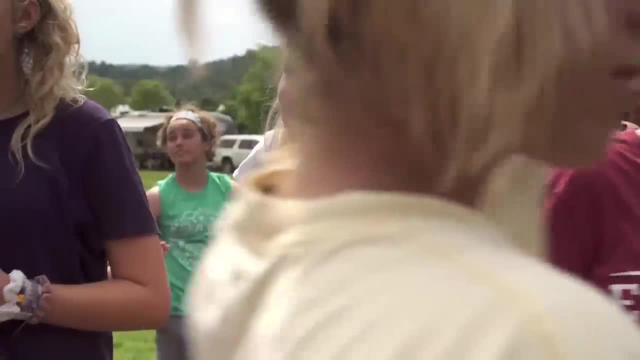 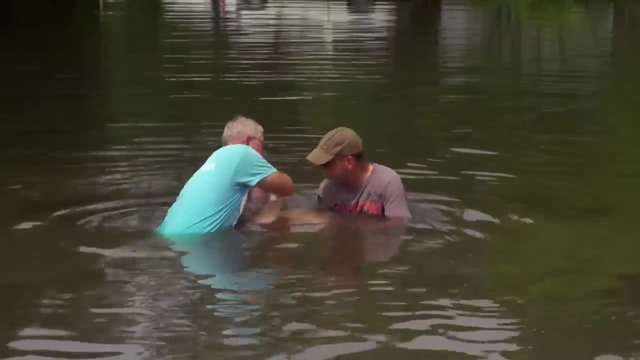 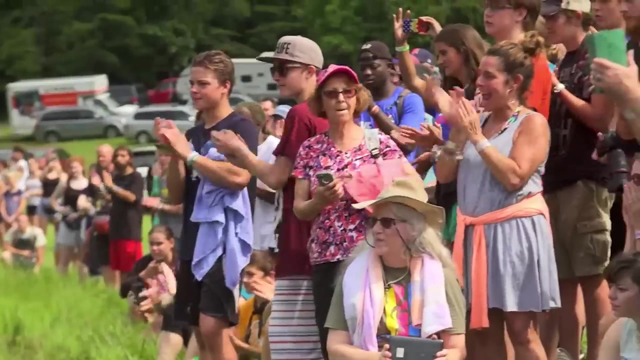 I'm feeling very happy and very excited and I'm glad I did that. I do feel like a new person. yes, The line of baptisms goes on for hours. Whoo Ready, Whoo, Whoo, Whoo. 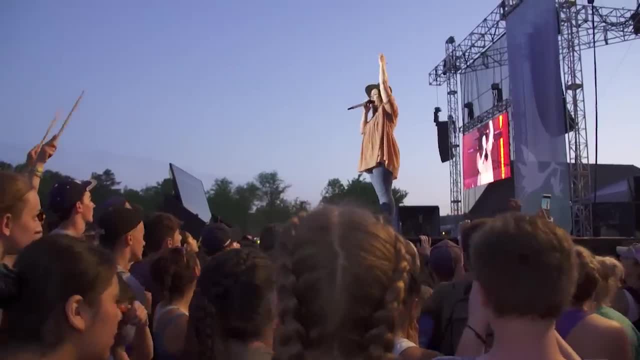 The day of the cross is coming. The day of the cross is come As night falls, As night falls. This is the presence of God that has come to show энергize to me. We find Zoe and her group amongst the crowd at the concert. 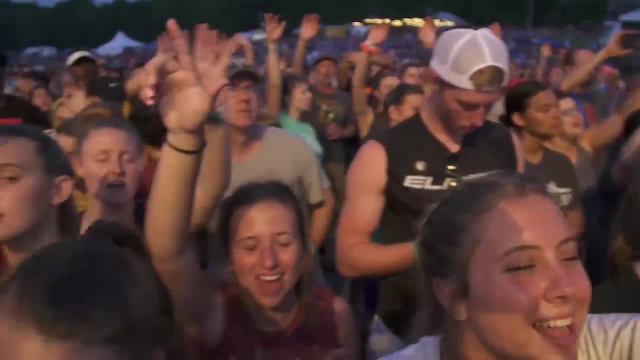 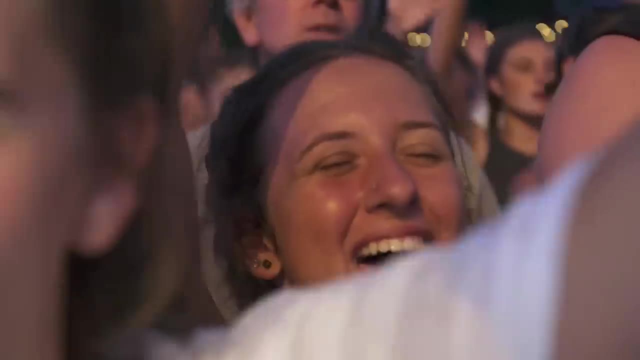 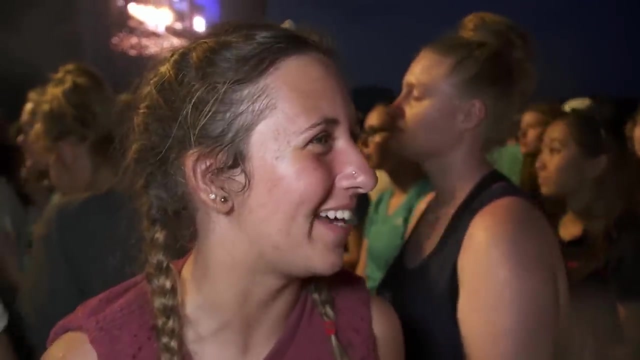 The day of Jesus. Break every chain. break every chain. break every chain. These girls are loyal fans. They know all the words to every song. It's indescribable, I don't know, like the echo off the hills and just having a hard time. 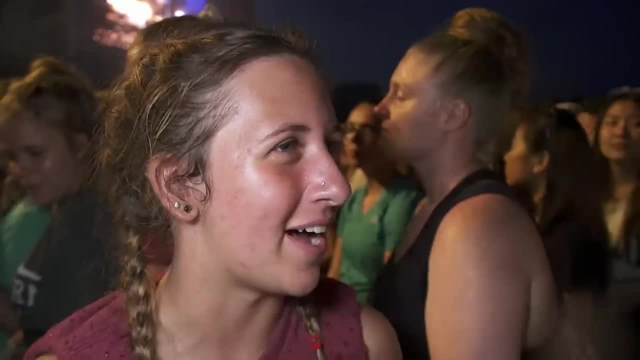 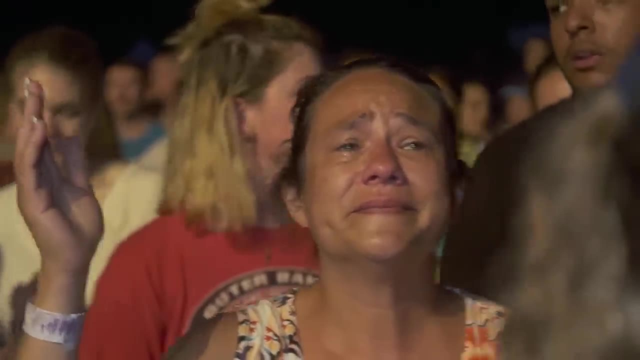 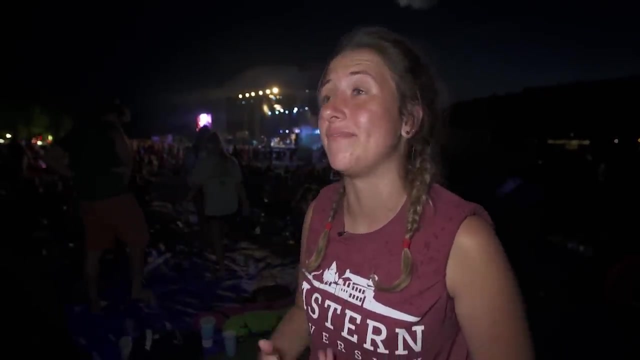 the hills and just having so many people around, like worshiping God, is unlike anything you'll ever experience. The crowd is truly overwhelmed. If I'm being completely honest, I've been through drugs, I've been through alcohol. nothing compares to what I'm feeling right now. 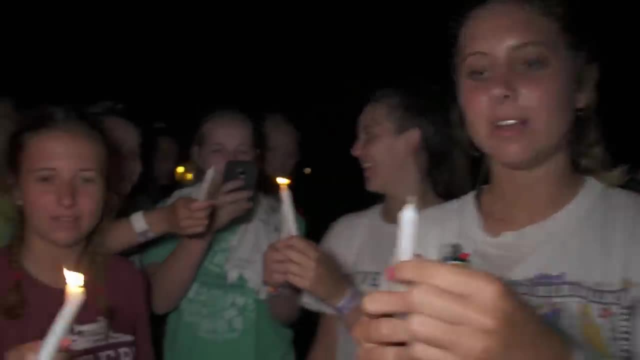 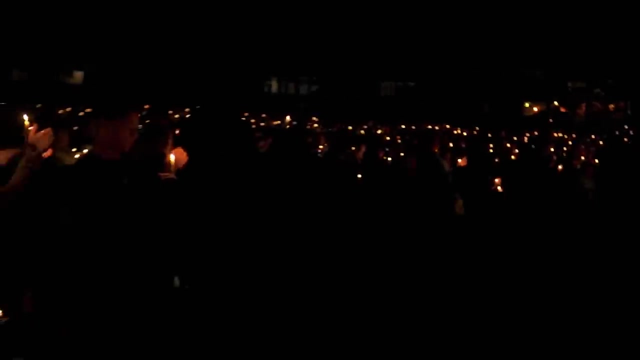 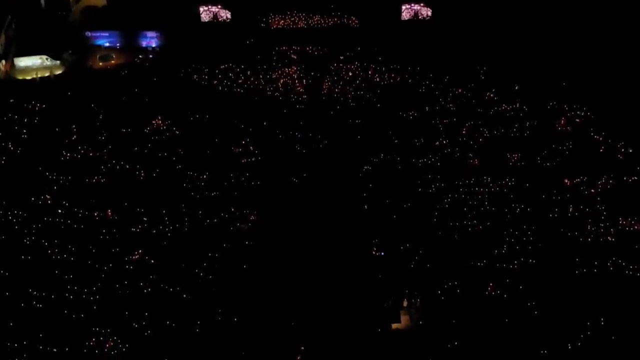 Despite the mistakes made in their former lives, these born again Christians believe they are here to save the world, even if this involves denouncing the non-believers. So the lighting of the candles is symbolic of how Jesus calls us the light of the world. 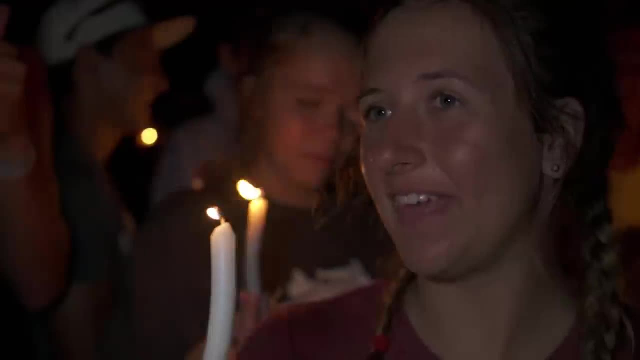 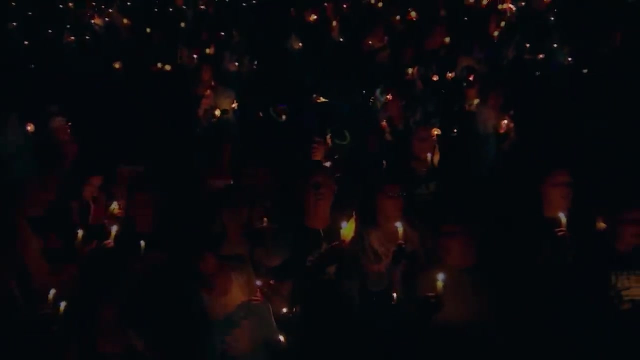 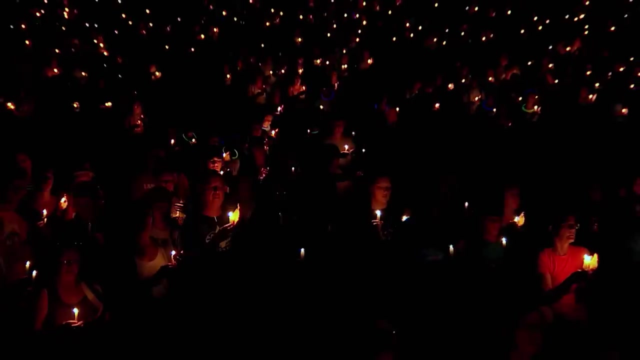 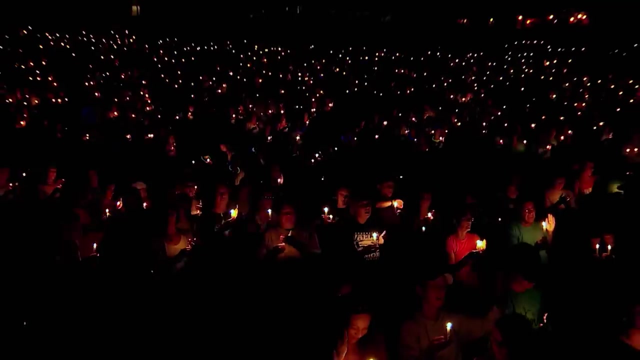 So we're bringing light to the dark places of the world as Christians. The other people are the darkness. Sing with me how great is our God, and all will sing. how great is our God, How great is our God. Sing that one more time. how great is our God. 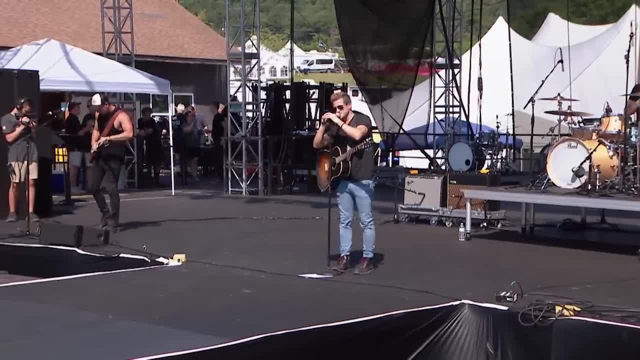 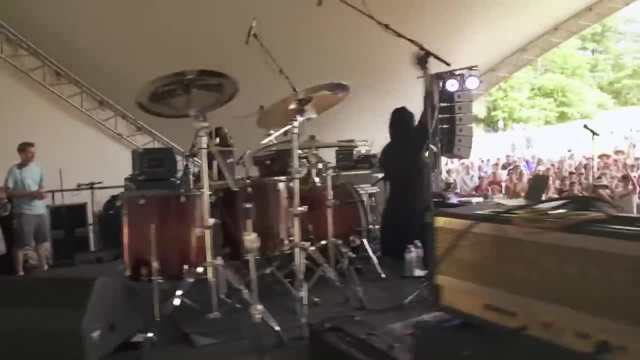 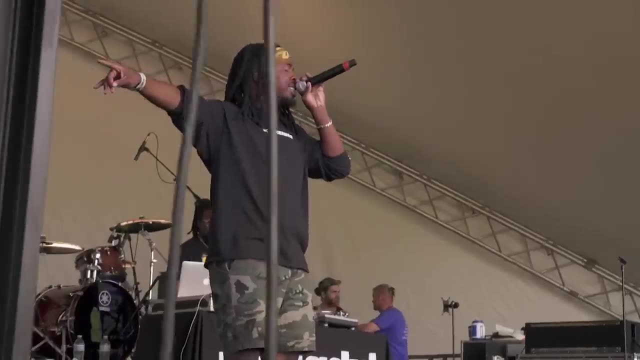 There's something for everyone. on the main stage the next day, Bible says that he loved us first. From self-righteous boy bands to stylish rappers, No Big Deal is a rising star who preaches God's word through his work. Only God could judge. but do you wanna see him litigate? 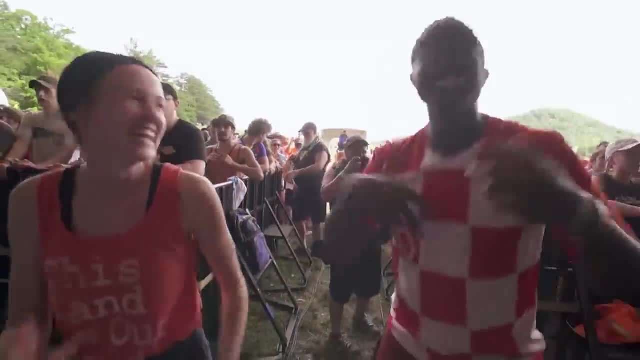 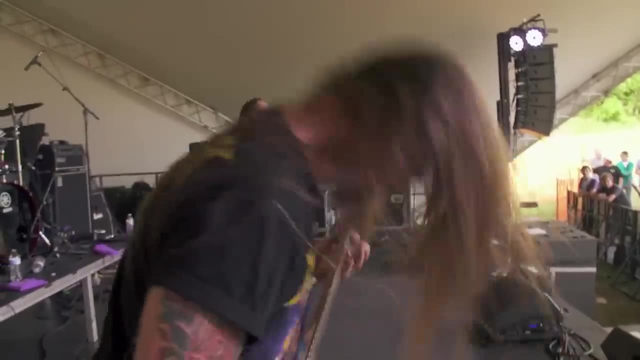 Will he pay? Will you get? no play around my real estate. There are also Christian metal groups at war with Satan. He's nothing but a garbage dump to get rid of. The battles are over. The whole world is wild and he does darkness in hell. 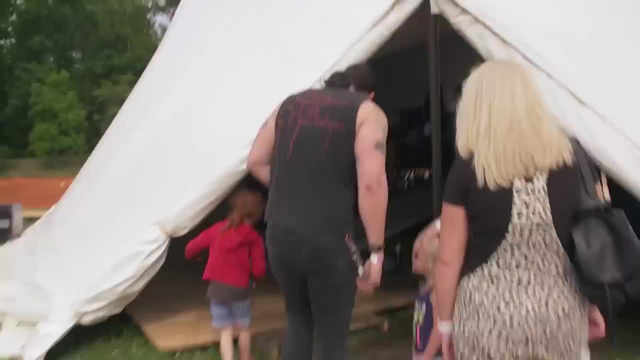 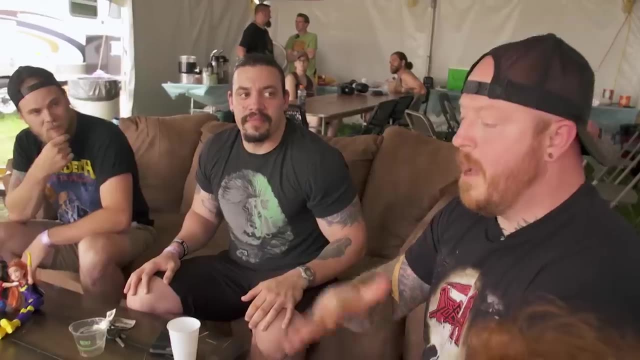 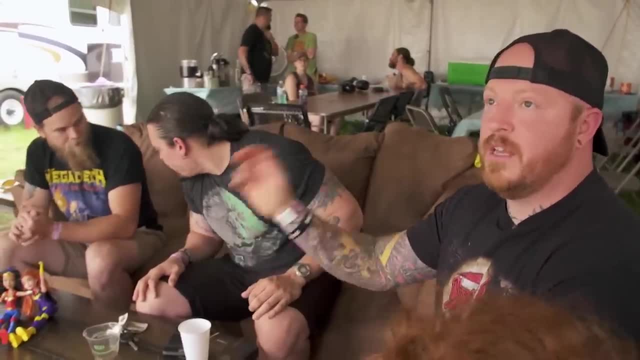 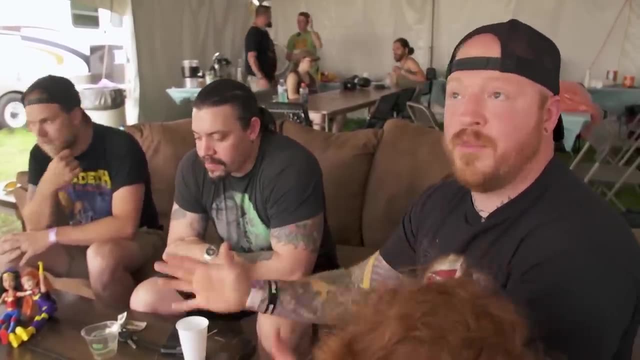 I wasn't always a believer. My father was a drug dealer, leader of a white power supremacy gang. I grew up with that kind of storyline. in my life I've personally been abused, kidnapped. I've been through a lot in my life. 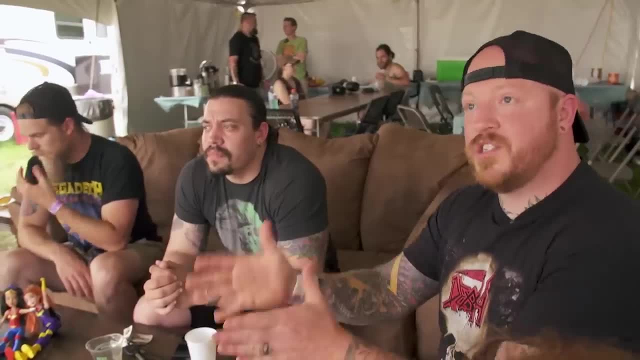 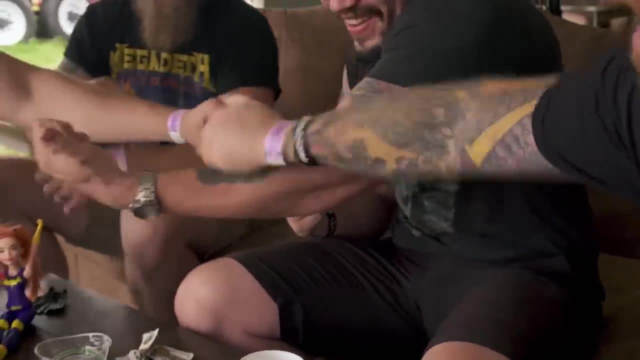 And then, as I got older, I just want to be a better dude. So that's where it started, and then molded into Christianity. Like many born-again Christians, Leroy has a difficult past. His spiritual rebirth has reinforced his faith. 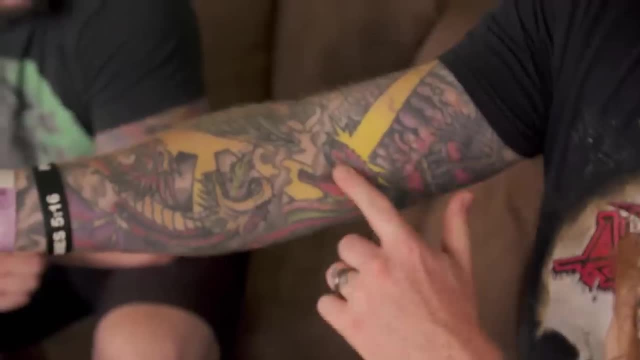 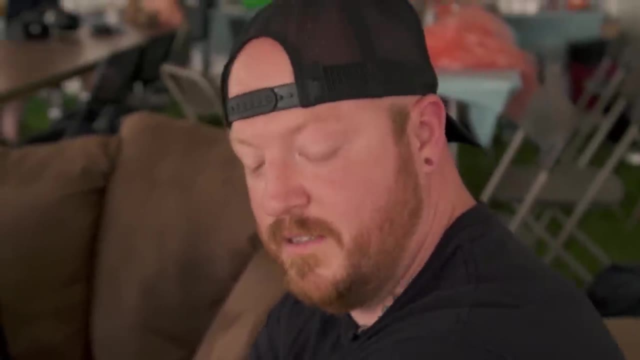 especially when expressed through his metal music. This is Seven-Headed Dragon of Revelation Fighting the Archangel Michael, And then this is the Beast Coming Out of the Abyss Fighting an angel as well. This Christian metal group holds all the conventions of the genre. 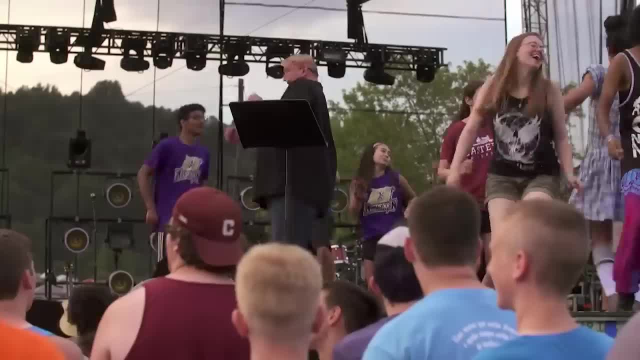 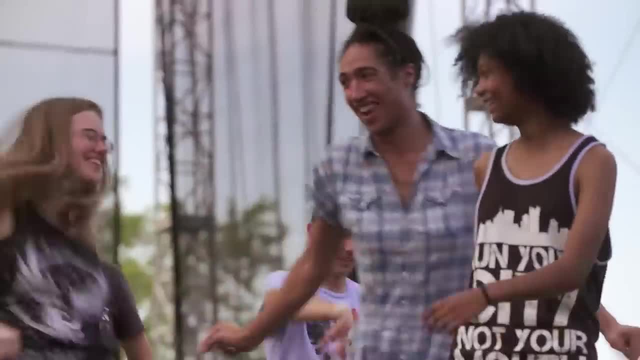 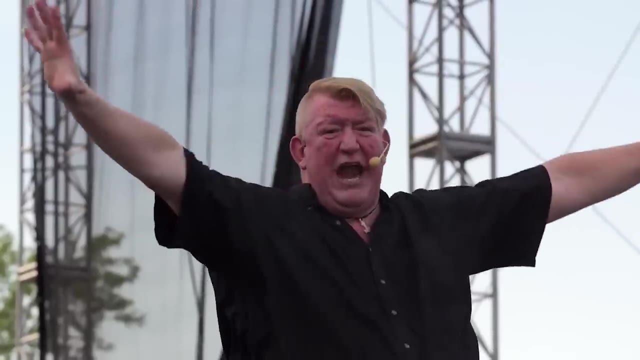 The Christian music industry is huge. Every year these songs are played over 170 million times. But behind the performance there is always a very clear political message: One day, every key, Every year, it's going to be wiped away. 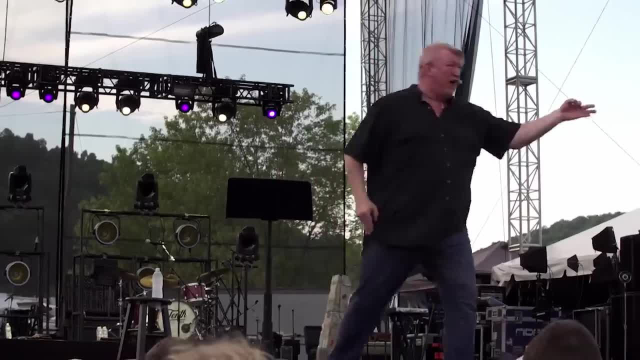 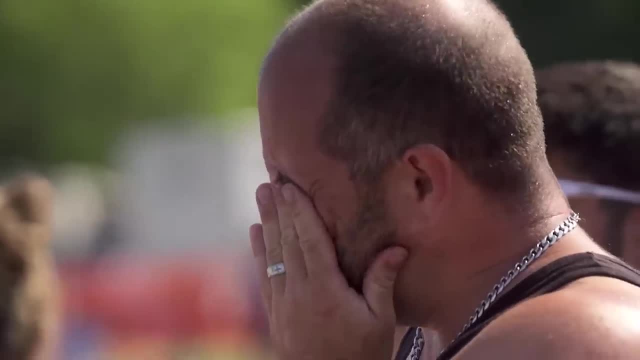 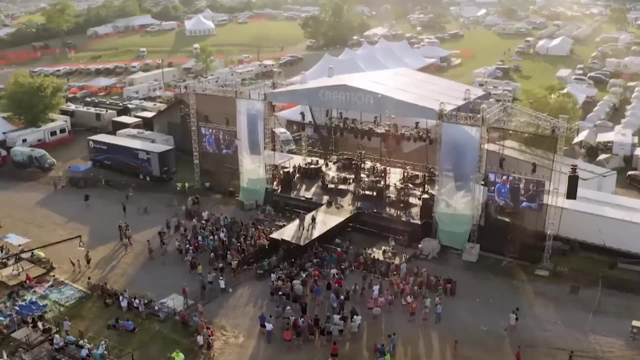 And there's going to be no more cancer and no more heartache and no more starving children and no more abortion. There is a day that's coming: The first controversial issue banning abortion. The festival is sponsored by Save the Storks. 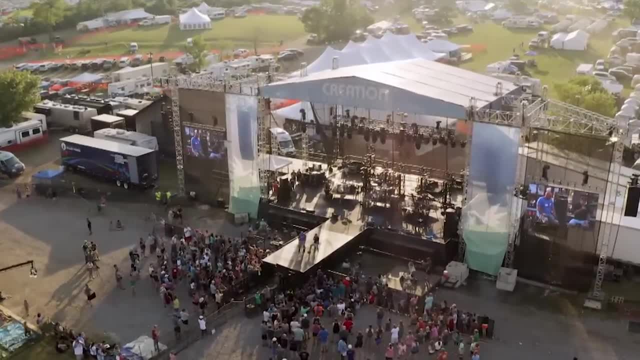 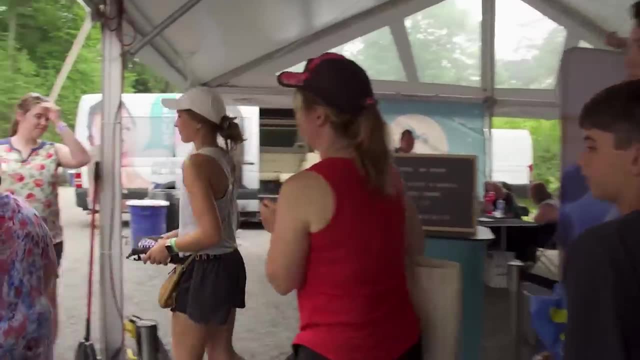 an anti-abortion non-profit. Their logo is even plastered across the main stage. Hi, if you guys are waiting to get on the bus, go ahead and come on. Anti-abortion campaigners are everywhere at the festival, So hi, everybody. 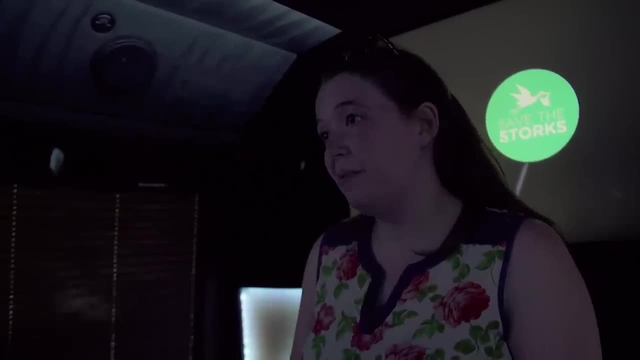 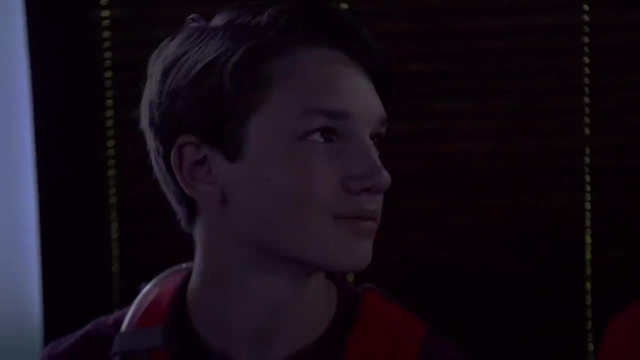 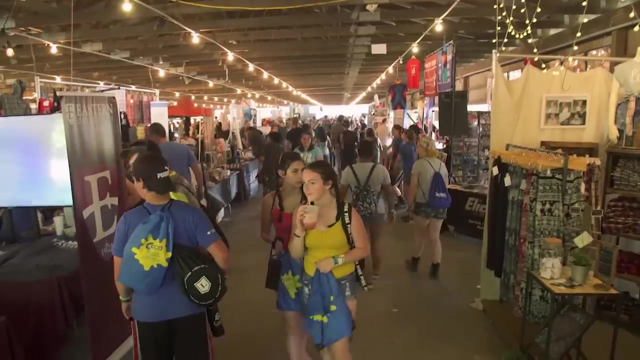 Yeah, so we have just a couple of videos. Our mission and our dream is to make abortion unthinkable, And every day, over 1,788 of those pregnancies are terminated. The non-profit doesn't shy away from strong, even shocking, symbols. 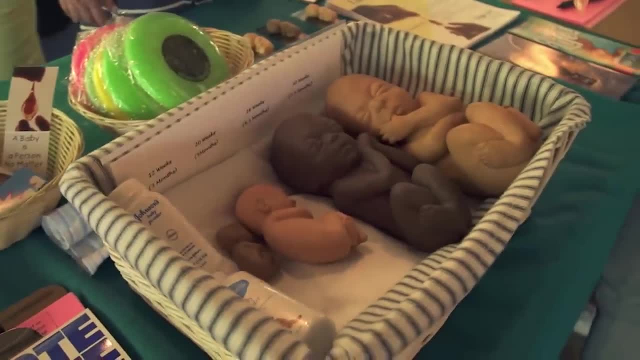 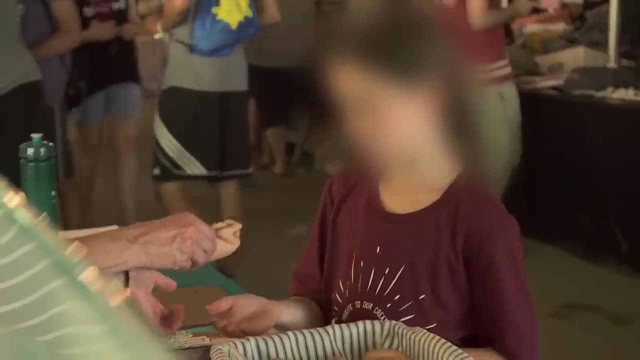 They give out three rubber fetuses to the youngest children. Here's a 20-week-old baby. another week or two or would be able to live outside the mother. You want to hold out your palm of your hand. see if it'll fit in yours. 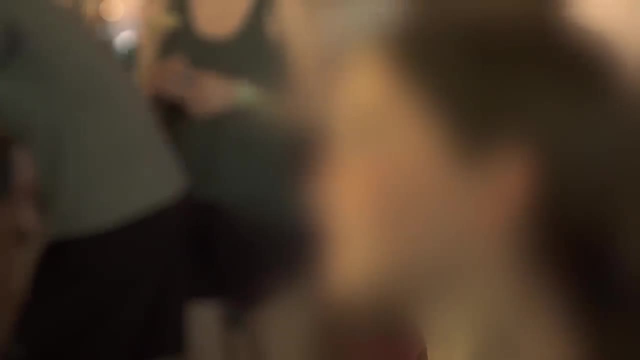 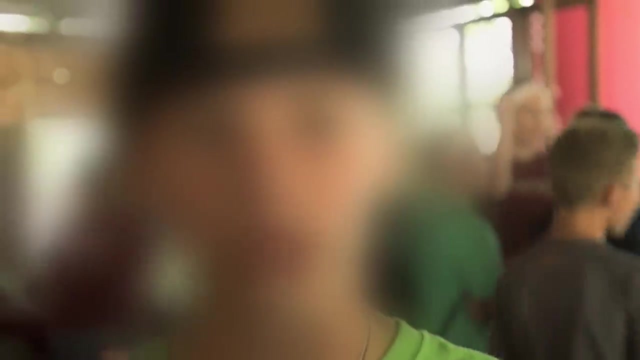 There you go. Their method seems to be working. We really want to like take this to each room of the hospital, if there's like anybody pregnant, and tell them that there's a baby in the stomach and they should be like getting rid of it. 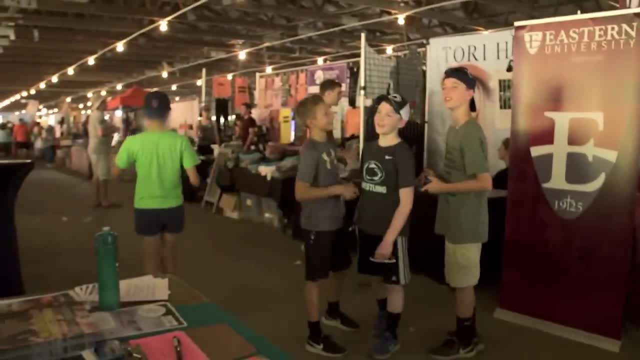 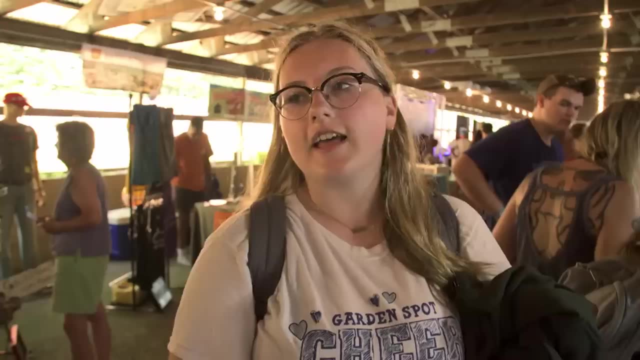 Amongst the other stands at the festival. the second major cause is abstinence. Yes, I am, I'm pregnant, I'm pregnant, I'm pregnant. There's different rings with Bibles, verses and stuff on them. God says that you shouldn't have sex before marriage. 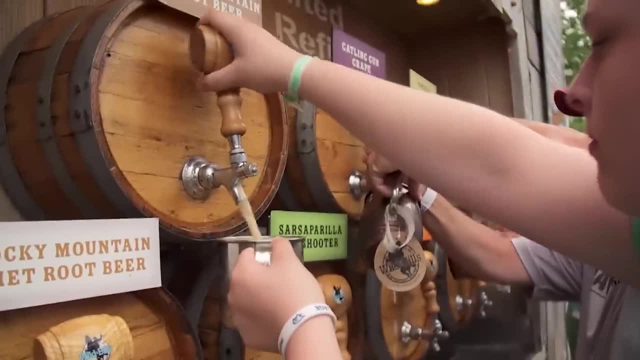 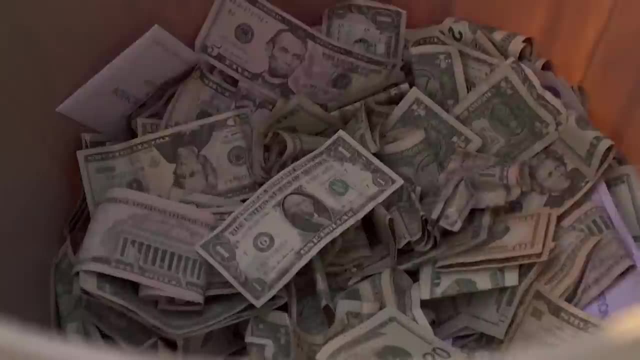 Even the beer is evangelist at Creation Festival. Do you sell beer? No, we don't. We sell root beer. What's root beer? It's an old-fashioned wild-billed soda. A normal ticket to the festival costs around $90,. 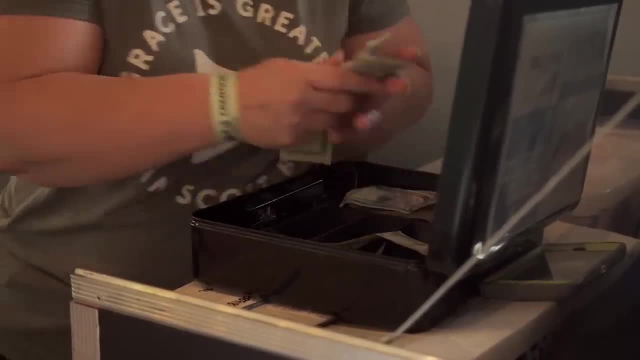 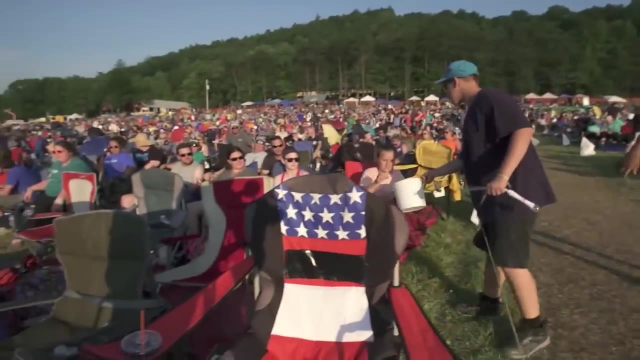 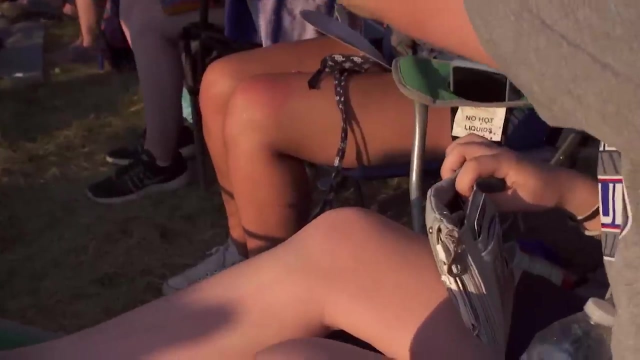 with VIP tickets reaching up to $800.. The festival also takes 10% on all sales made on site, With its 1,000 members of staff working voluntarily. On top of this, the festival holds a huge daily collection to increase its profits. 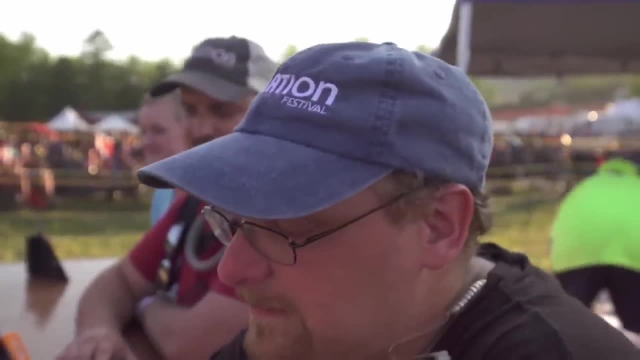 And if you're out of cash, they also take credit cards. How much did it cost you to use the campus costume? Uh, $85.. I don't want to know. I just asked God for a number and that's what he gave me. 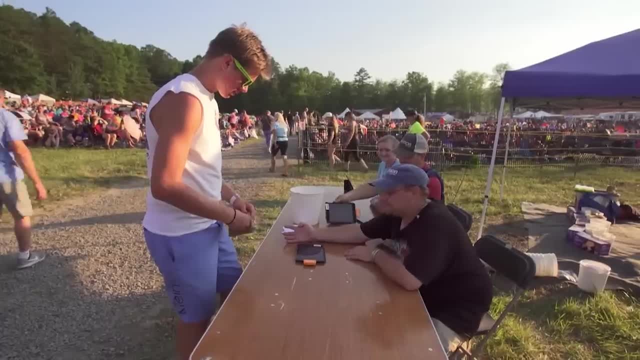 So that's what I'm giving him. A lot of people came. A lot of people opened up, Trees were cleared up. The business of the festival continues. It's been a long time since I've been here. It's been a long time. 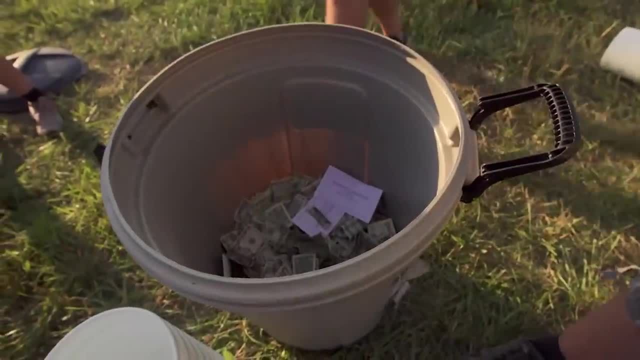 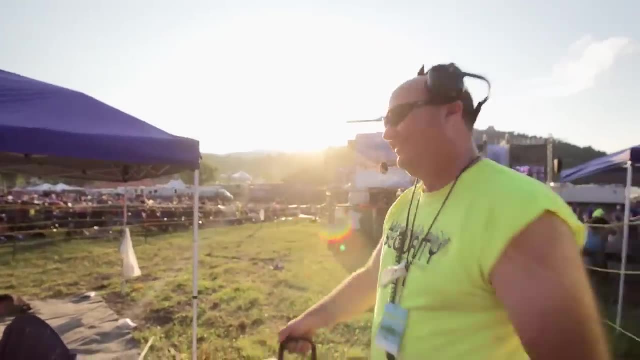 It's been a long time. It's been a long time. The business is clearly highly profitable, even though the organizers refuse to reveal their revenue. I knew they had what God planned for them to have. You know, in a day and a half or so. 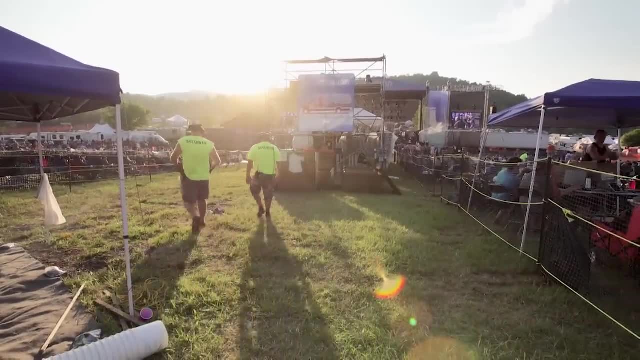 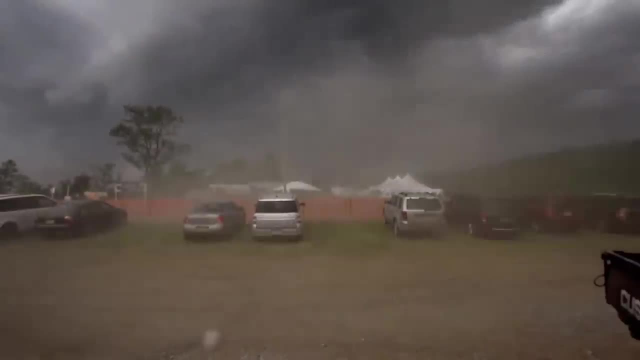 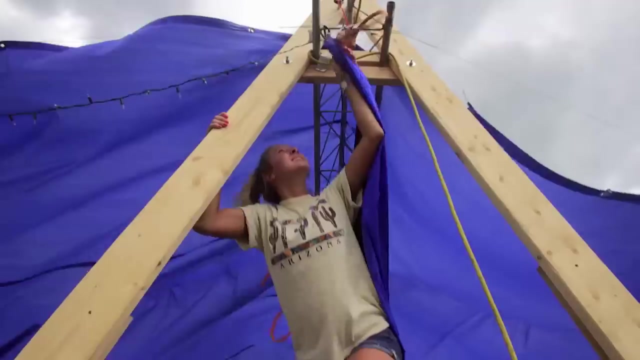 these good folks will be tearing all this stuff down. Just a few minutes after this collection, God's almighty hand seems to strike the festival site: Violent winds and torrential rains. The campsite is completely destroyed. Some participants aren't fans of the more capitalist side of this event. 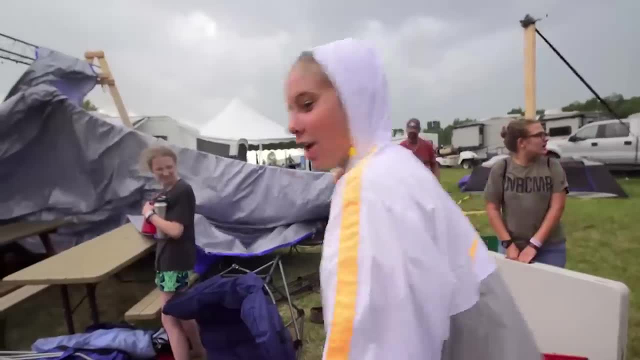 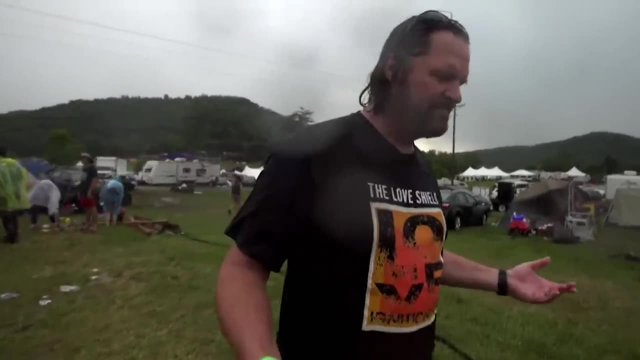 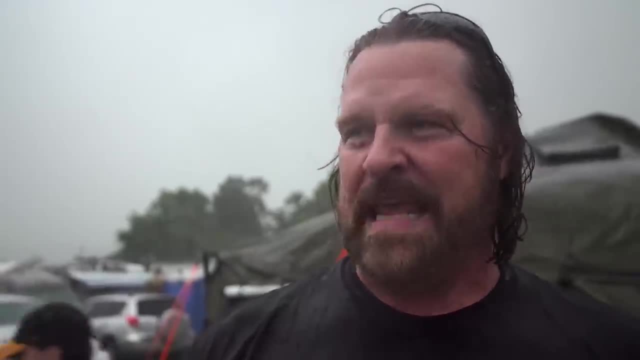 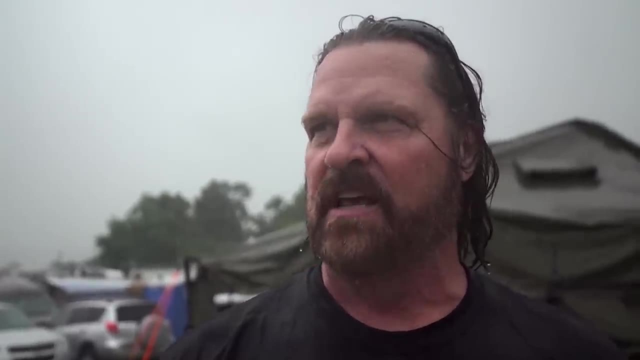 Backlash, Backlash, Backlash, Backlash. From what, If they don't do what He wants, which is not let it be lead by money or about money, about business, that He would take it away from them? Jesus? 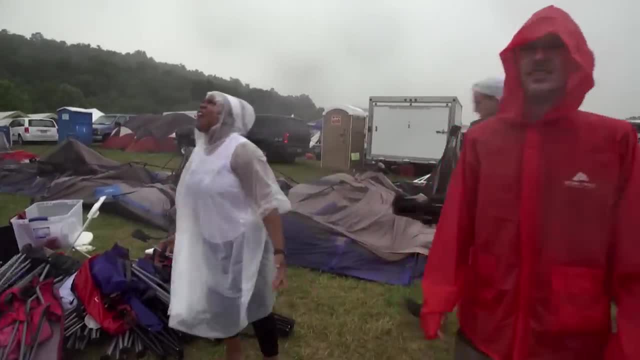 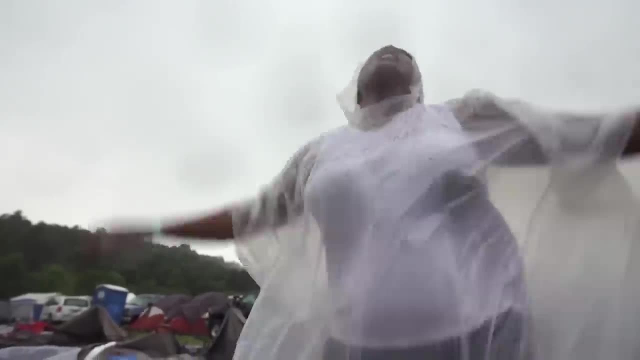 Father God, you are in control. Jesus, Even in the capital of capitalism, church collectors aren't always welcome. You are greater than their sons. You are in control, Lord God. You are in control, Lord God. So you make the http right now, Jesus. 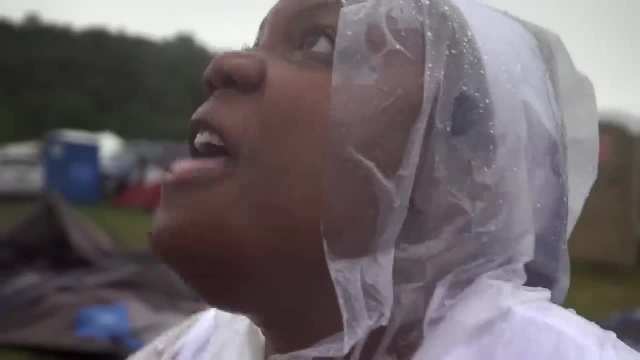 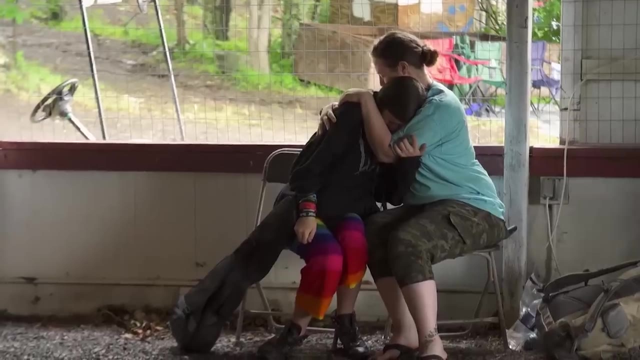 He will not have any victory here this weekend, this time, at this festival anymore. Father God, You are in control from here on out. You are clean and out. Father God, Young people come from all four corners of the states for the festival. 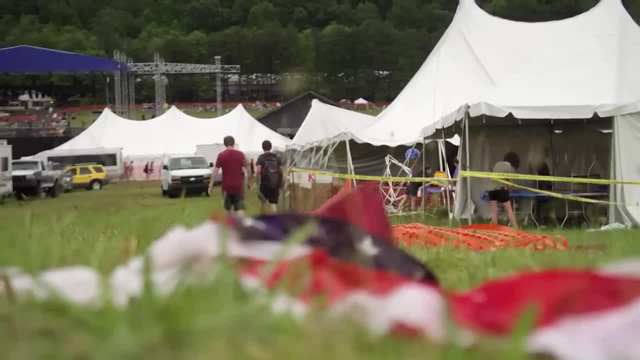 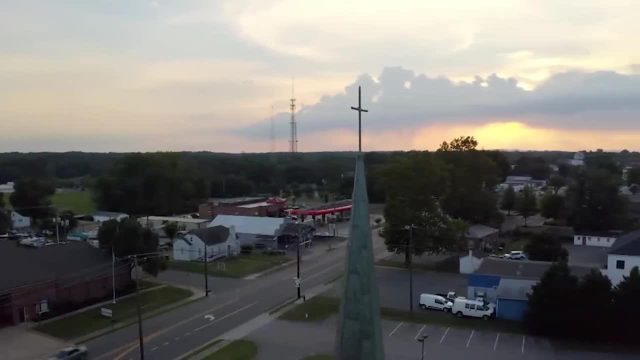 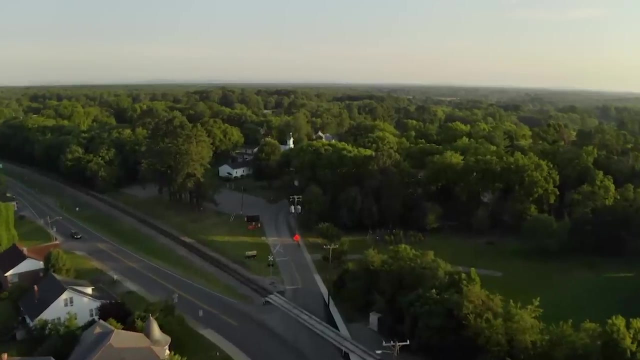 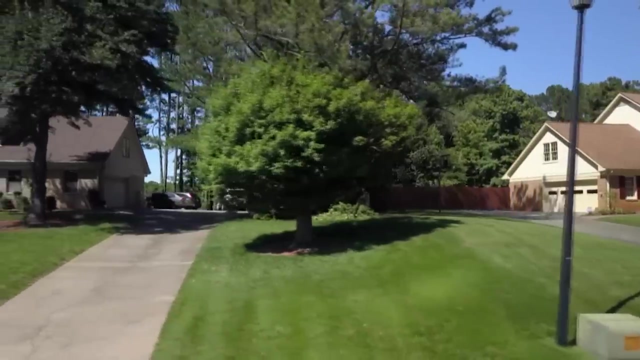 All of them have grown up in an extremely religious environment. To discover this 100% Christian lifestyle, we travel to the quaint town of Leesburg, Florida, an hour away from Orlando. It's 7 am here at the Copley household. 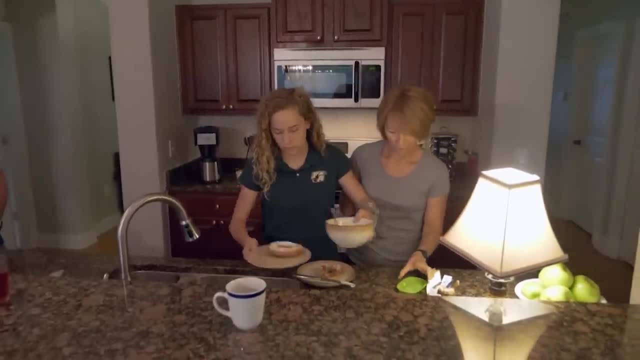 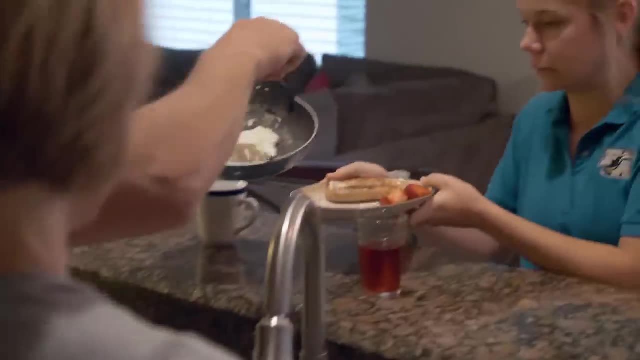 Here, you can sit right here. Lex, Lex, Yeah, Evangelists Keith, Angie and their daughters Layla and Lexi are having breakfast before heading to school. Don't get burned. Let me burn your fingers. Sorry, Glenn, I'm probably burned. 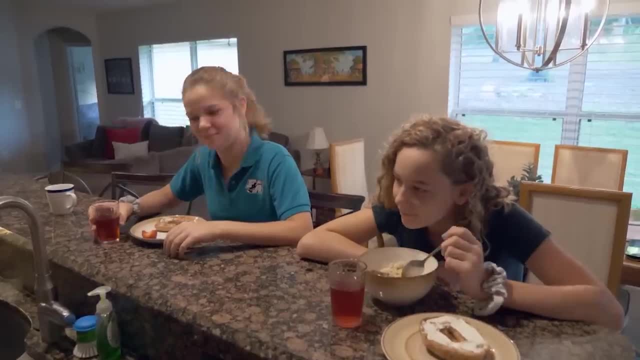 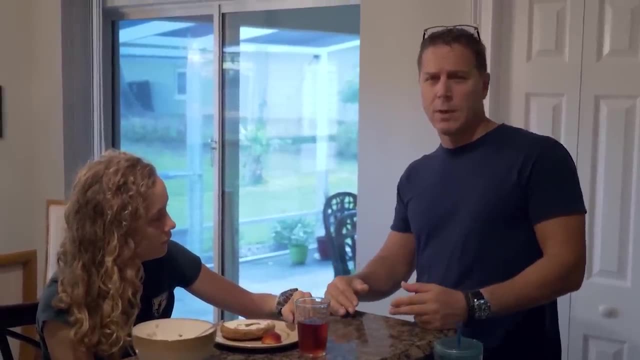 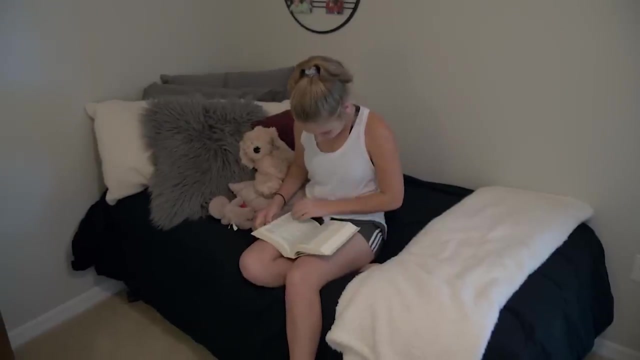 We've always taken the approach with educating our kids, to teach them to evaluate all that information through a biblical worldview or through a Christian worldview. Like thousands of teenagers across America, 15-year-old Layla has only known the Christian way of life. There isn't a single poster or magazine in her bedroom. 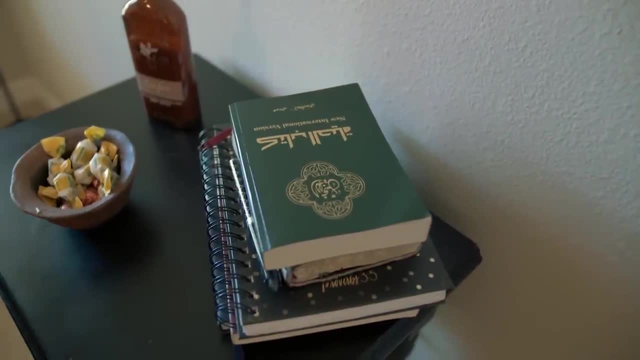 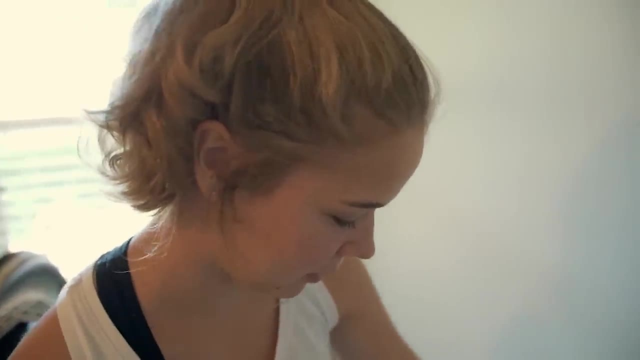 We could only find religious books stacked on her nightstand. This is the Arabic Bible, because I'm trying to learn Arabic, So yeah. And then this is my old Bible from when I was a kid. It's all torn apart. And then my new Bible is in here, and I keep it in here because I think it's so special. 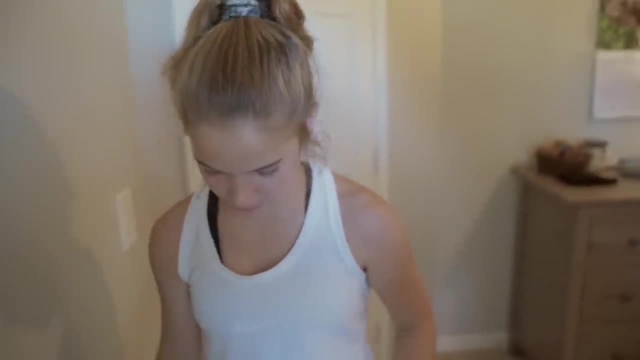 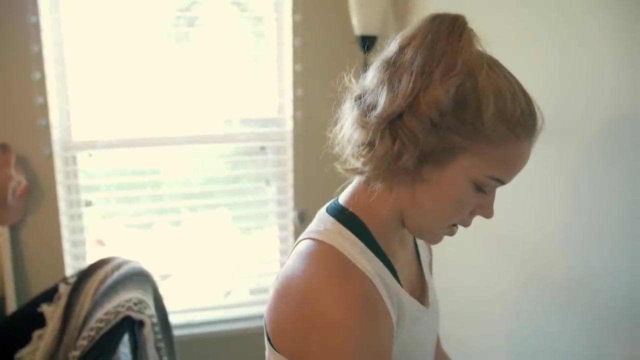 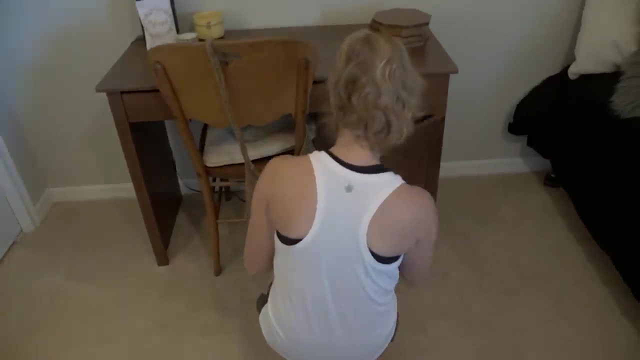 So I love it. This is a Christian book by a preacher named Francis Chan. Do you have any non-Christian books? Um, let's see, Even at the back of her closet, What's down here? I don't think so. 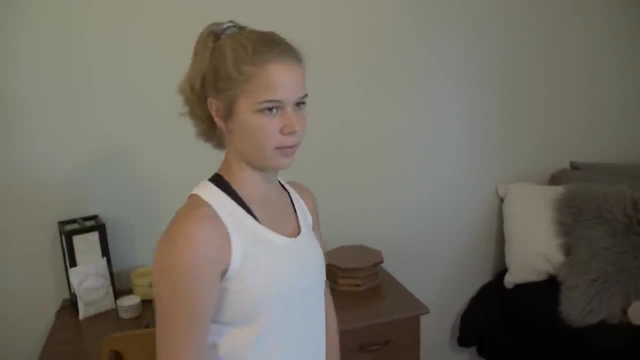 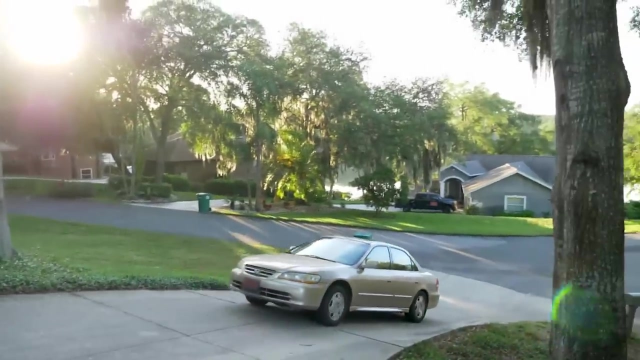 She can't find a single one, But we have them in our around. Finally, Layla finds one non-religious novel. She heads off with her sister and dad on the school run. That's all you got. Oh no. 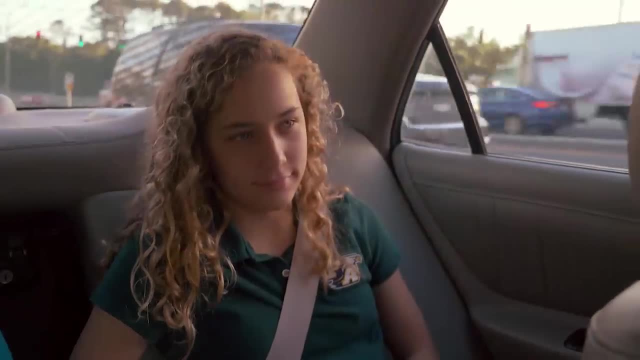 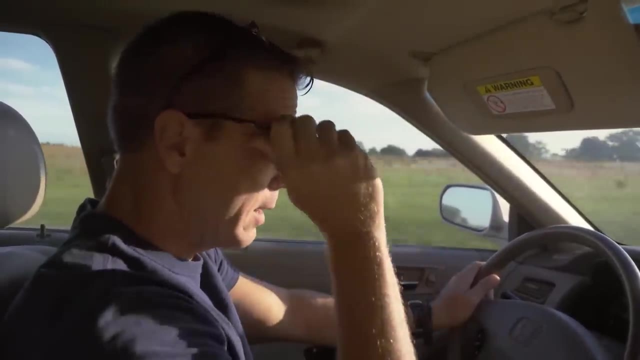 And, of course, religion. It stays with them at all times, even on the radio. We actually have Christian radio on just about anywhere in the country. you can find a Christian radio station. The Copleys cross the town center on their way to school. 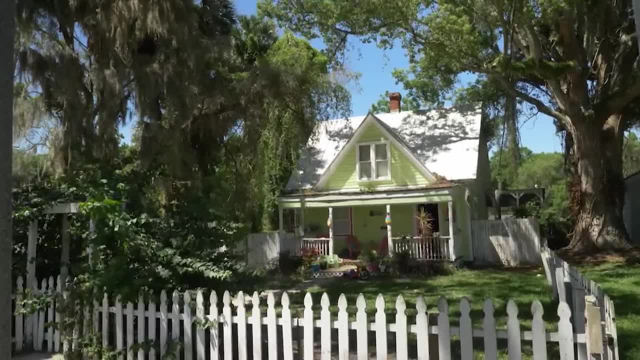 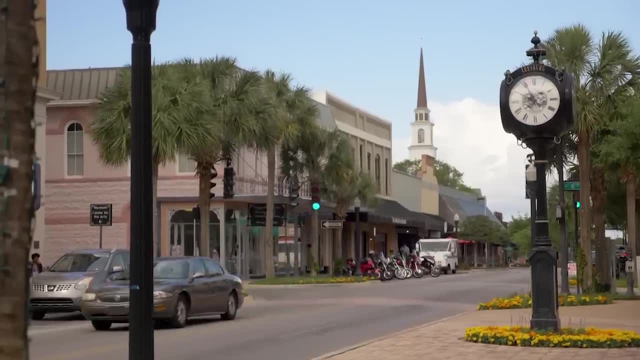 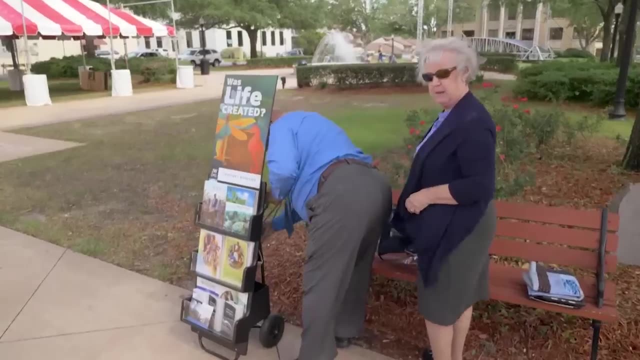 Leesburg boasts an almost entirely Christian population. There are 151 churches for only 22,000 residents. Hardly surprising, given that this is the case in most rural American towns. It's impossible to cross The main street without being stopped by Christian groups. 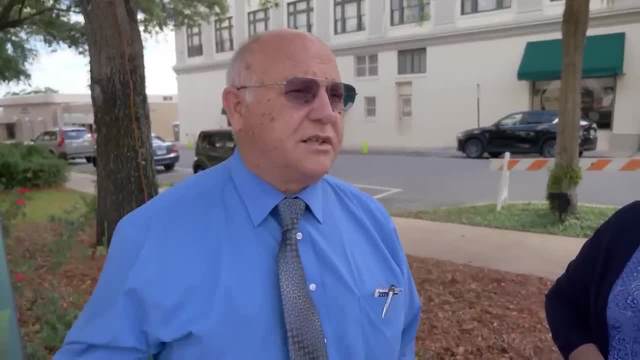 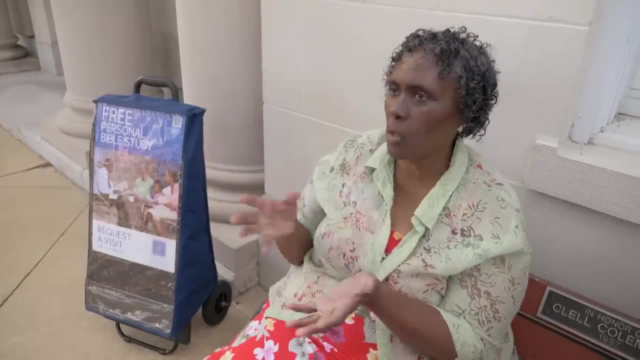 One of the commandments that Jesus left with us was that we needed to preach a good news. All of them are trying to increase the number of worshipers at their church. As the people go by and they see something that they want, then we, you know, talk and introduce the message that we have. 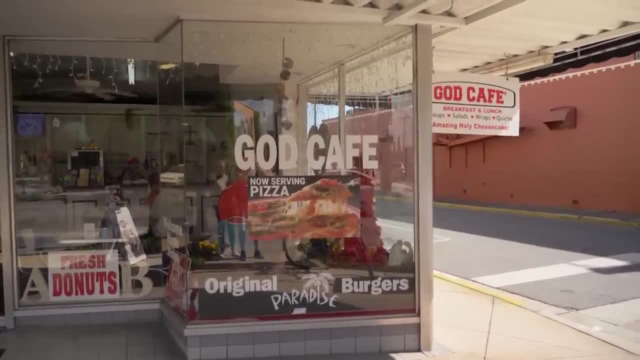 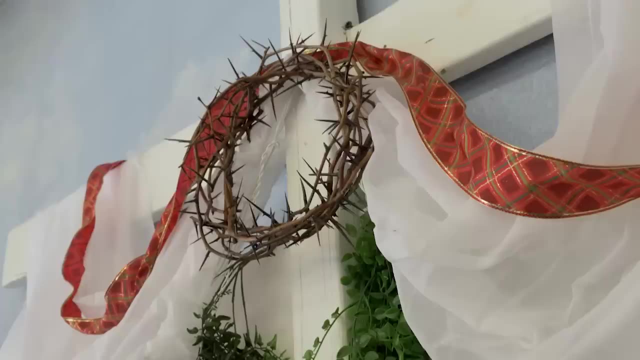 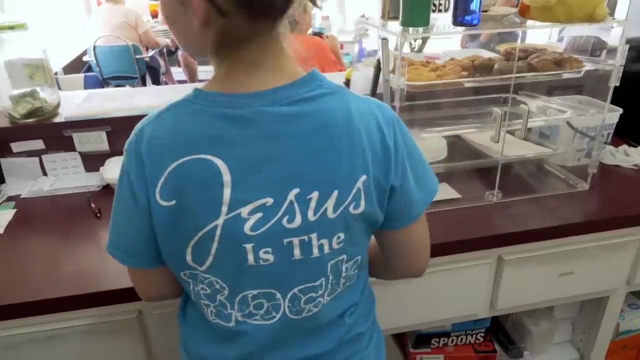 Further down Main Street, some people are becoming even more inventive when spreading God's Word, like at the God Cafe: Giant crucifixes, posters of Jesus, even the waiters' t-shirts. This is a 100% divine cafe, So I've been given a paycheck. 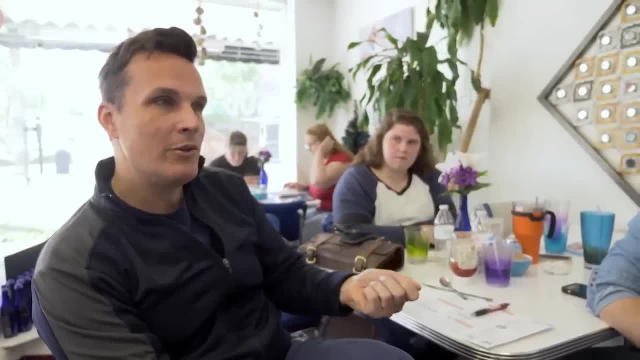 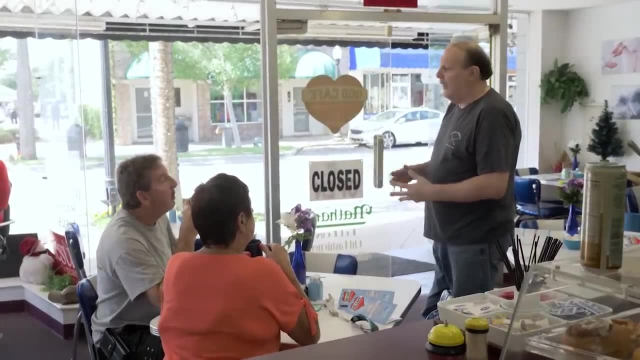 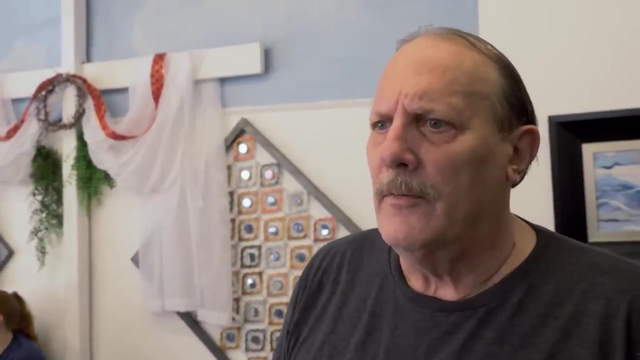 I've been given this money. Why not spend it in a place that you know God is present, versus a Starbucks? Gary opened this restaurant 12 years ago. Basically, what God wants is to be seen, But you know the enemy's out there going to and fro, so we need Satan. 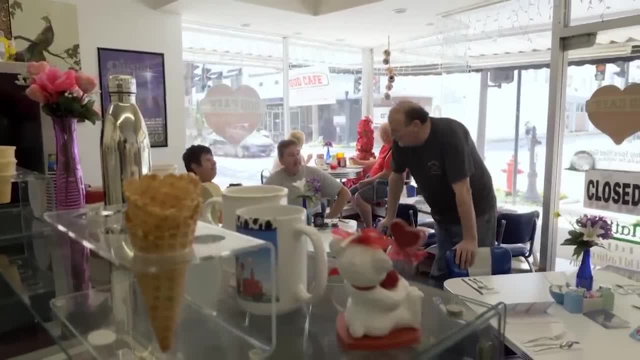 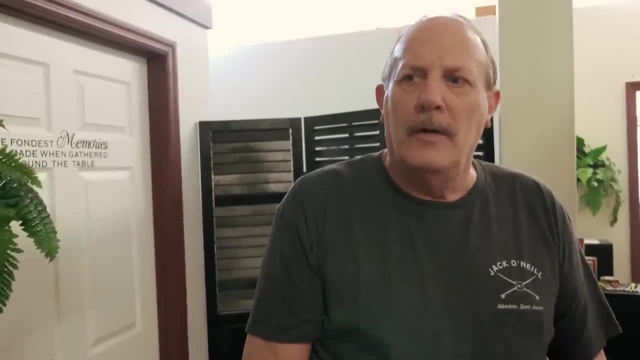 Donald Trump earned 60% of his votes here in Leesburg, with one of them being Gary's. God is using Donald Trump to change America and get things right. I believe he believes in God and I believe he believes in Jesus. 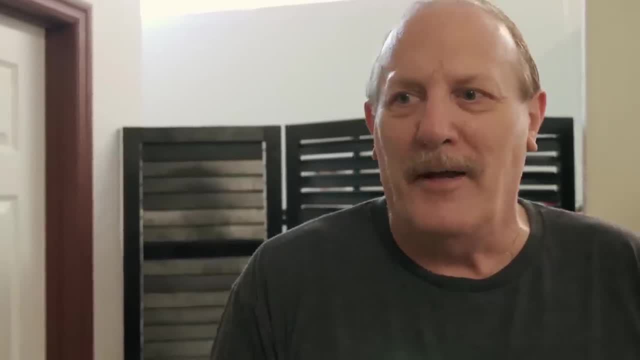 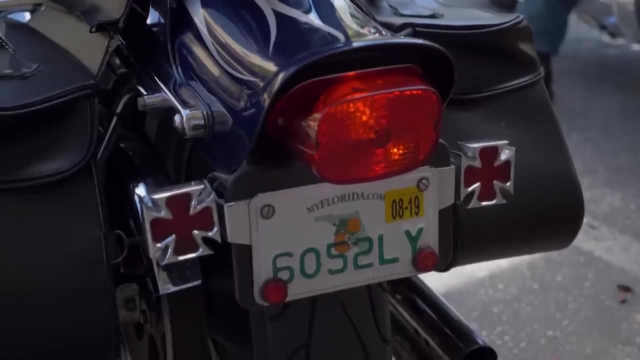 I mean they have Bible study in the White House. so you know that's just starting in the right direction. We find some Christian bikers hanging out outside the God Cafe. God bless America. Far from the traditional bad boy image. 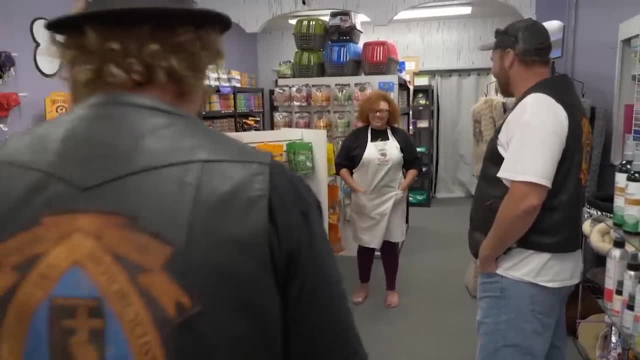 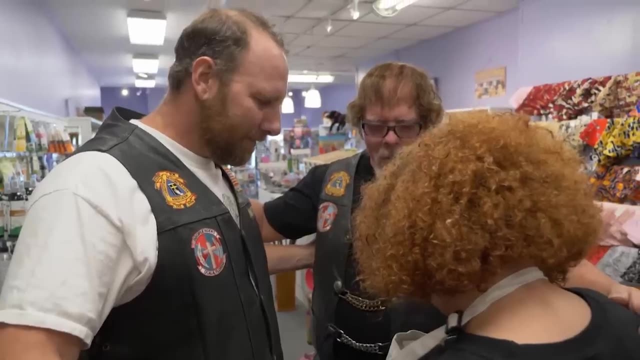 these bikers are here to bless all local businesses. The sales lady accepts enthusiastically: Lord Jesus, we're here with Caitlin. You know that, Lord. We're just asking for safety within her store. Lord, that there's no problems. 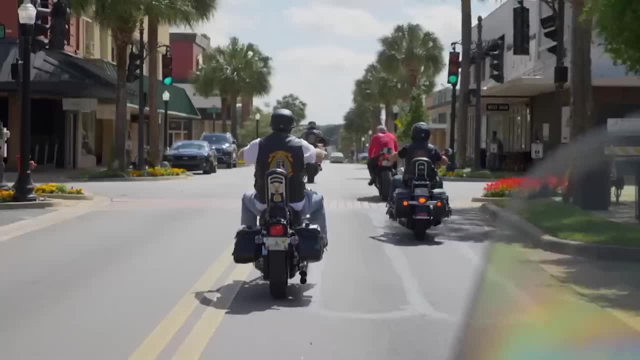 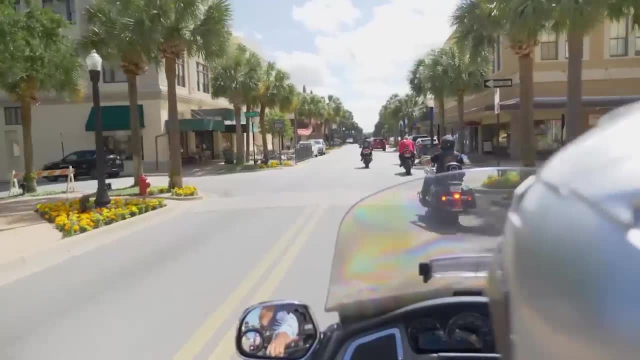 No one comes in and tries to rip her off. Lord, and walk off with a lot of her Jesus' bikers, bless the town and its inhabitants and even, on occasion, convert the non-believers. We catch up with Lila and Lexi. 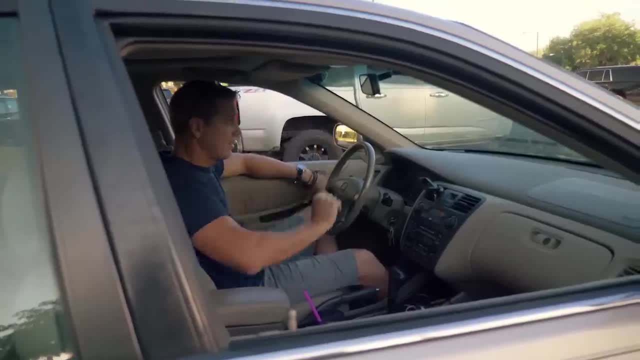 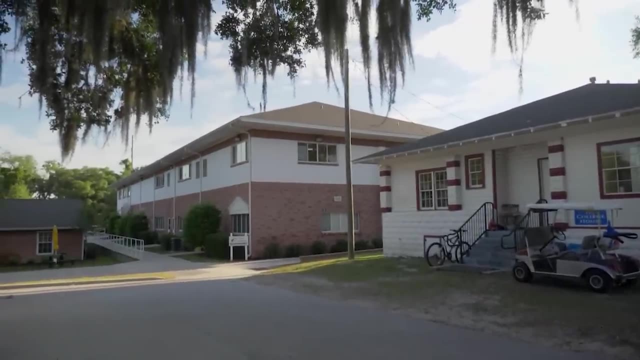 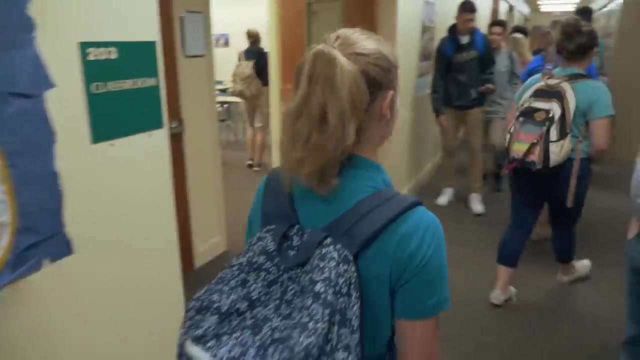 Hi Dad, love you, Have a good day, Drive safe. Love you guys. They've just arrived at school. This private school belongs to one of the town's largest churches, First Baptist. The oldest sister, Lila, begins her day with math class. 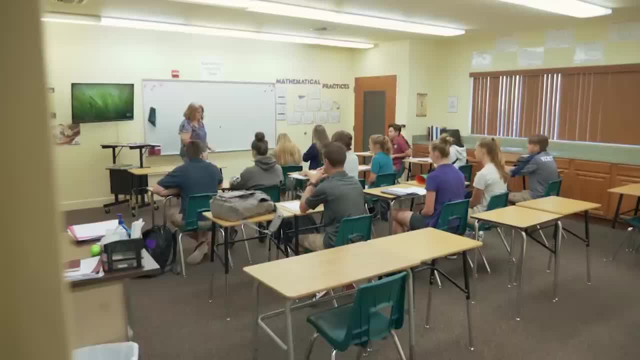 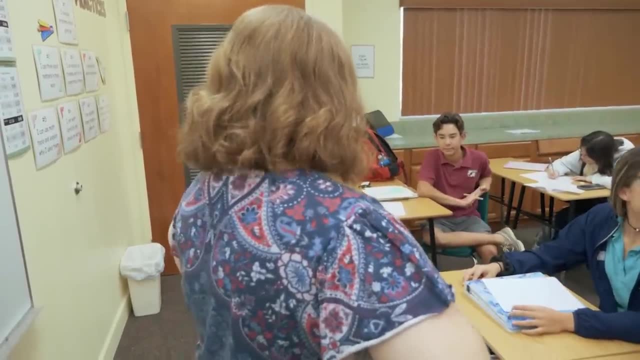 However, the teacher doesn't start class with algebra or geometry. Any prayer requests? today I'll stop rolling. I have a long drive, but I feel like it's rolling A long drive. Yeah, Okay, Yes, kid, Just for this weekend. in general, 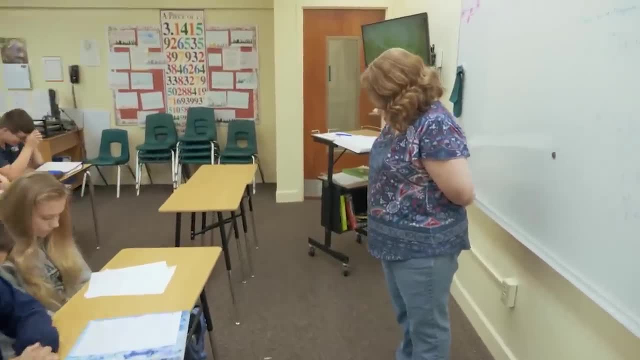 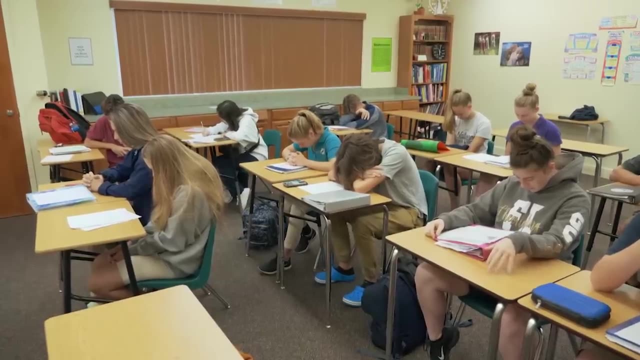 Okay, now we're going to pray. Bye, we're going to pray now. Dear Heavenly Father, thank you for this day. I pray for- Praying for a good weekend, a win at a basketball match, Here- all aspects of daily life are covered by God. 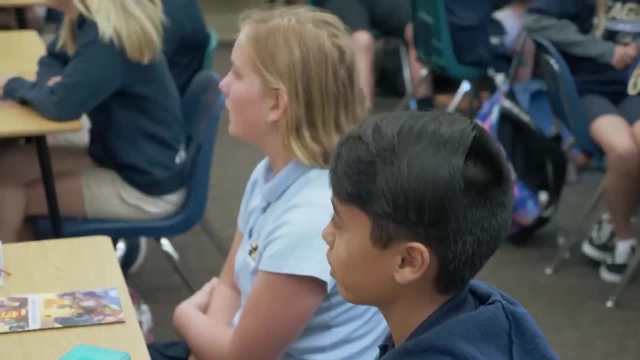 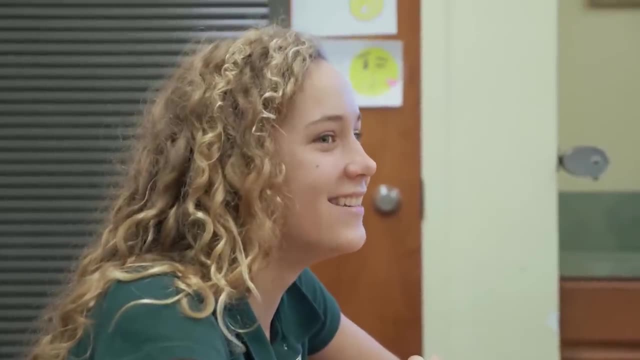 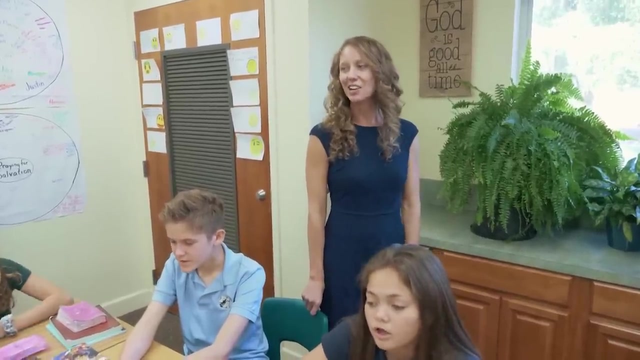 Amen. In the neighboring classroom, When the day of evil comes, Students are learning the Bible by heart. They'll do this for one hour every day up until they're seniors. Take the helmet of salvation. Mindy is teaching her students that if they don't keep their faith, 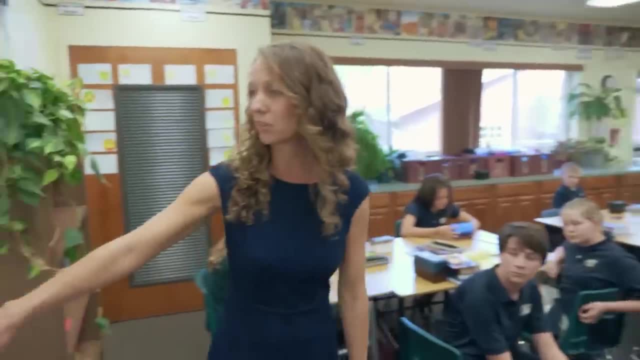 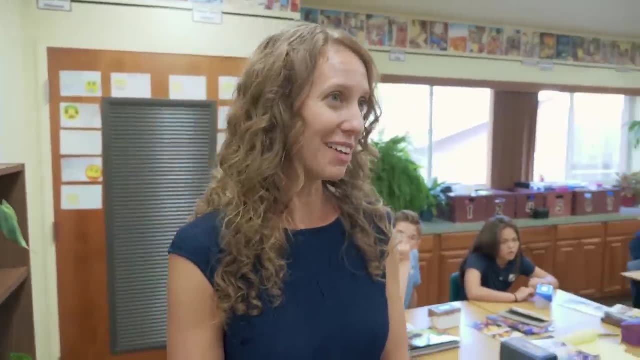 they'll be damned to hell. We actually pray for people who are not believers all the time: Aunts, uncles, neighbors that we love and we know, and we want to pray for them. We want to see them in heaven, Spending the afterlife in hell. 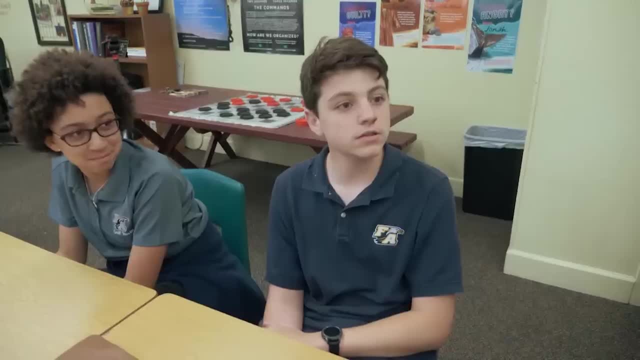 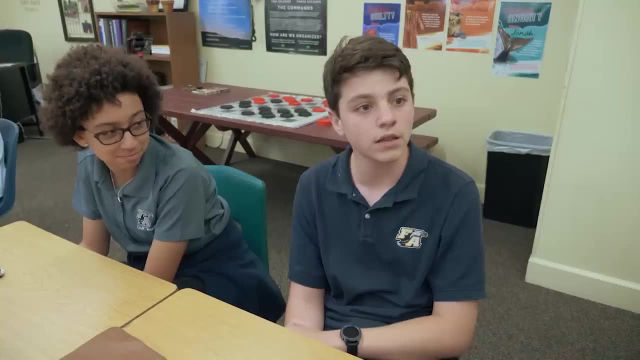 is a real fear for these kids. I feel like hell is something that you should be afraid of, And it's kind of like a motivation to strive to be like more godly and Christ-like so that you don't go there. It's something meant to scare you. 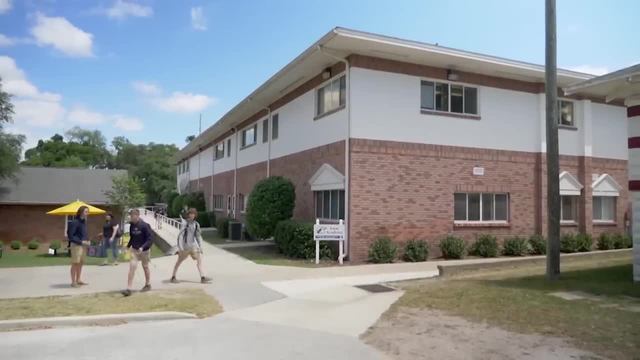 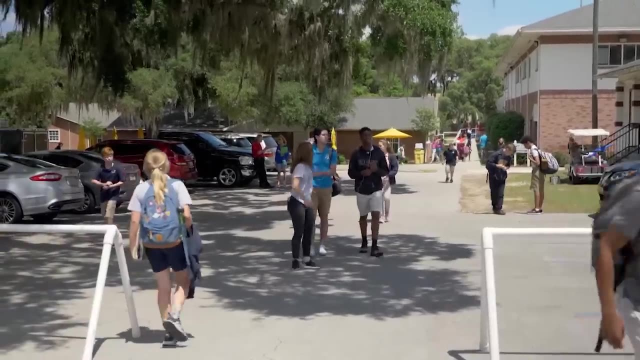 Again at recess. it's the Bible that dictates how these kids behave, Especially when it comes to matters of the heart. It's a taboo topic for this group. They're barely able to open up about it. All right, all right, all right. 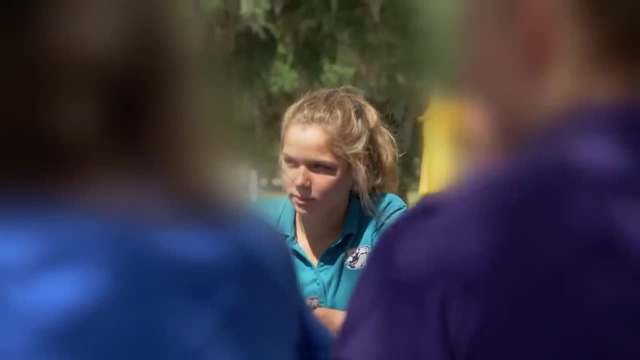 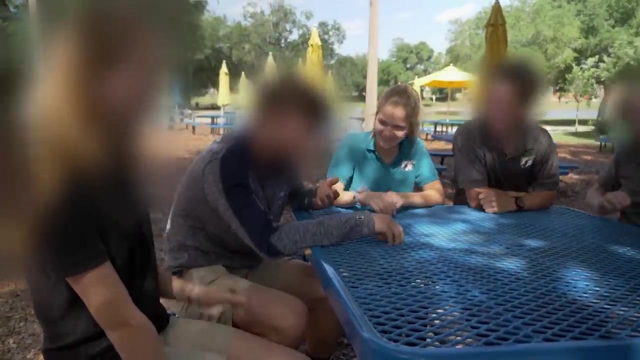 Sammy, I'm probably the most fallen. He's successful. Yeah, Good job, Sammy. This one is not successful. Okay, I am dating. You don't have to bring this up. These teenagers are between 15 and 18 years old. Christian goal is to be a Christian. He was a Christian since he was a teenager. He was a Christian since he was a teenager. He was a Christian since he was a Christian is to try and stay away from sexual relations till marriage, and I would define those as like any. 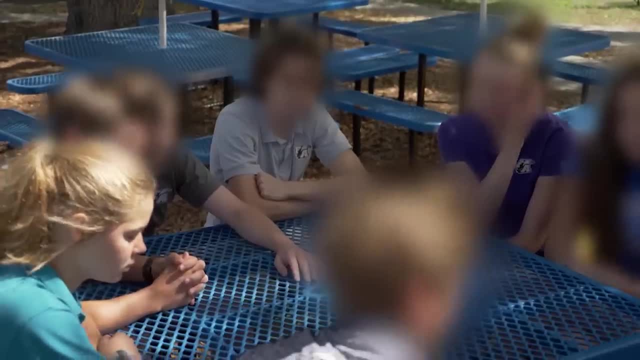 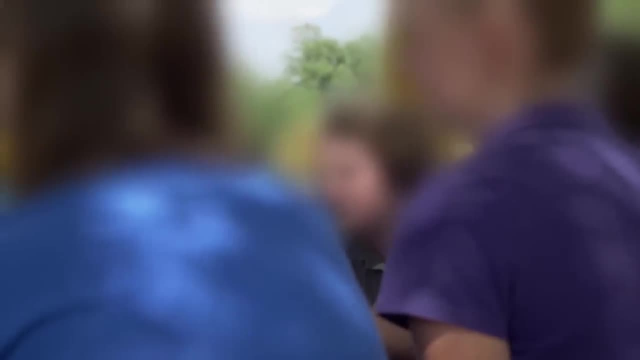 Sleeping together? I can't think of a word. Sleeping together Probably include like oral sex in that too. Yeah, And then probably any sort of Social media. I can't think of the exact word Roping. No, I'm not saying that. 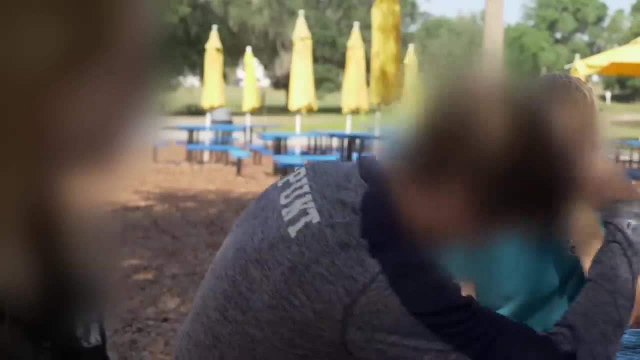 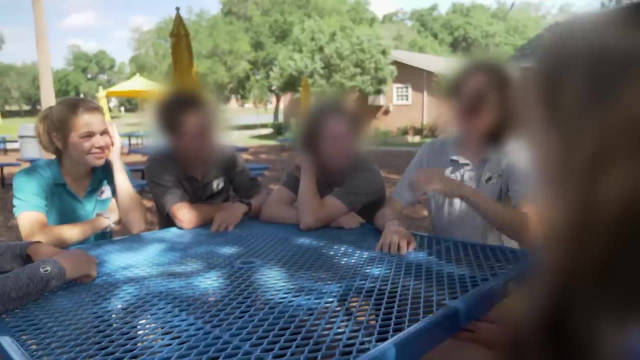 I'm saying like What's the word Via social media? Is it penetration that you're looking for? Yes, like any sort of penetration, Sometimes it's easier if you have like a friend or a parent go with you on your date. 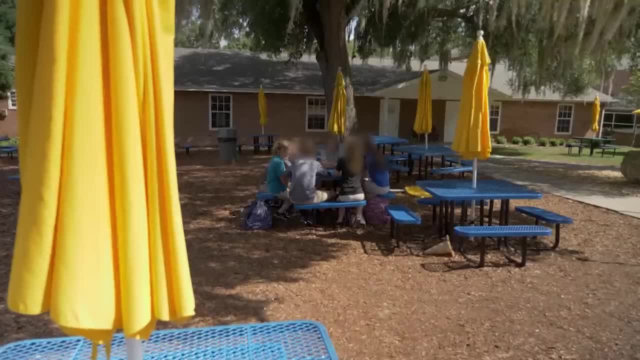 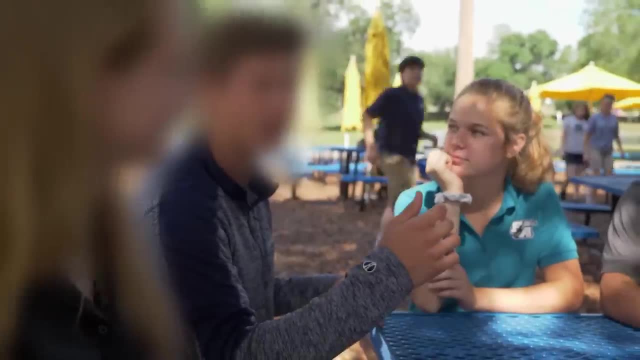 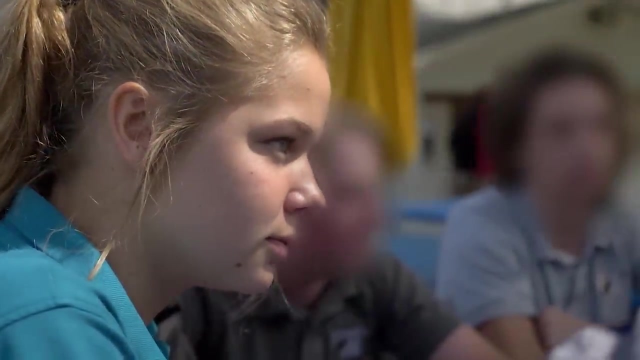 so you can avoid like the temptation of sex or like Abstinence isn't the only restriction imposed on these teens. I've seen like a lot of like our friends go through like times where they start doing like more secular things. 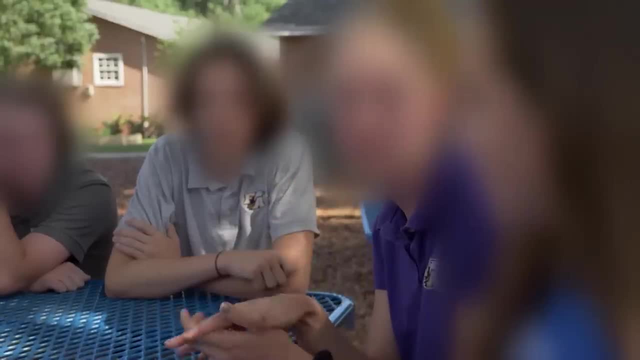 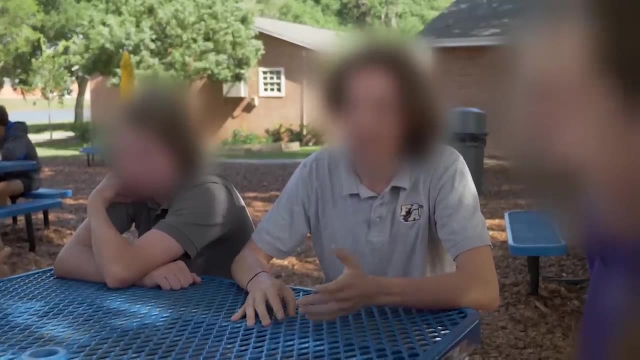 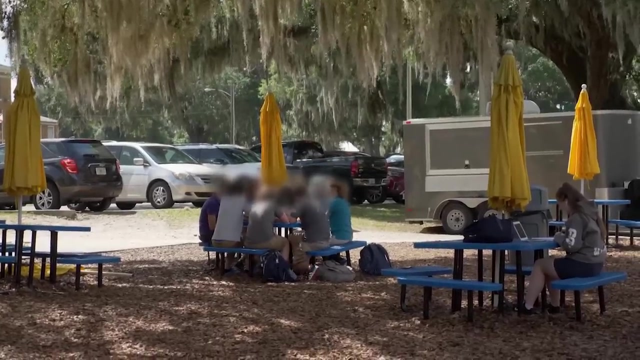 What's a more Secular thing? Secular things can be as simple as gossiping, Talking bad about someone else, A lot of drinking, smoking, drugs, sex. All that kind of stuff is against what the Bible would say. To instill these Christian values into their kids. 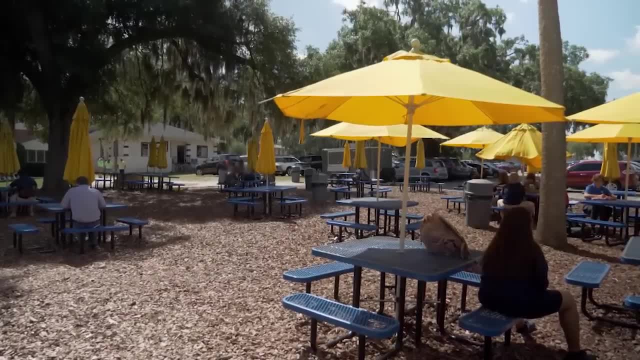 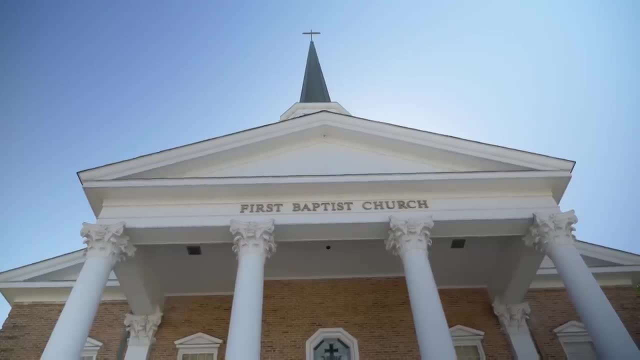 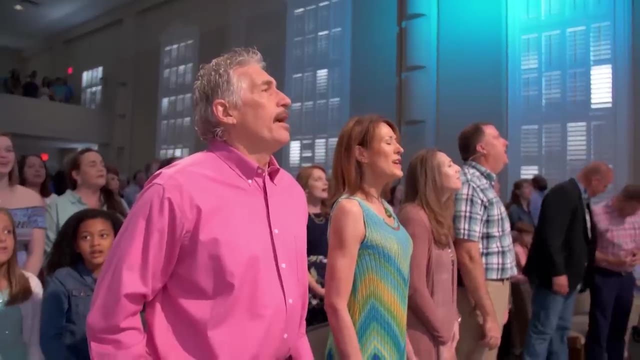 families spend between $5,000 and $12,000 a year, depending on which classes they are enrolled in. Religious organizations like First Baptist and its school are exempt from paying taxes here in the United States. This particular church is rich and powerful. 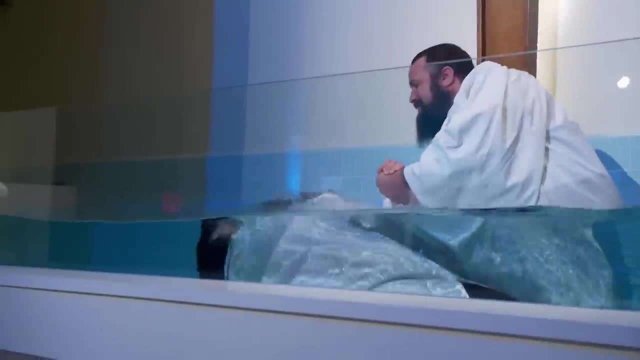 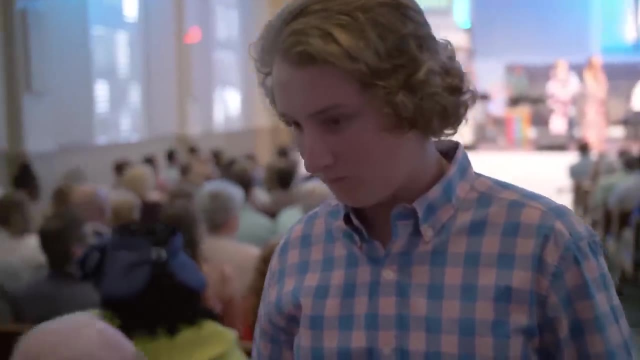 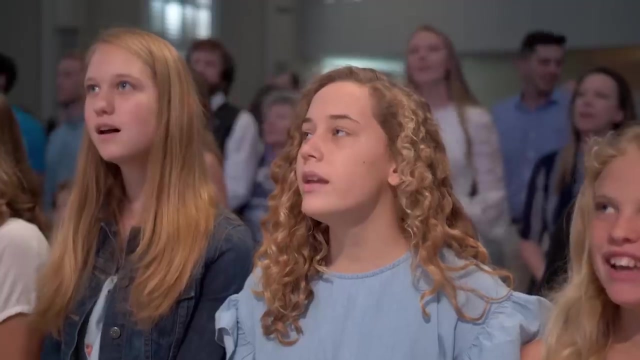 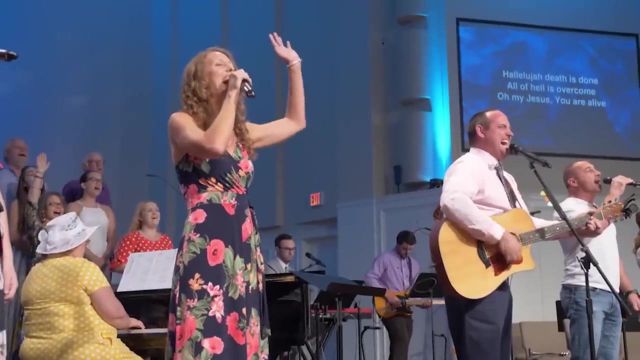 The community boasts 2,500 members and is still recruiting, with new believers continuously being baptized. During the celebration, First Academy students walk around for the collection крепedorg. The Copley family are also present, as is one of the high school's teachers, Mandy. 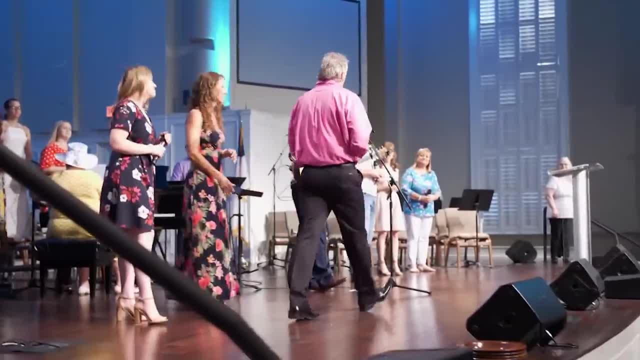 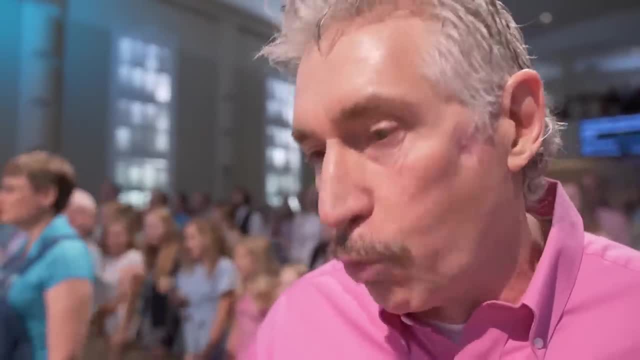 School, social life, family and even financial matters all revolve around the church Head. Pastor Art has a lot of influence in the community. ¶ The people give 10% of their revenues ¶ to the Lord's work here. ¶. ¶ The、 ¶ ¶ Yes ¶. 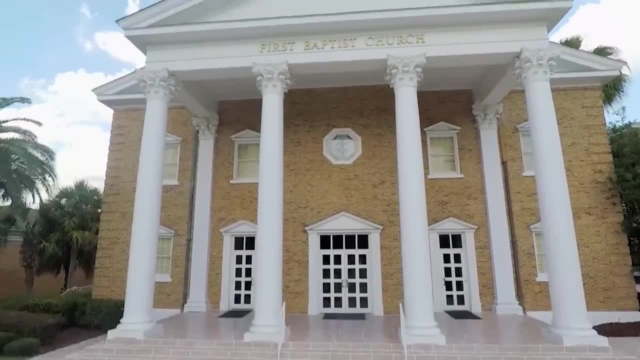 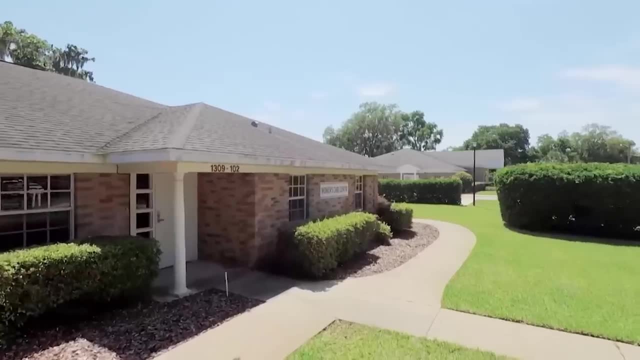 ¶ I'm so, ¶ ¶ For sure, ¶ ¶ For sure ¶ ¶ Yes, ¶ ¶ For sure ¶. ¶ The leader has ¶ ¶ The leader has to ¶ Lead the way ¶. thanks to these donations, the church has its own hospital, a clinic for pregnant women, a refuge. 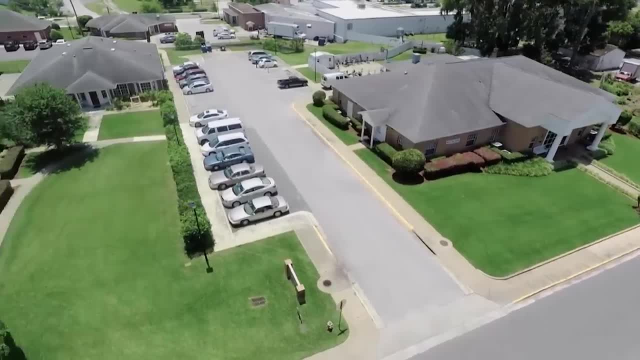 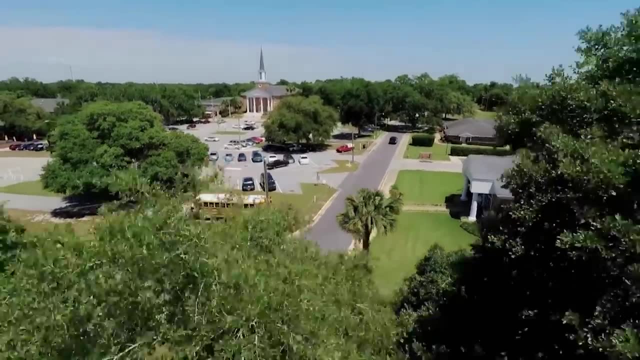 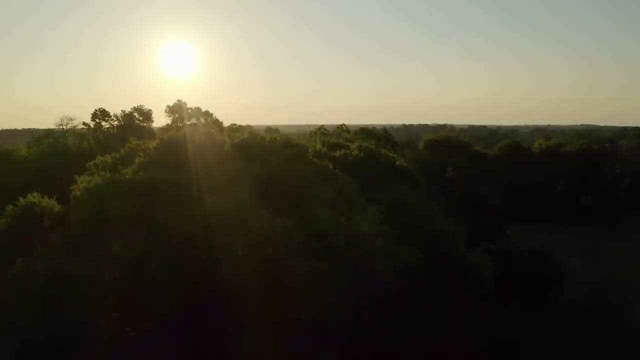 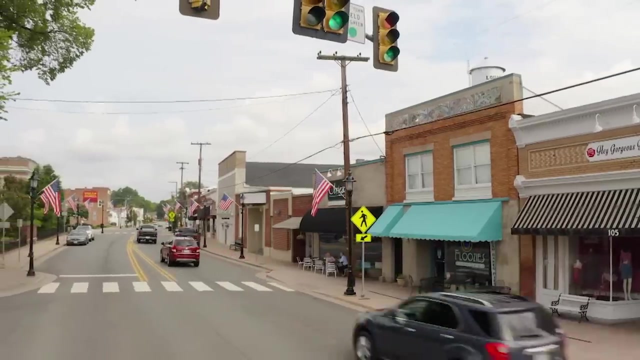 shelter for men and for women in difficulty, a training center for evangelization and even its own shop- every possible facility to ensure the members of the community stick with their own people. in certain towns, faith has even made its way into public institutions. it's sunday morning here in louisa, a town in virginia. 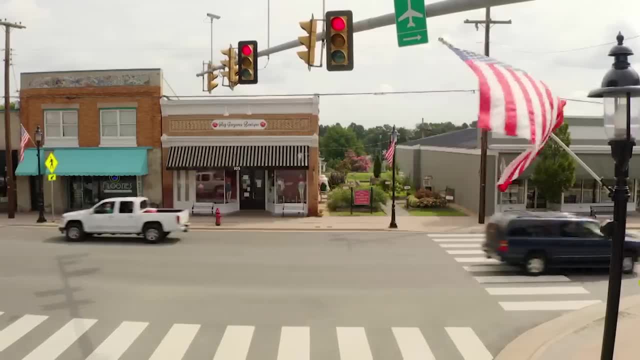 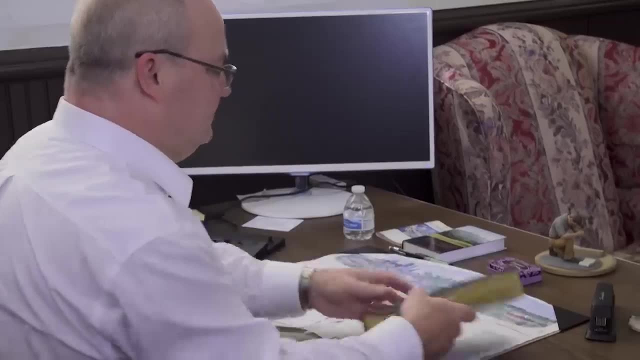 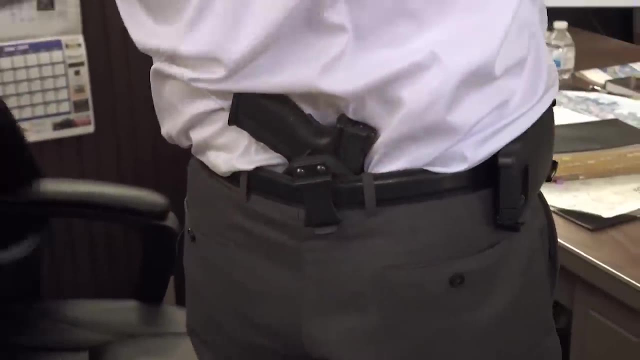 pastor of the main church, mark o'connor, is preparing his sermon when getting ready for sunday service. it's his pistol. he grabs and starts to shoot instead of his chasuble. Well, I'm carrying a gun because part of a pastor's slash chaplain's job is the protection of the flock. 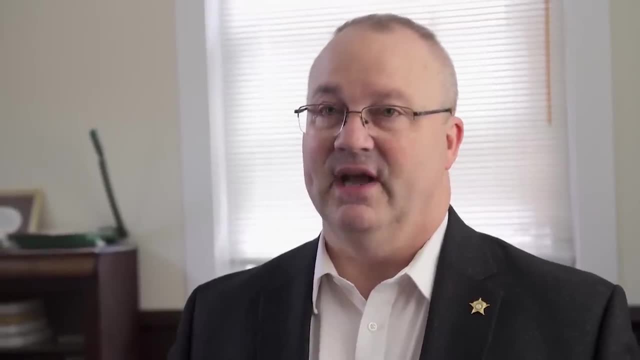 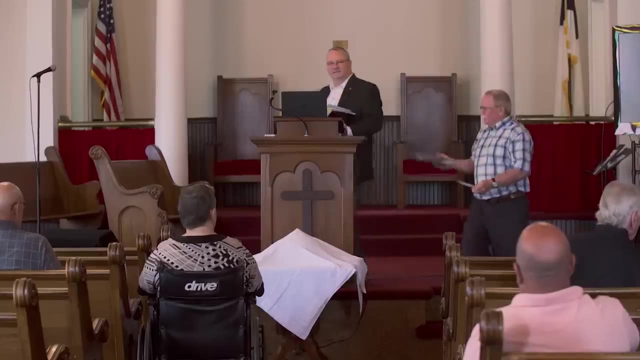 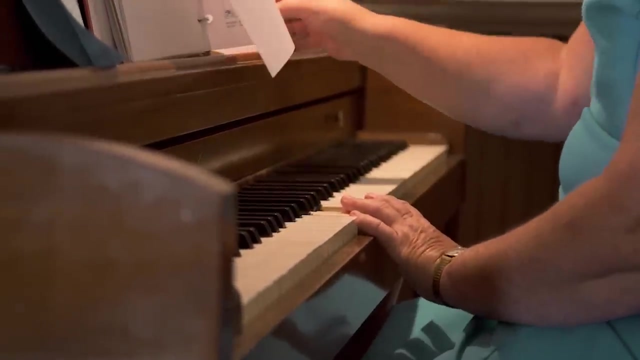 spiritual and physical. You know it's part of the job and I take it pretty seriously. so Morning everybody. This armed pastor holds some very conservative and controversial views. This says homosexuality is a sin. Homosexuality is a sin, just like lying. 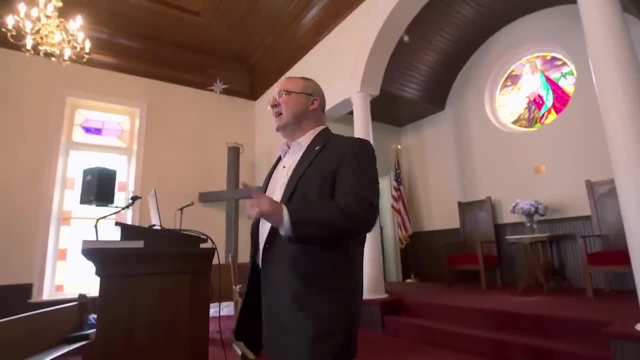 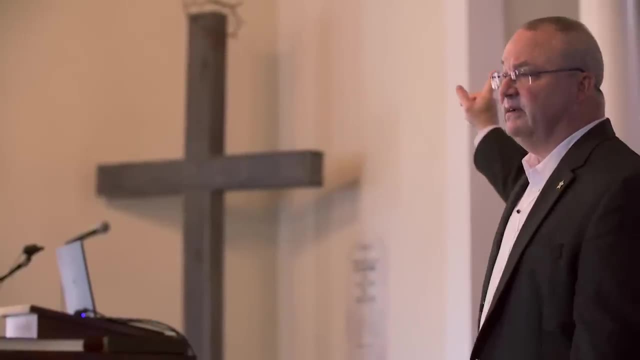 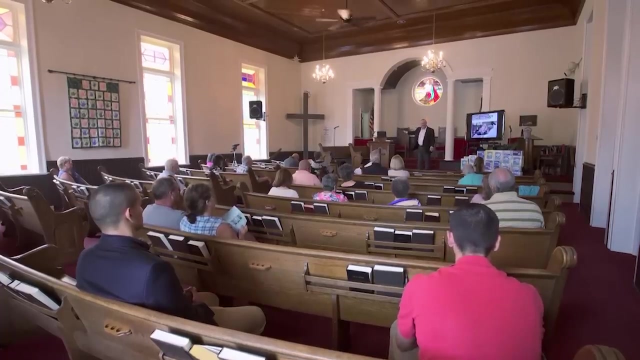 just like stealing Sex name a sin. they're all equal in the eyes of God. Mark believes there's only one destination for all sinners: If you keep down the path you're on, you're going to go to hell forever. 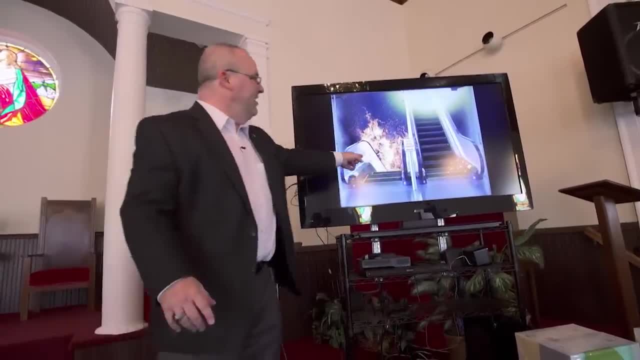 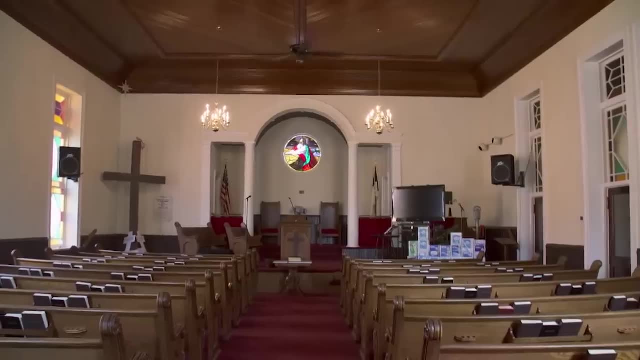 So the choice is simple: right, Who wants to go down there and start cooking? His mission to moralize the population doesn't stop at the altar After the service. Mark poses his Bible in the house of God and closes his church before heading out. 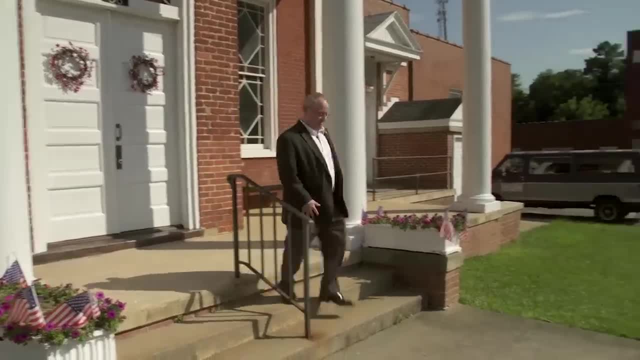 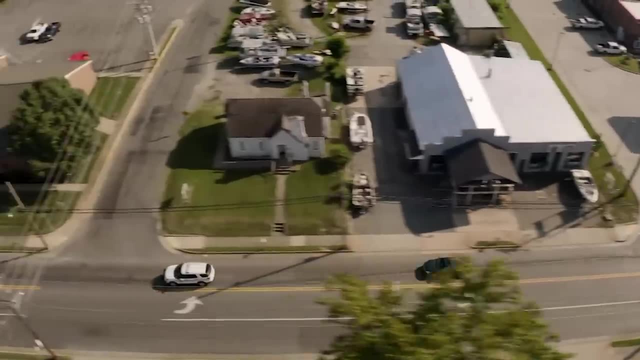 on an unusual mission, riding along with one of the sheriff's patrolmen. Hey, Daniel, How you doing, man? Good to see you. Yes, indeed, Let's go Side by side with law enforcement. he preaches to those who have strayed. 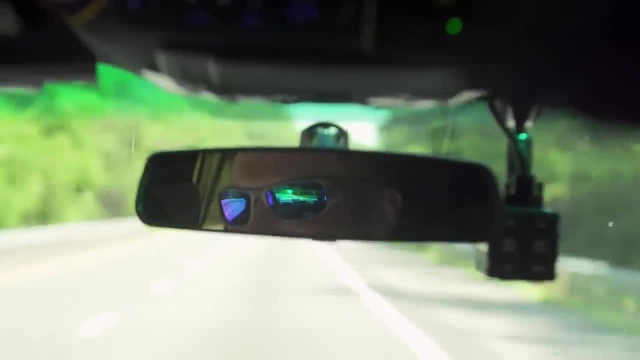 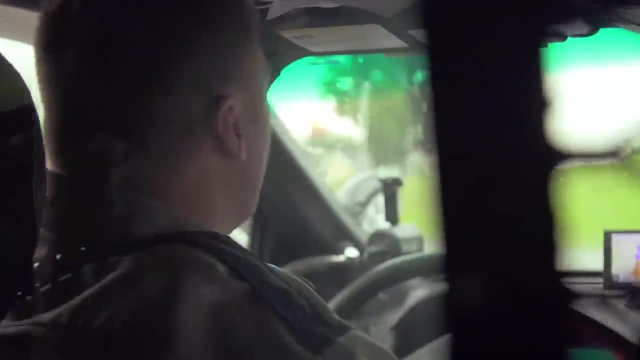 from the righteous path. The pastor is on patrol with Daniel, who is very religious- Anything in abundance is a sin- but They even discuss their own visions of heaven, Like when we get to heaven, that means I'm going to be walking down the streets of heaven. 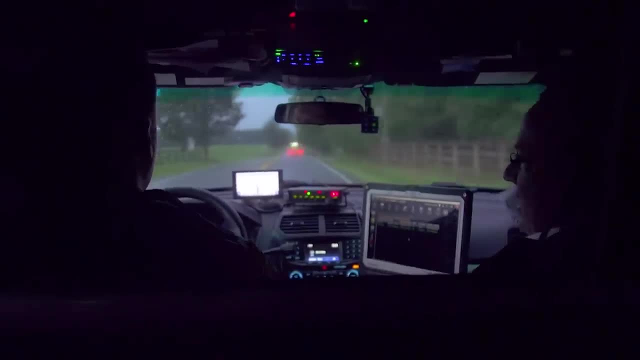 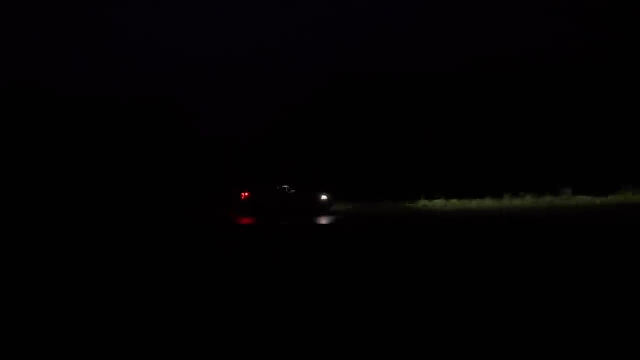 I'm going to see like Noah, as in Noah in the ark. I'm going to say: Noah, what's up, man? He's going to say: hey, Mark, how you doing As night falls, Daniel is on high alert. 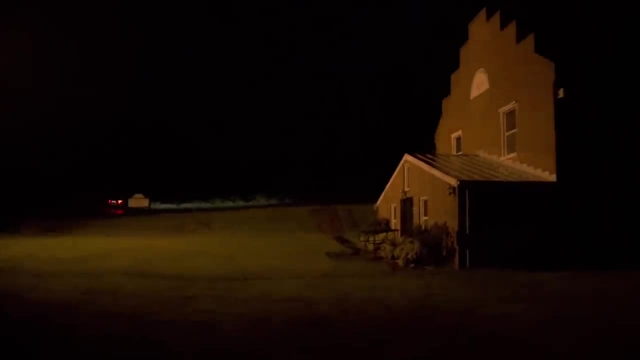 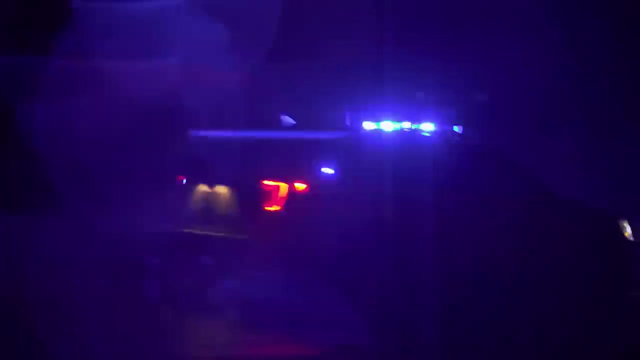 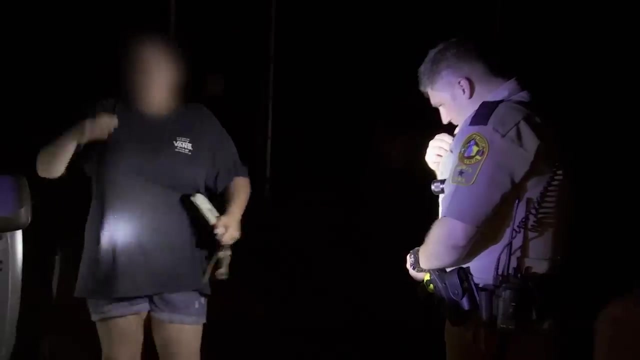 It's the holidays here in the States and a lot of young people are taking advantage to head out and enjoy themselves. As expected, Daniel finds himself flagging down a speeding car- Courtney, the driver is only 20 years old and is really stressed. 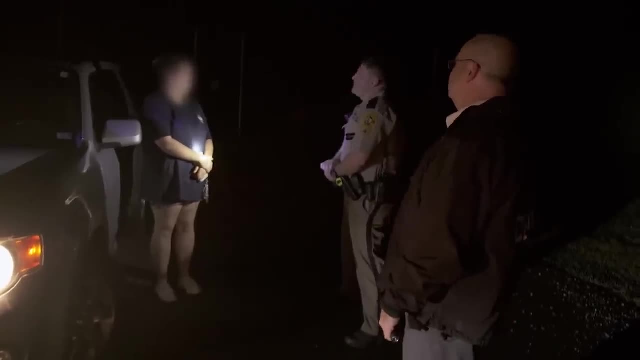 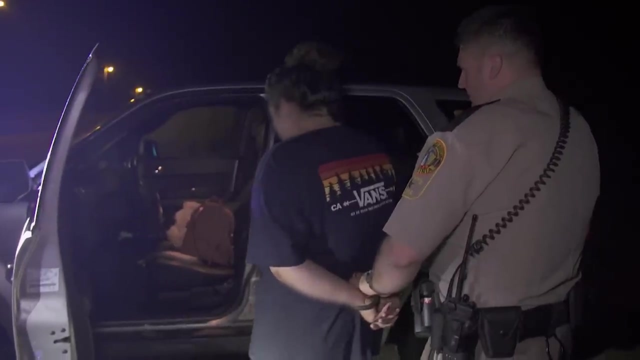 You're really nervous, but I'll also smell marijuana in your car. See what's up with that. Daniel immediately handcuffs the young woman who is now panicking. Am I going to jail? When we approached the car, there was a very strong smell of marijuana. 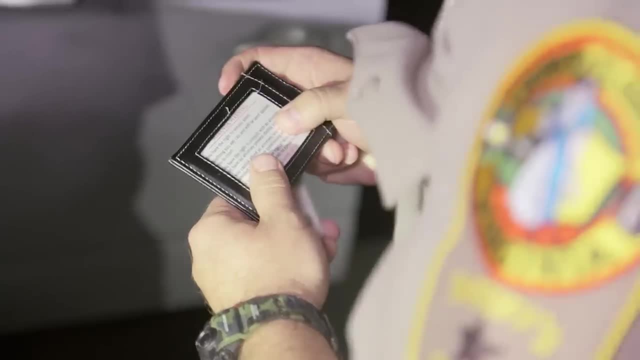 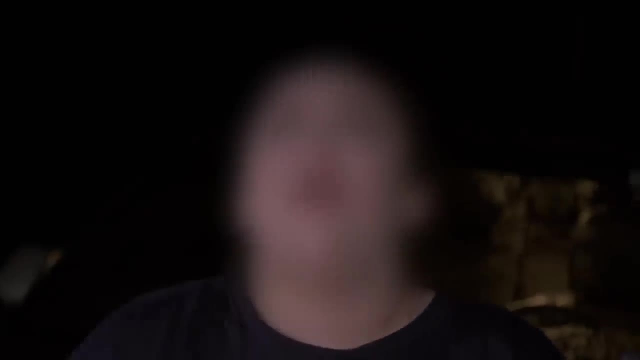 Marijuana, which is illegal in Virginia. You have the right to remain silent. Anything you say can and will be used against you in court. You have the right to Enter the pastor. Fuck you, I'm so pissed. All right, what are you pissed at? 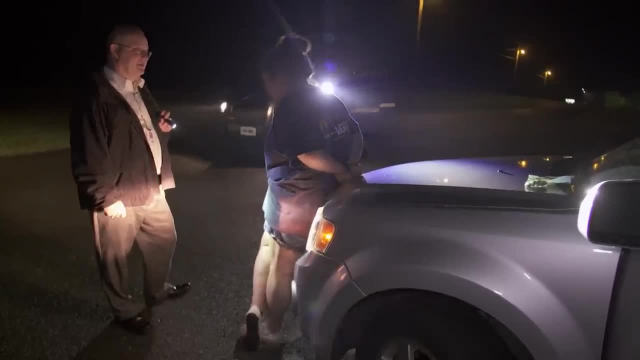 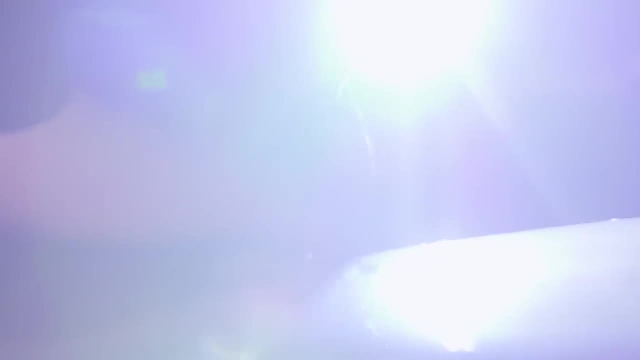 I just don't want to go to jail. You should not want to go to jail. Jail is not a pleasant place. Mark begins lecturing Courtney. The young handcuffed woman doesn't really have any other choice but to listen. We get to pick the sin that we want to do. 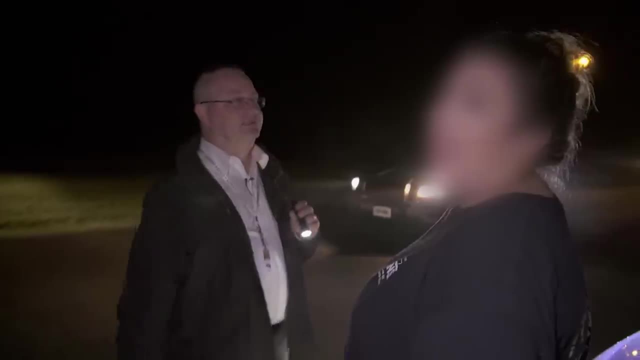 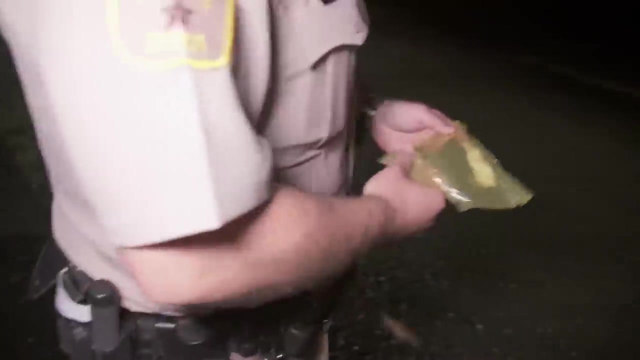 but we don't get to pick the consequence or when it comes. Does that make sense? I don't know. I'm so scared. I'm so scared. Daniel finds marijuana in the car And apparently it's a hybrid with the name wedding cakes. 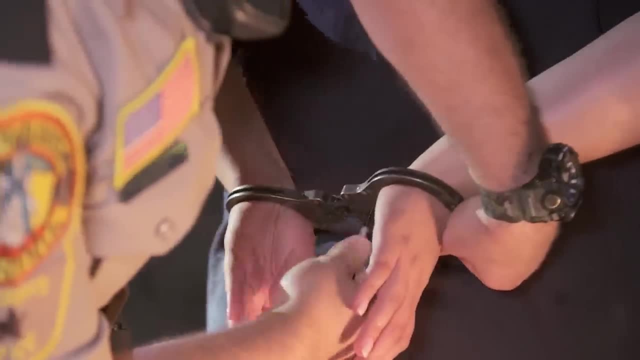 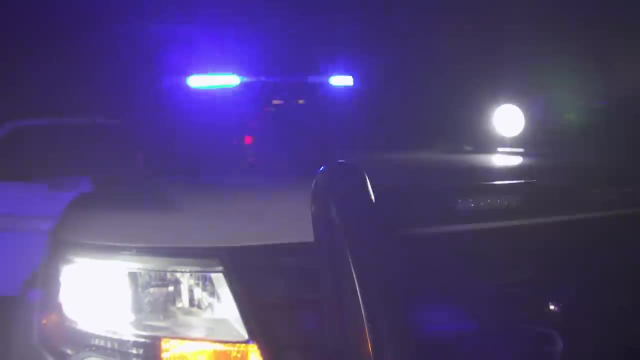 I don't know if that's sweet or not. He decides to remove the handcuffs once Courtney has calmed down a bit. The more you wiggle, the worse it gets. Daniel believes that faith can be the new shock tactic in getting people to follow the law. 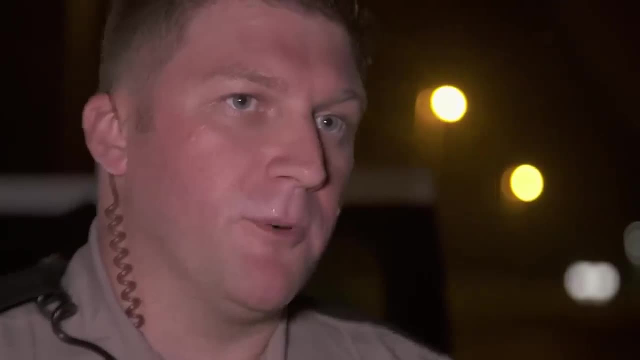 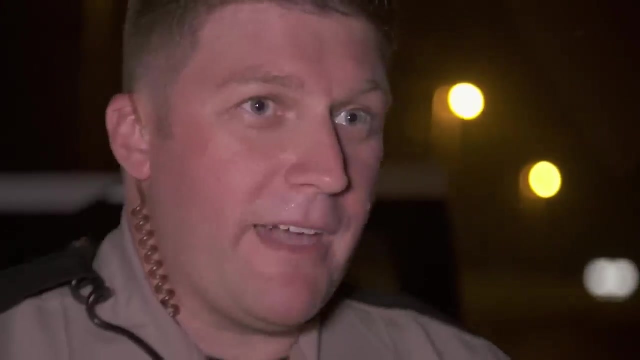 You know, 20,, 30 years ago people respected officers more Really. Yeah, They knew that if they got out of line- I hate to say this- they would get smacked. Legally we can't do that obviously. 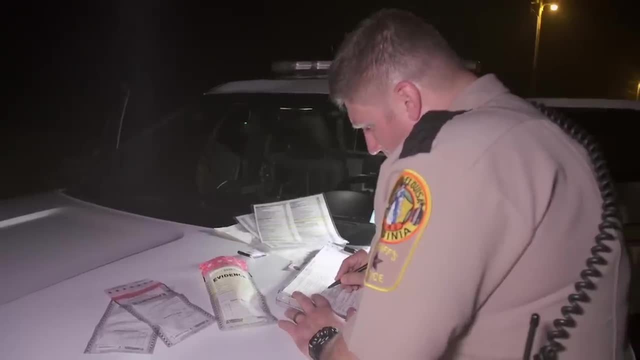 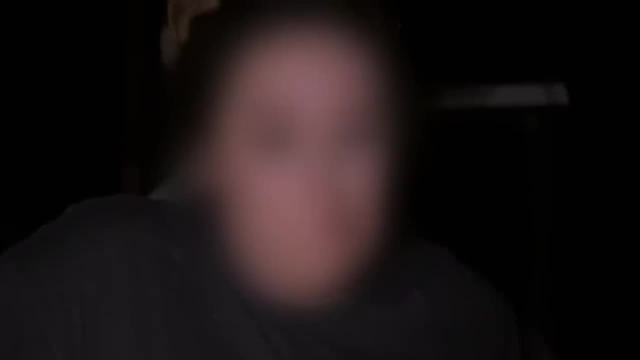 So now we have to talk to people. While Daniel writes up her court summoning, Mark keeps going with his sermon. Us finding you here tonight, I believe, was orchestrated by God, So I would say this is God saying: hey, I love you. 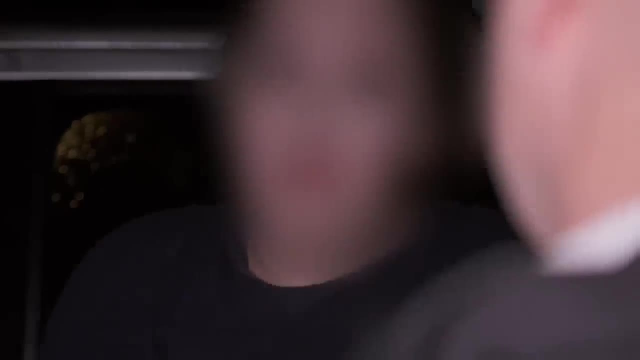 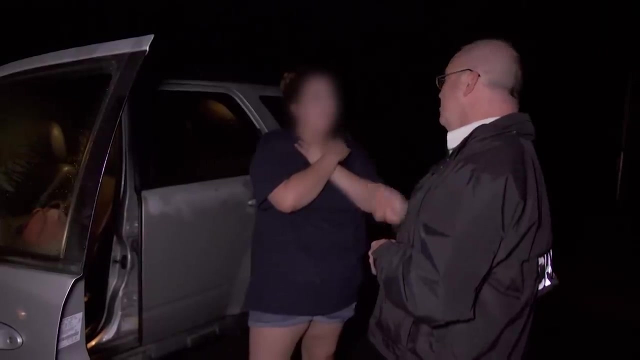 and I want you to go down a different path. Now, which one are you going to pick? I mean, I think this is a giant wake-up call for you. What I would like for you to do is to remember the feeling you had when he put handcuffs on you. 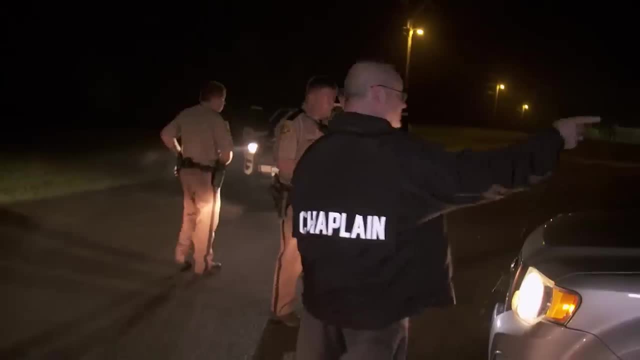 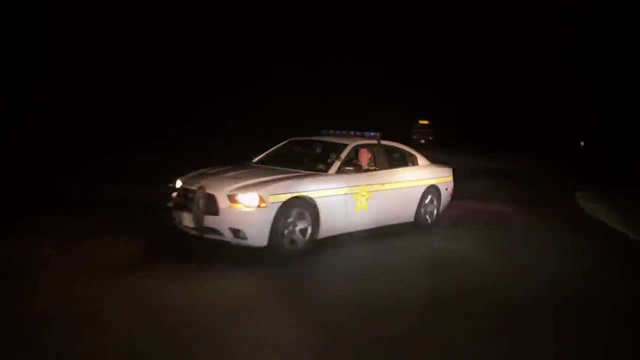 and you thought about going to jail. for real. Take care of yourself, Mark and Daniel. stop three other people that night. That was some skanky weed though, man. I'll tell you that. Whoo A pastor on patrol with the police. 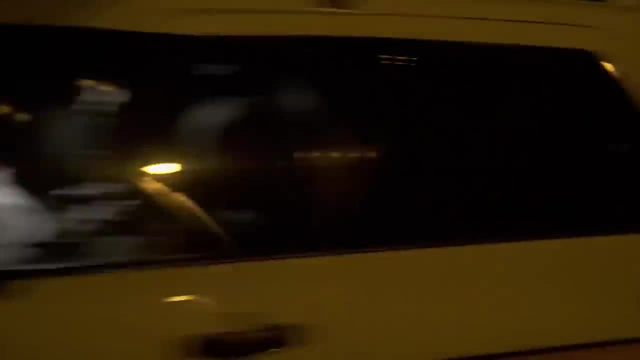 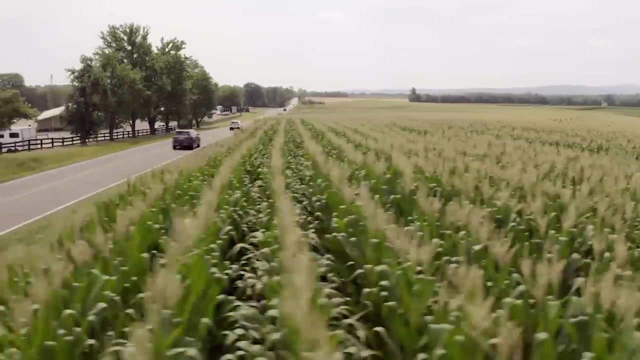 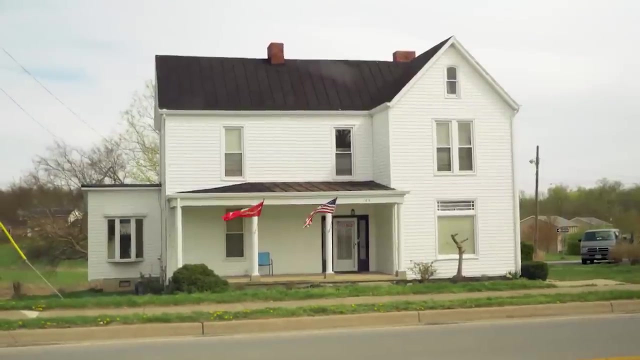 unusual but not unheard of here in the United States. In other states there are even scientists who give their life to God. Williamstown is a small, peaceful town in Kentucky. However, hundreds of tourists descend onto it every day to visit a surprising museum: the Creation Museum. 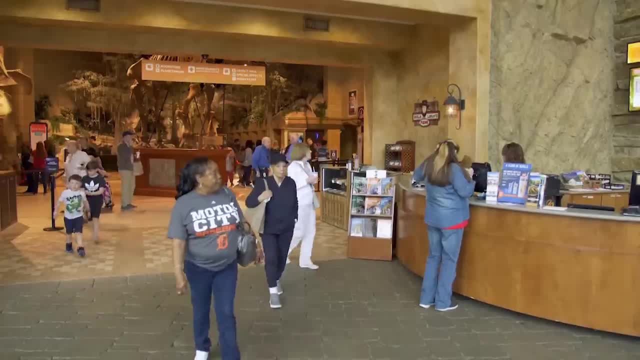 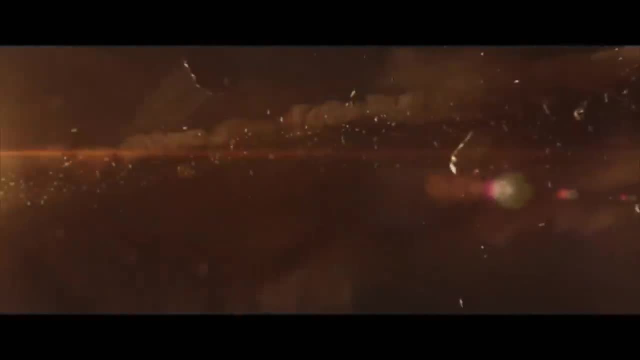 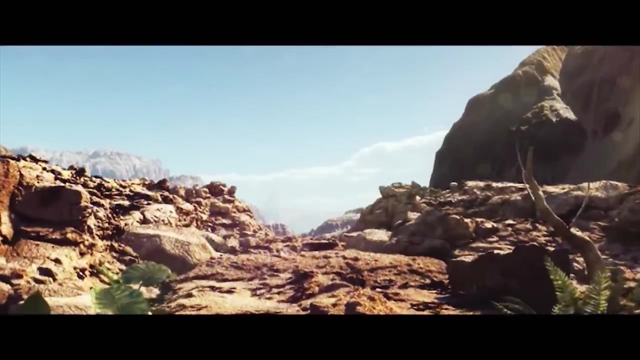 Visitors are welcomed with this film Denying the Big Bang and the world's 14-billion-year evolution. the creation of the world's largest museum, Williamstown, is one of them. Let the earth bring forth grass Exhibitions with pseudo-scientific information. 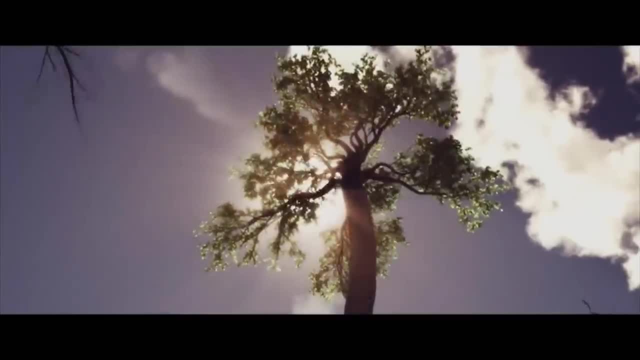 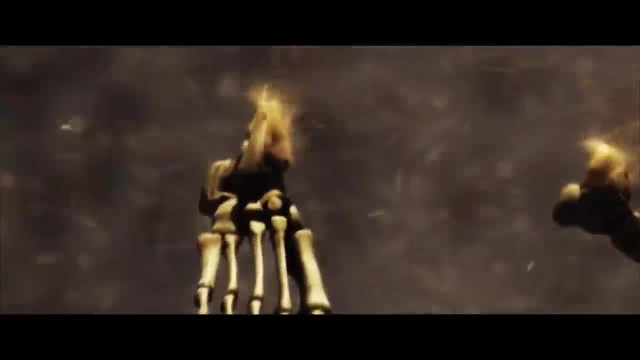 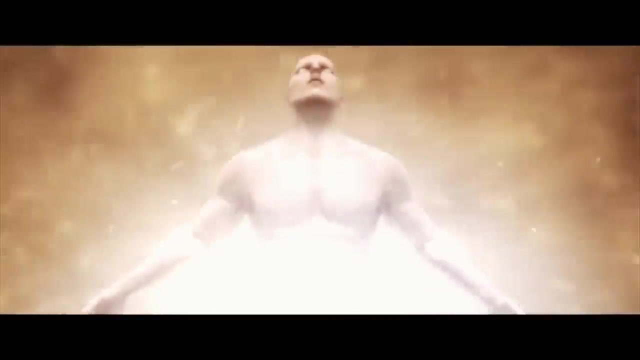 about how the world, its animals and mankind were created by God over a period of six days, around 6,000 years ago, as the Bible tells it. This school of thought is known as creationism. There is absolutely no scientific basis to this story, but it's one of many. 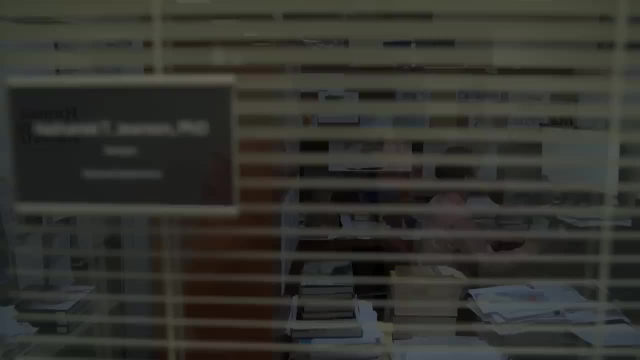 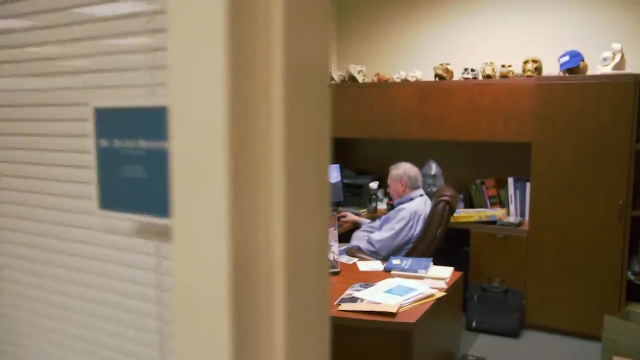 It's a story of the world. It's a story of the world. It's an interesting story, yet 42% of Americans believe it. The museum has hired ten scientists in an attempt to lend credibility to their theories. All hold degrees from universities that are recognized. 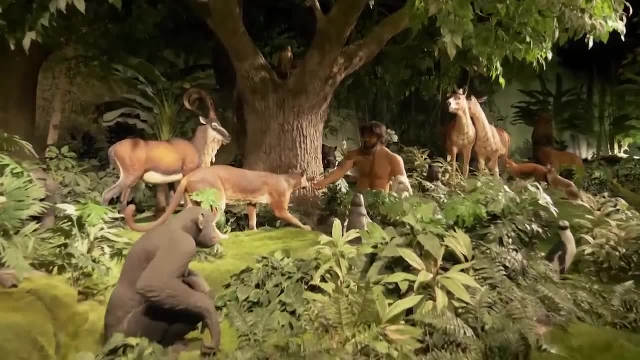 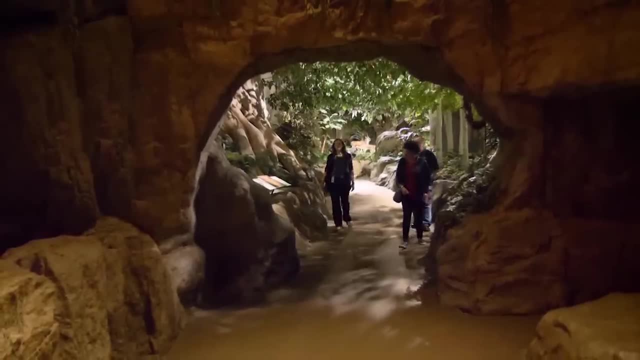 by the state, like Harvard, for example. I am taking you all to the through the Garden of Eden. Dr Gabriela Rocha de Carvalho Haynes has a PhD in paleontology and geology. Dr Gabriela Rocha de Carvalho Haynes has a PhD in paleontology and geology. 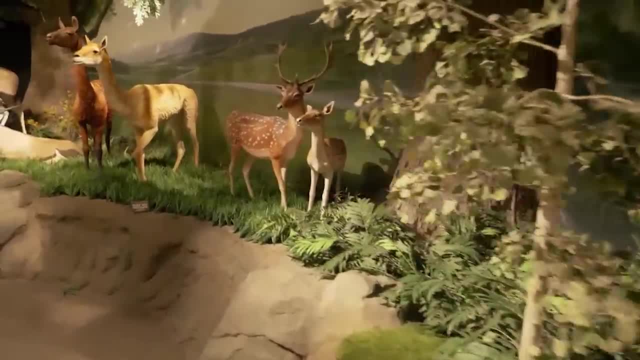 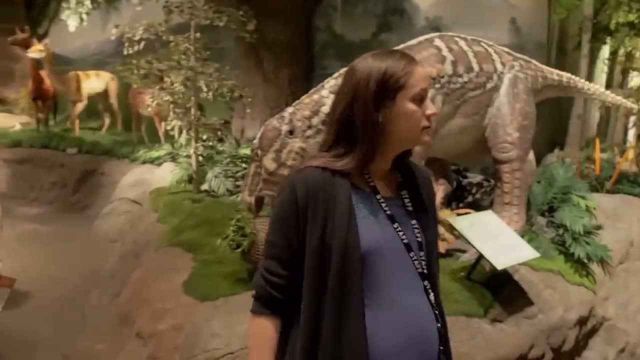 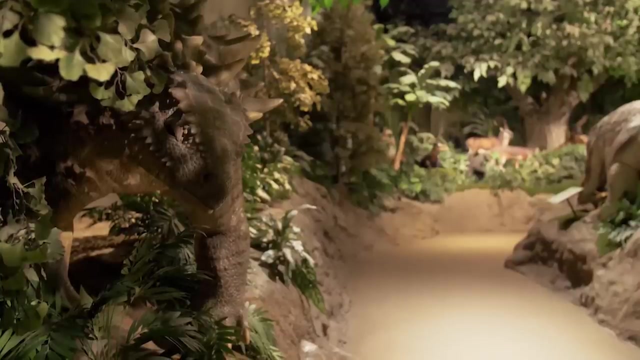 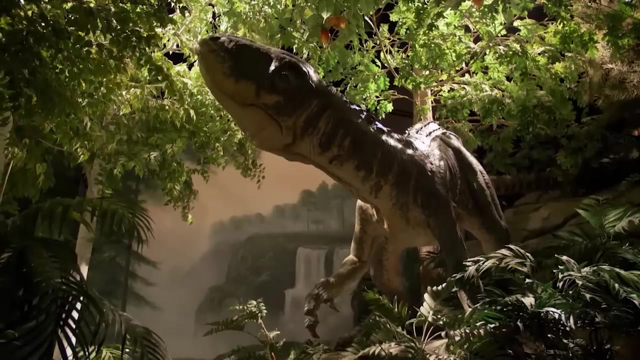 Scientists here have turned their backs on what they've learned at university, instead choosing the Bible as evidence to support their theories. According to them, all living creatures were created on the same day, 6,000 years ago. Every living creature on Earth, even dinosaurs. 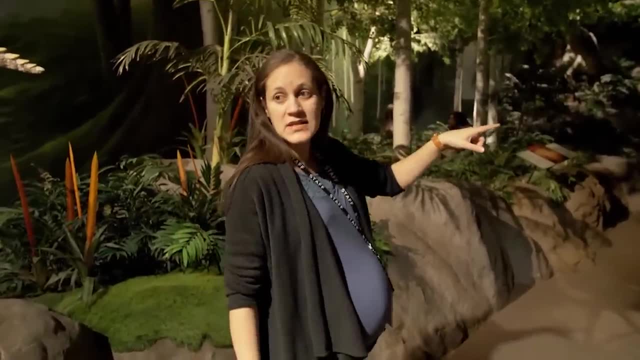 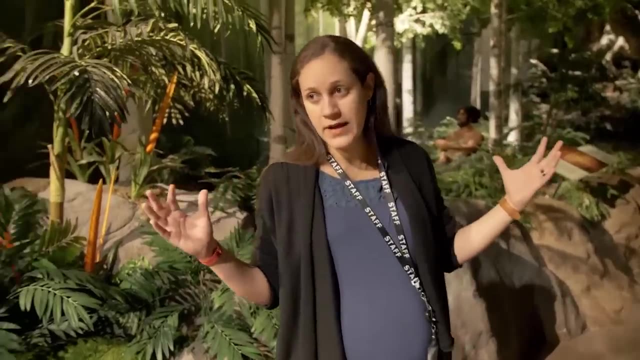 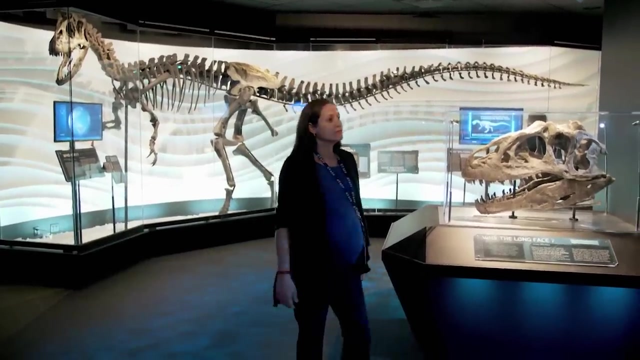 We can see some dinosaurs, and right there we can see Adam and Eve, So they were all together in the same environment. She tells this in spite of the fact that 60 million years separate the end of the dinosaurs and the appearance of the first humans. creationists are rewriting history, particularly with the 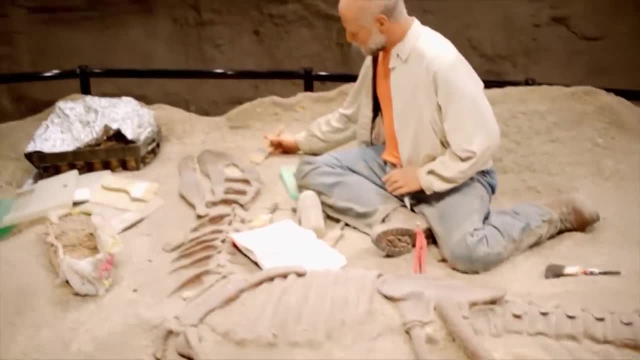 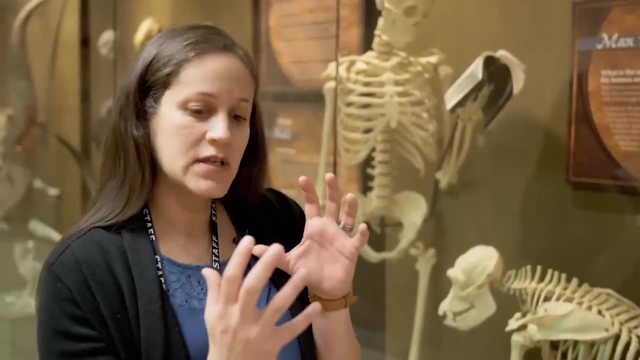 story of the discovery of Lucy, the skull of the most well-known Australopithecus, proof of human history And evolution. When they found the pelvis of Lucy, they looked and they said it looks like an ape, but it. 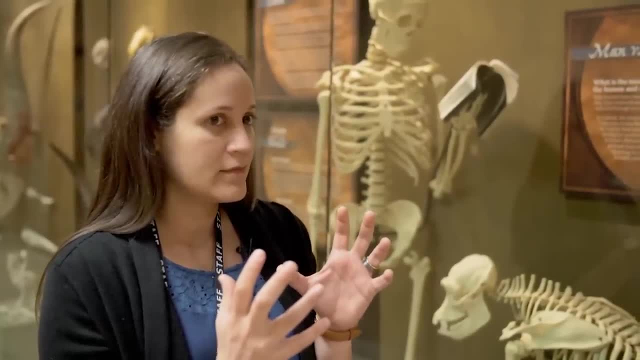 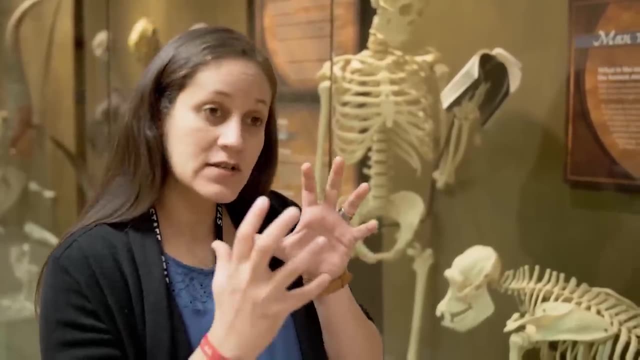 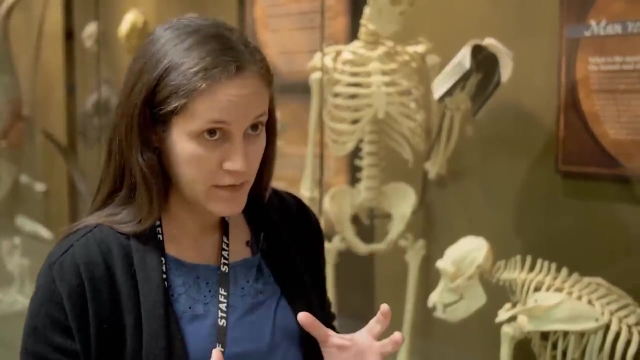 cannot be an ape. It has to be human. because they wanted it to be human. And then what they did? they took that pelvis to a lab and they reshape it in a human shape. The point is, when you don't have a Christian worldview. 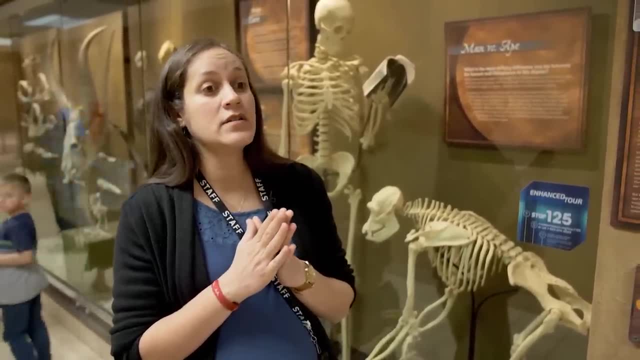 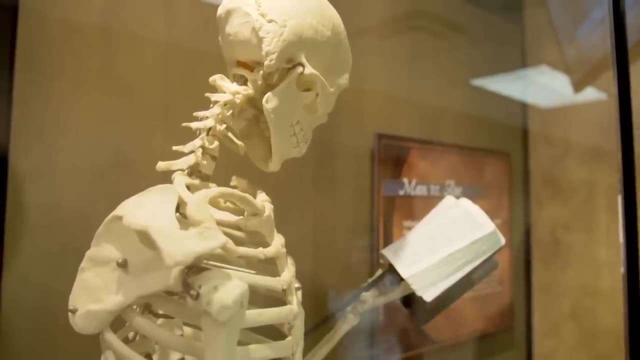 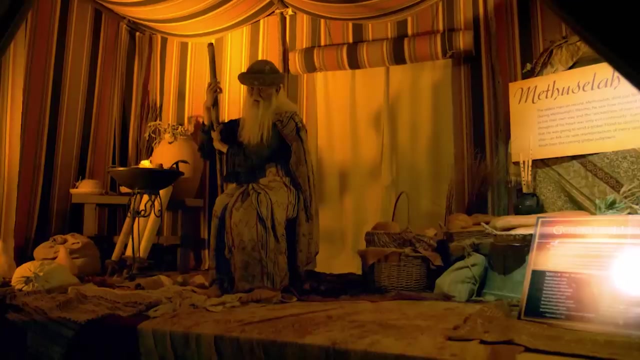 What kind of commitment do you have with honesty, with truth? What is life? According to Gabriela man's, evolution is a complete fallacy and conspiracy theory dreamed up by scientists and atheists. These creationist theories are taught in a number of Christian schools across the country. 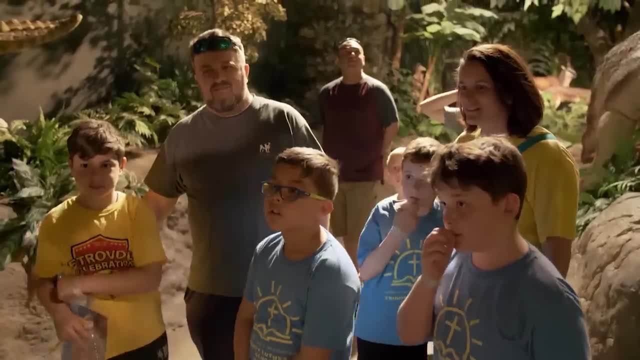 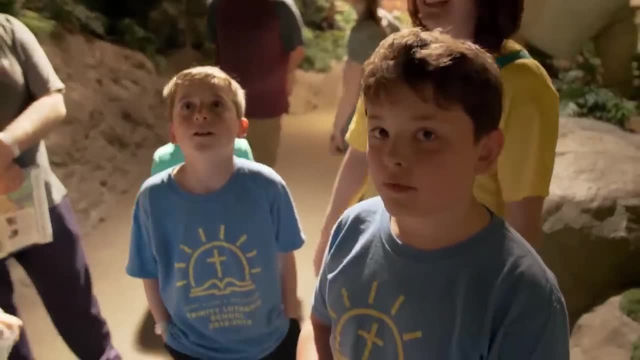 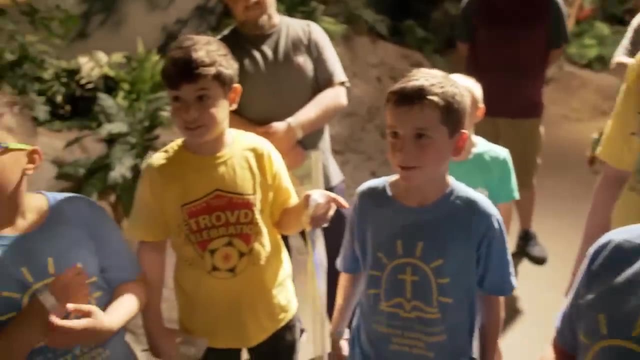 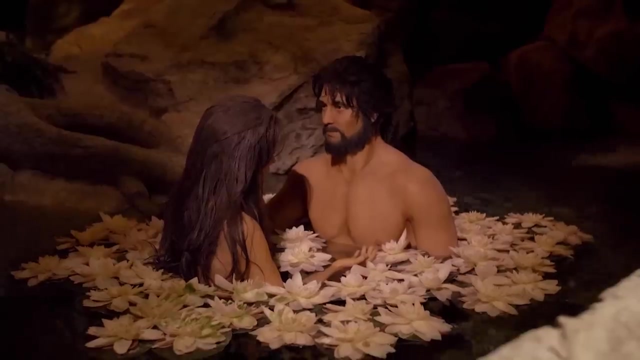 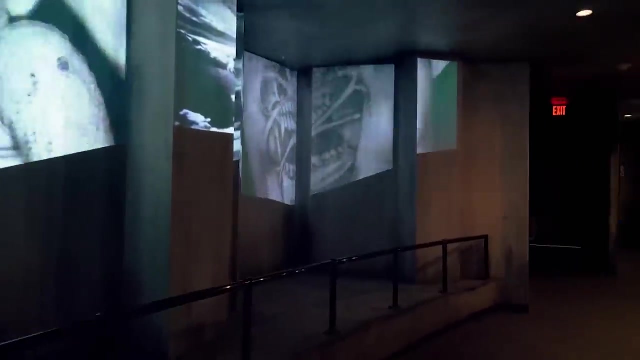 from a very young age. What do you like the most so far? Dinosaurs, Dinosaurs. This is the scene when Adam and Eve, they sin against God. The Bible explains that suffering and pain only arrived on earth after the first original sin. 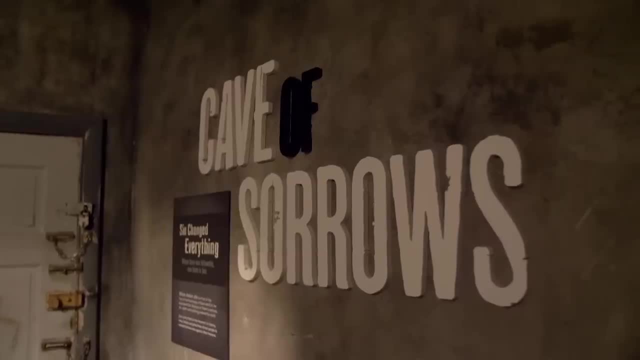 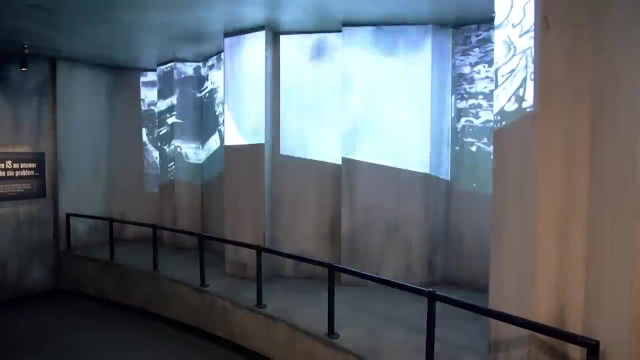 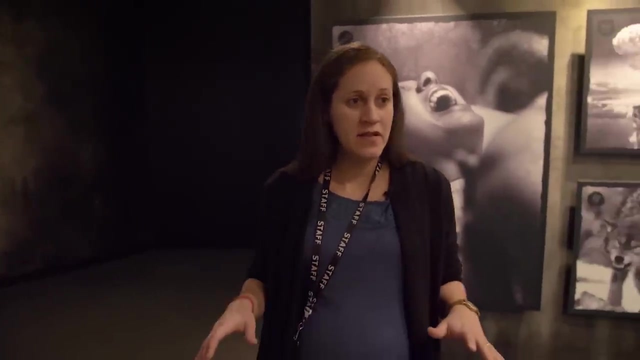 The museum has made a real house of whores or Cave of Sorrows of sorrows to depict this. Because of the sin, it brought chaos, It brought death. So the world is not safe anymore. We have wars, we have pain, as in that picture. 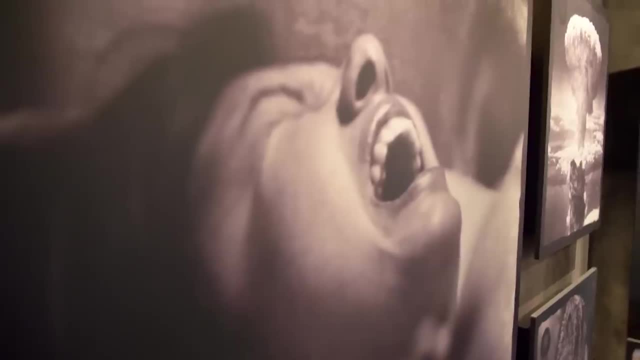 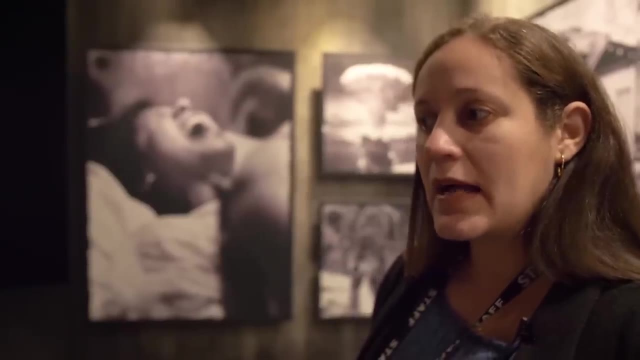 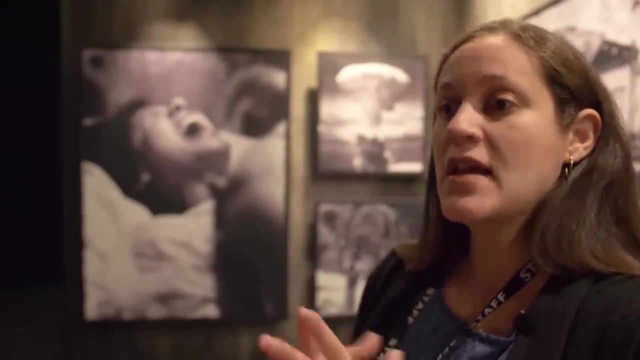 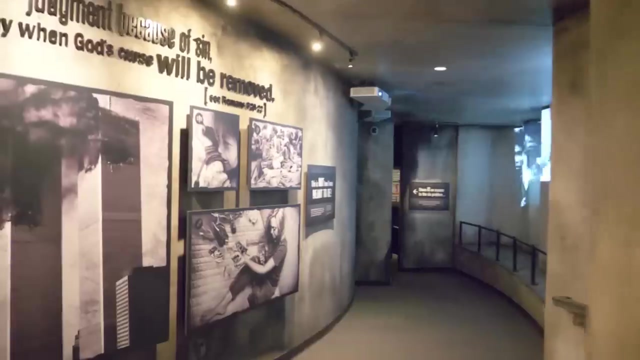 and I am pregnant now, so I can understand that the curse of the pain. Do you feel punished? Yeah, we all feel punished because of the sin, yes, because of the sin in our skin: Nazi concentration camps, the 9-11 attacks, drugs. 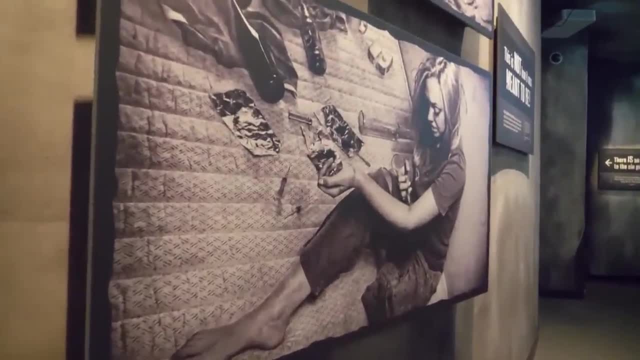 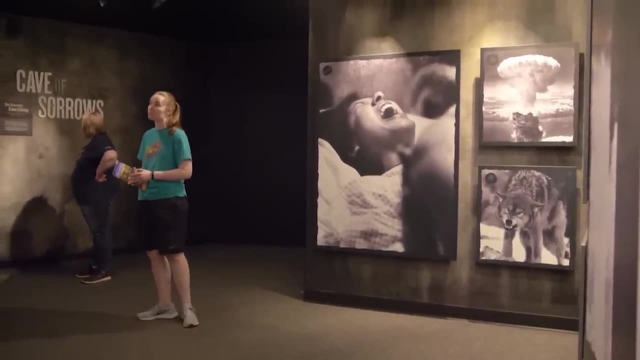 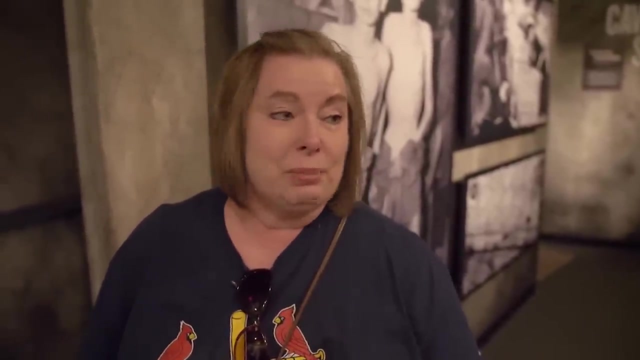 This is exactly what would happen for a creationist if one were to stray from God a corridor to scare Christians into staying on the righteous path. I get emotional at everything. I just I don't know. I just, I mean, I believe very strongly about it. 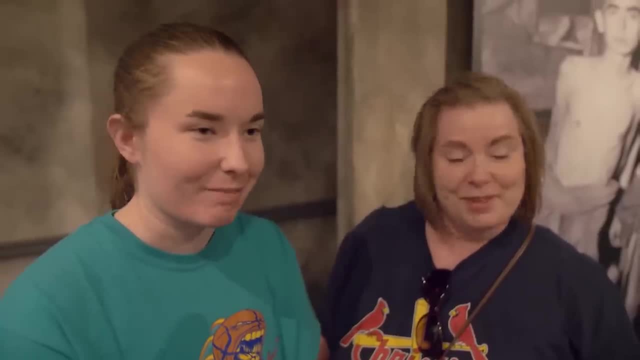 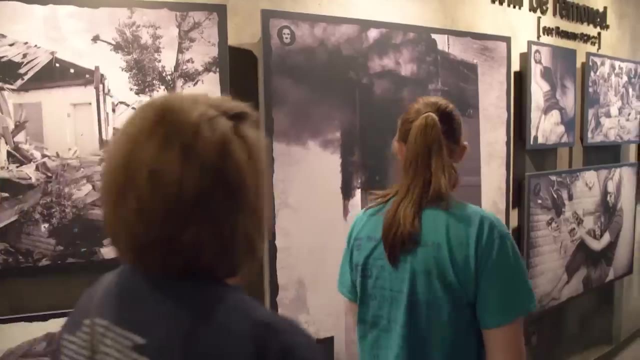 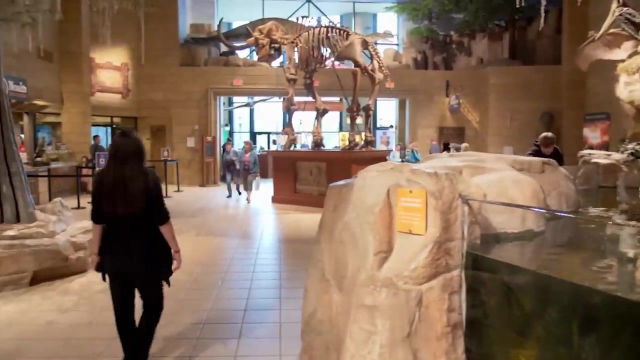 Yeah, it's very powerful the imagery. It's scary- Not really. I know where I'm going, so nothing to fear. The 70,000-square-foot Museum of Evangelization and Pseudoscience has attracted more than three and a half million people since it opened in 2007.. 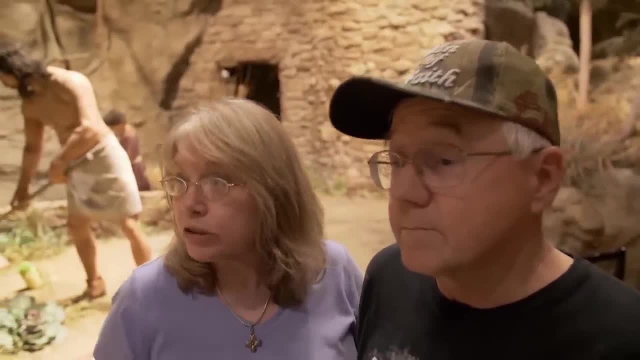 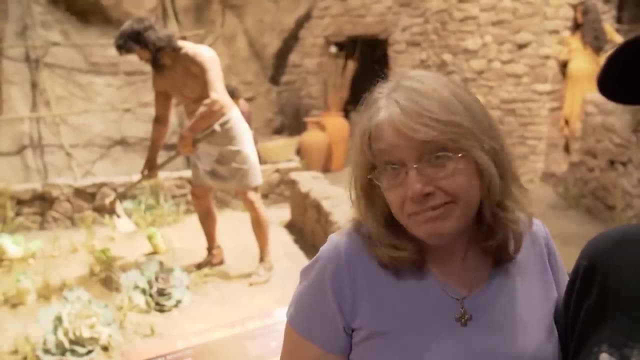 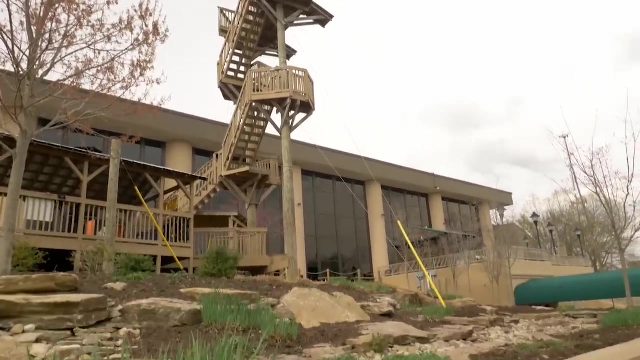 I think it's awesome and I would love for my grandkids to come see it before they're taught the opposite. Why? Because this is what I believe in. The museum is run by a creationist organization called Answers in Genesis. Its directors have gone even further. 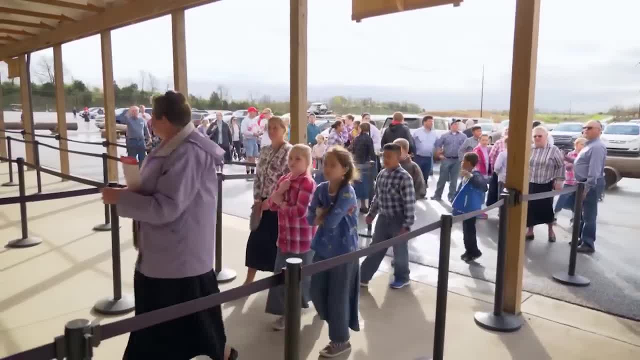 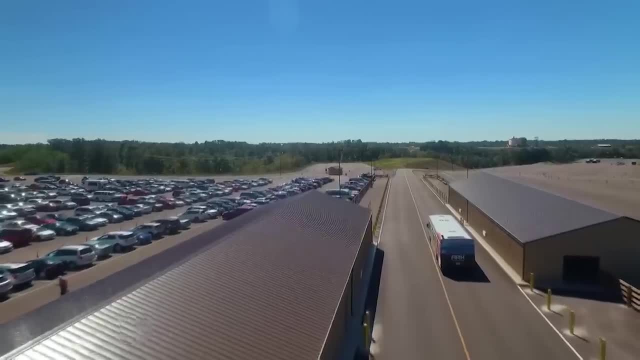 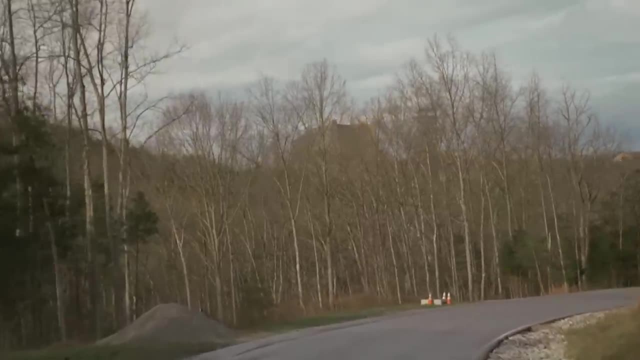 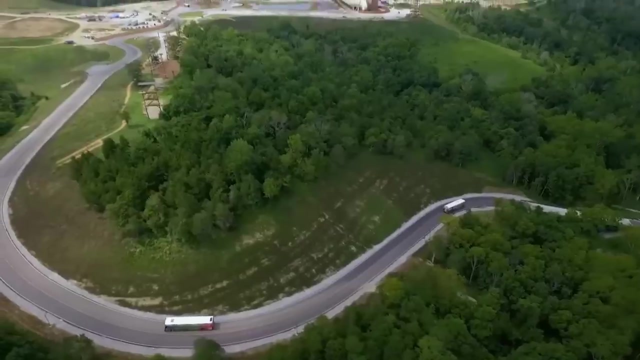 to spread their theories. Thirty minutes from the museum, tourist groups are boarding this bus. They've traveled from hundreds of miles away to visit an out-of-the-ordinary Christian tourist attraction. Bus three approaching the bridge, parking lots on it, A gigantic Noah's Ark. 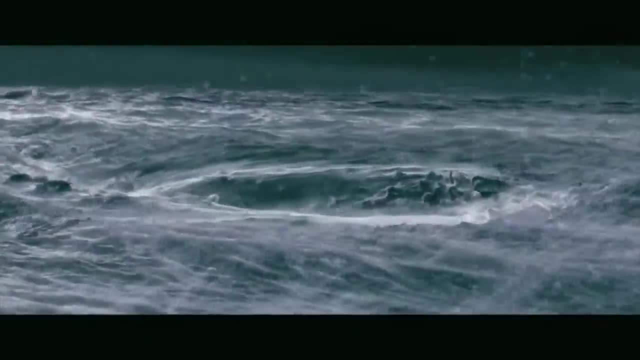 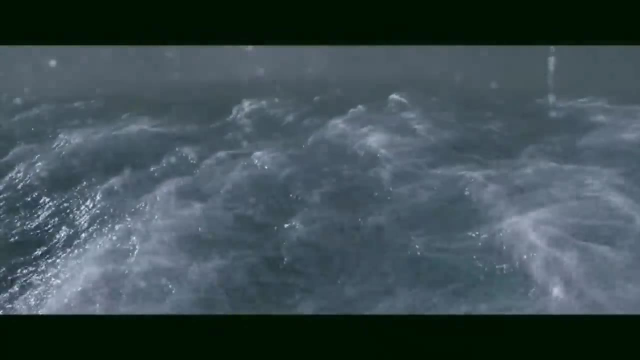 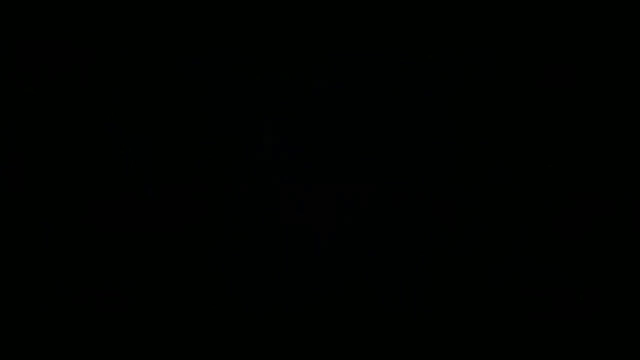 The Bible says that God destroyed Noah's Ark and destroyed almost all life thanks to a rainstorm that flooded the entire planet. Only Noah and his family survived, along with the animals he had sheltered in his ark. This modern half-museum, half-attraction ark. 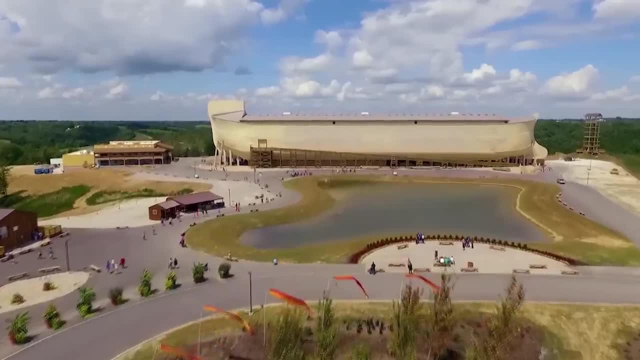 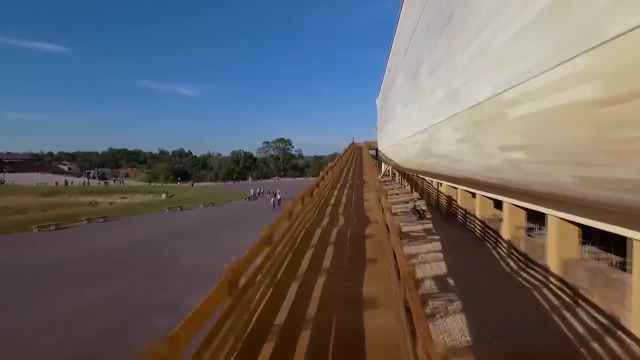 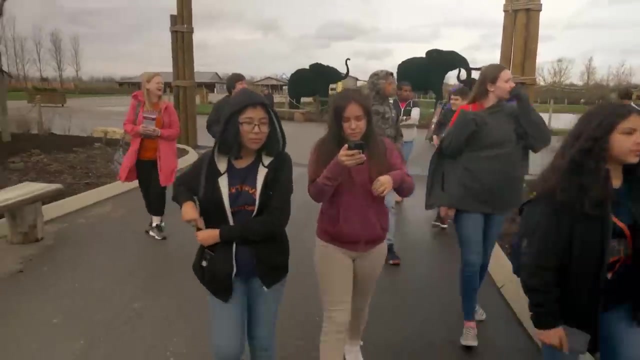 tells Noah's story. This colossal structure measures 500 feet long and 50 feet high, weighing over 8,000 tons. It's a huge ark, Guys. this way, Guys, this way, There's a monument. Tara and her students have traveled. 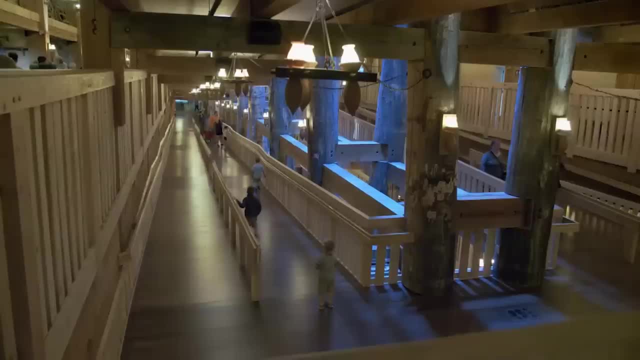 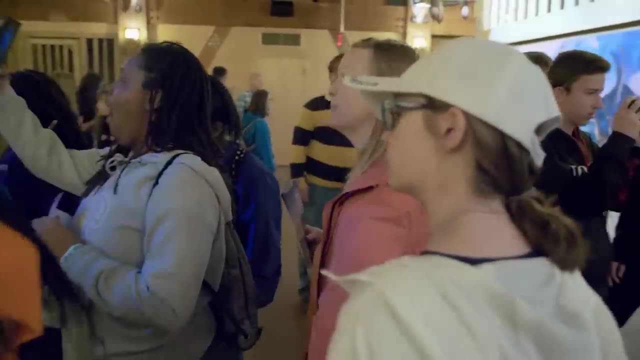 all the way from Virginia. Entrance to the ark costs almost $50 per person. Just make sure you don't walk off the family. Oh, that's cool. That'd be cool. T-walls- look at a picture Ready. Can I get one? 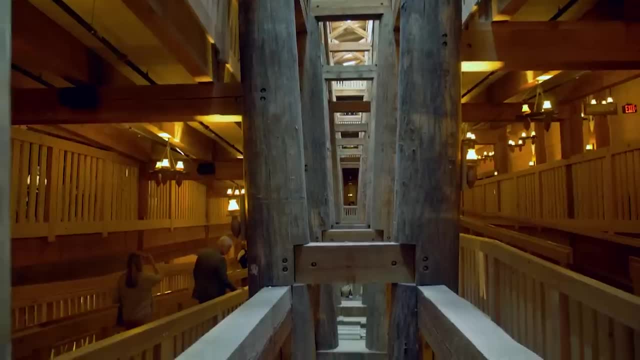 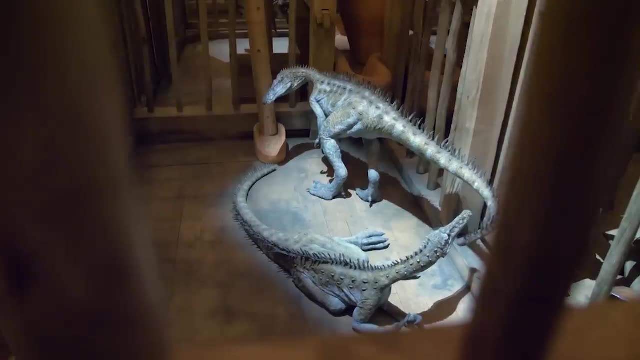 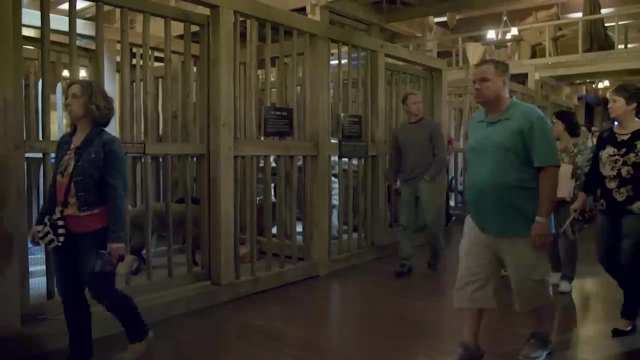 Inside, every detail of the story has been painstakingly recreated. Animals such as bears, whales and other animals like this have been left behind. Bears, hippos, even dinosaurs in cages, the sounds of the water and the animals. 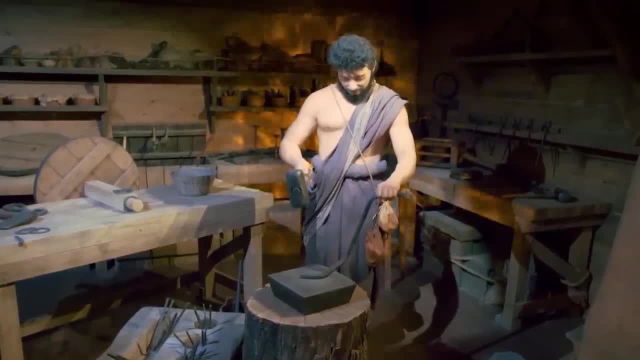 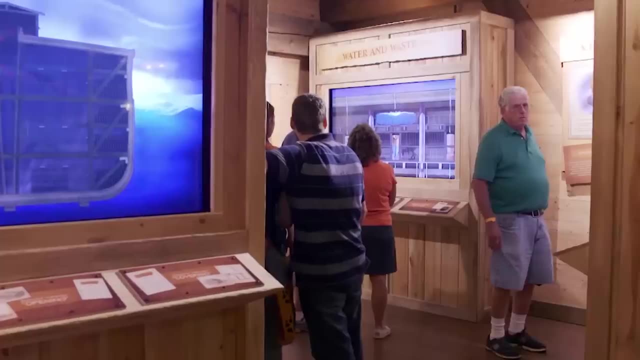 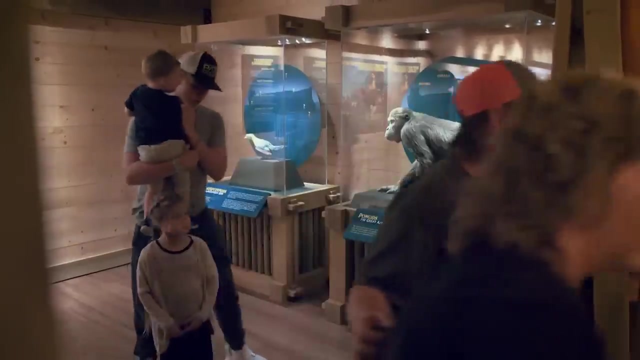 even Noah and his children at work. LCS, all LCS, let's follow. Tara teaches creationism in her class. This is legal for private schools in the US and this tourist attraction is an excellent visual tool to support the ark. It's a great way to learn more about Noah and his theories. 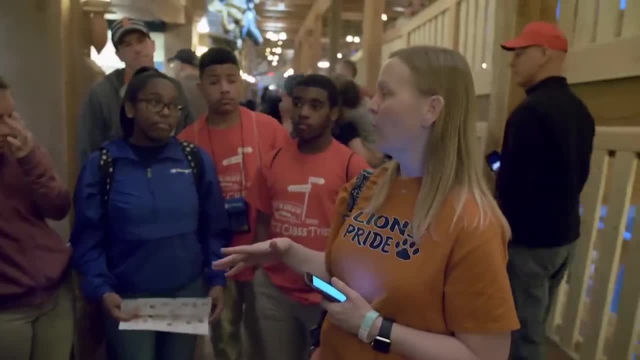 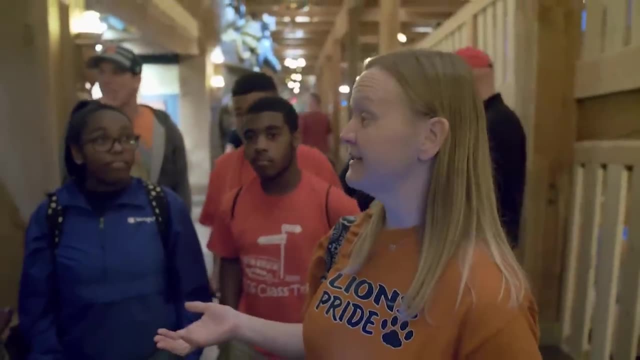 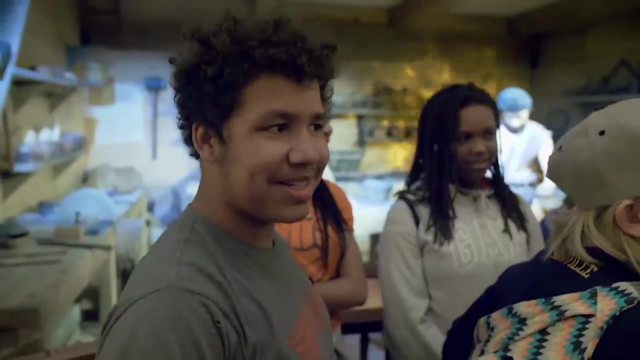 Does anybody know how old Noah was when he entered the ark? 600 years old, 600 years old. And does anybody know what the Bible says about how old he was when they left the ark? Raise your hand- 601.. 601,, that's right. OK, why do you think Noah lived to be 600 years old? I think that it would be the same way that we live to be, you know, 80 or 90 years old today. It's just the body aged differently back then. 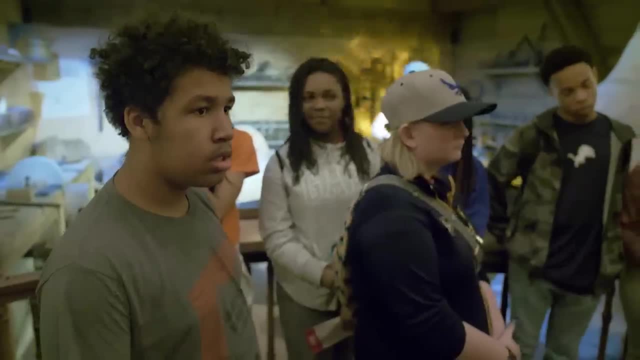 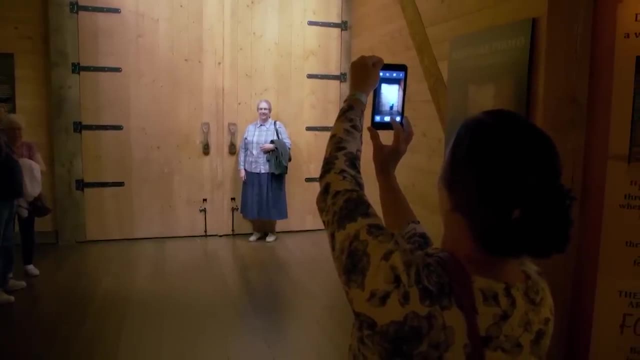 These Christians believe we live for hundreds of years during Noah's time. What do you call it? Nadine and her group have traveled from North Carolina. I love it. I love it To think in our world that it's pretty wicked right now. 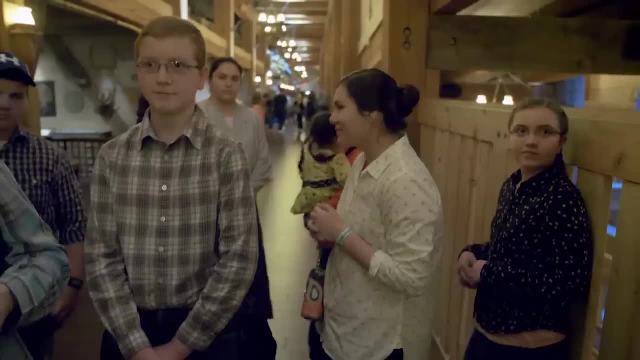 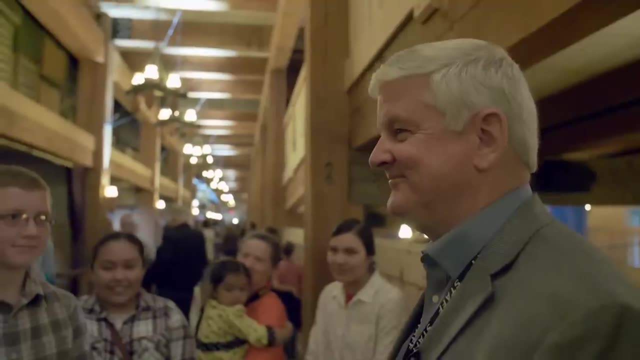 there's some good Christian things. I love it. Nadine is won over. She does, however, have some feedback to pass on to the ark's director, Patrick. I wish that the women were dressed a little more decently. The women. 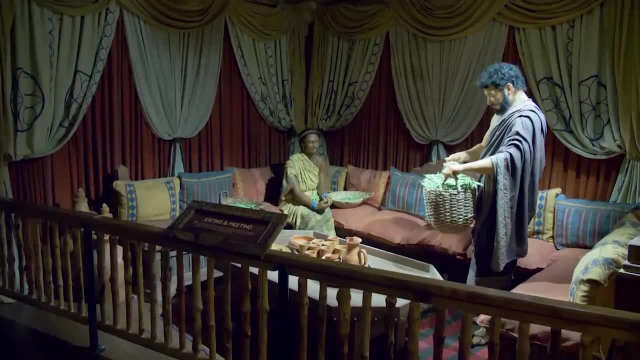 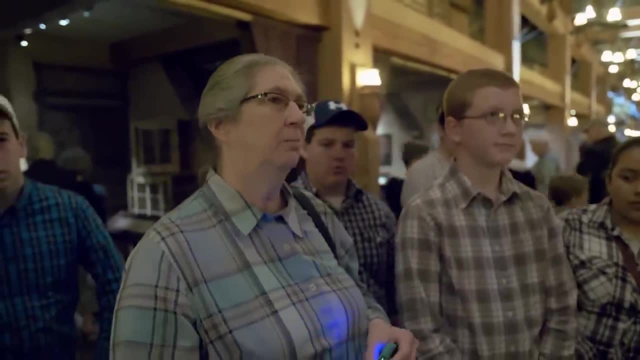 And we are Noah's wife and the three daughters-in-law. Really, Some of the wax figures I think are a little bit. I wish it was a little more modest. Thank you for that. We tried to be as authentic as we could. 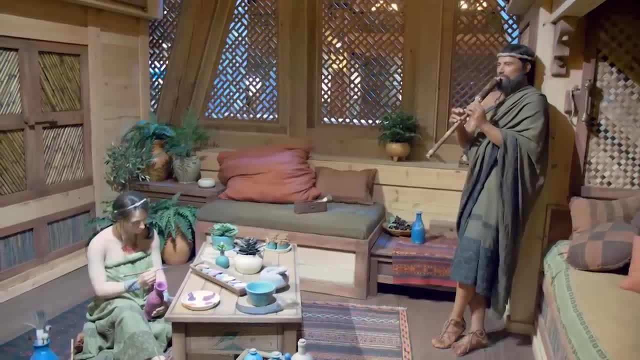 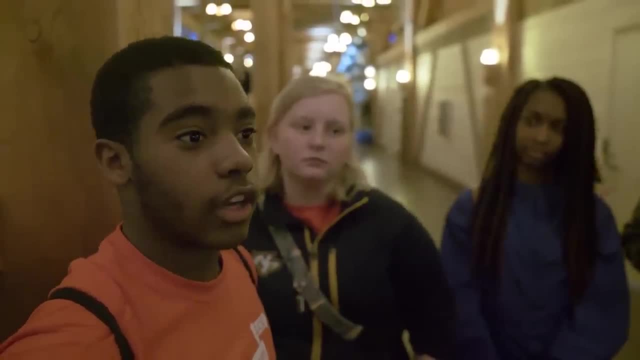 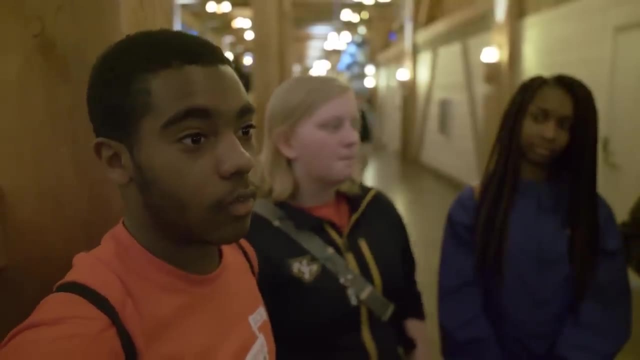 These women were a little too naked for Nadine's liking. Terrace students, however, have some questions. Feeding all the animals: it'll be really hard, because you got like 1,300 animals, to be exact, And I know like feeding all of them will be really hard. 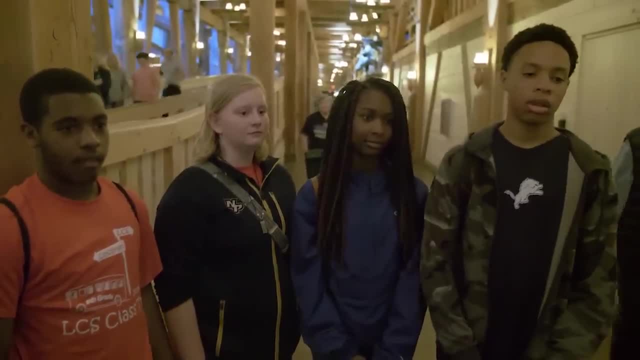 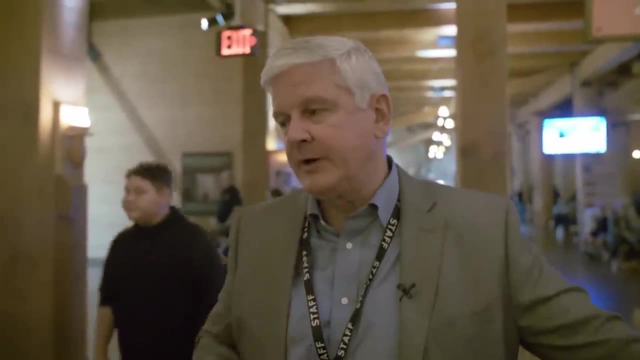 Of course Patrick has an explanation. So for eight people they didn't have to see every one of those animals every day. so we think they would've probably had some automation in the feeding. That's why you see the feeding troughs and Europe and so on. 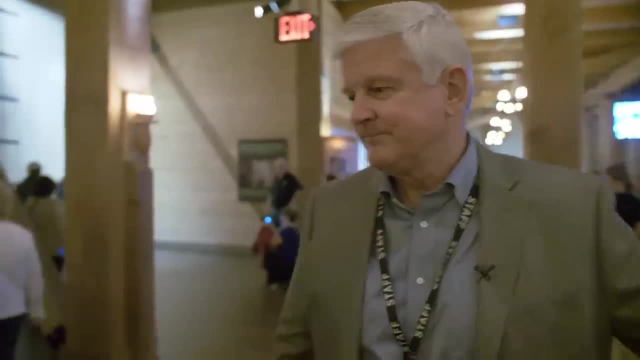 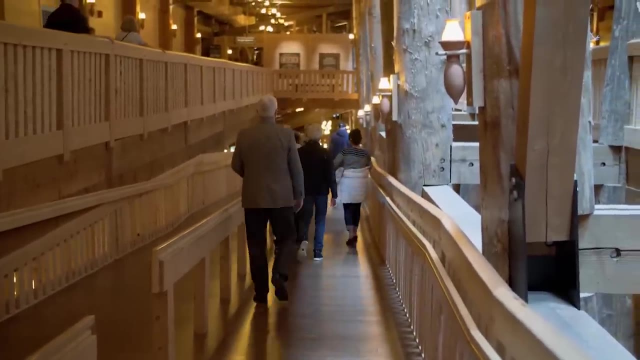 That's a long line. That's a long line. That's a long line. and the different ways to feed the animals That make sense. Yes, sir, Okay. This huge Christian monument has been funded by private investors. It cost over $100 million to build. 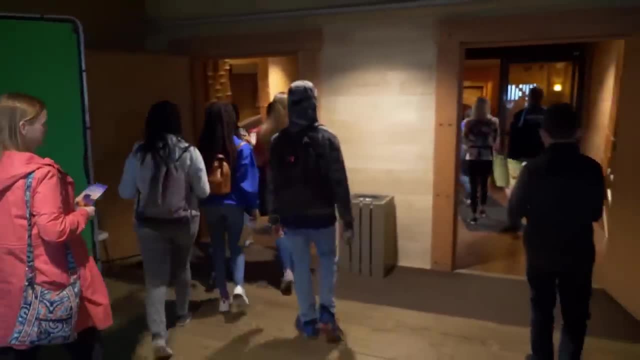 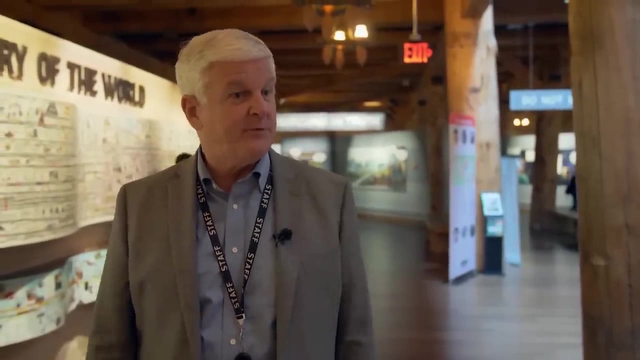 but has become a true tourist destination. We wanna try to draw people in to hear the message And you know, quite frankly, if you don't make it fun then people probably wouldn't come. But Christians like to have fun too. A huge restaurant. 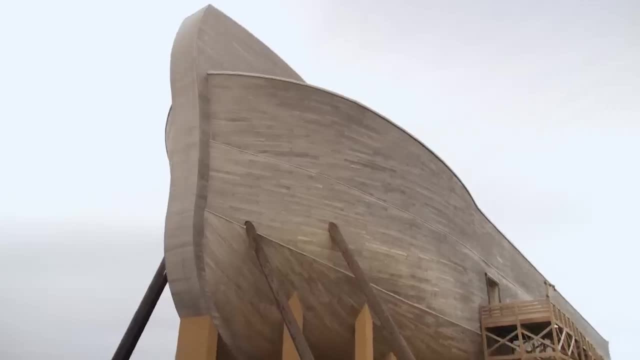 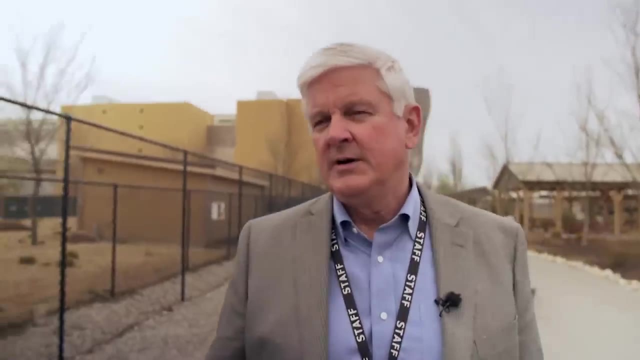 a zip wire, even a petting zoo. Noah's Ark is the Disneyland of the Christian world and it's highly profitable. Before the Ark, we were probably a $30 million company and now we're about a $110 million company. 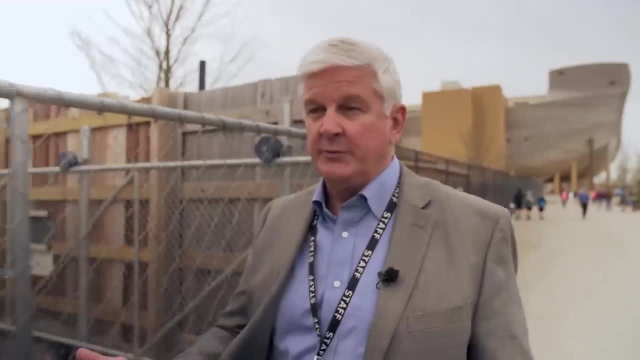 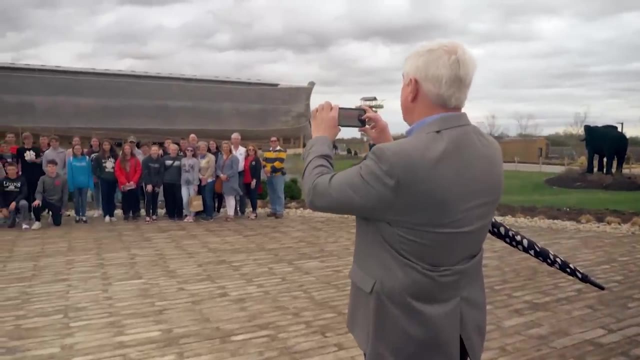 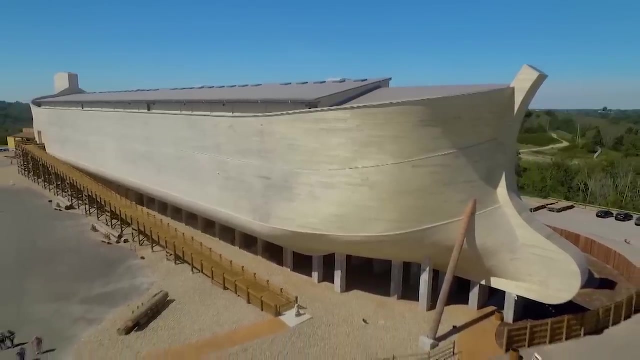 So the Ark has really exploded, our ability to reach people. That's the real, that's the big point- is that we're able to reach more and more people. Giant Noah's Ark, Everybody look happy. Music festivals, schools, museums, Evangelists will do absolutely anything. 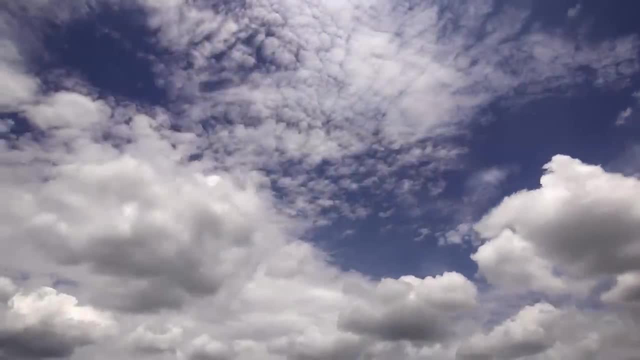 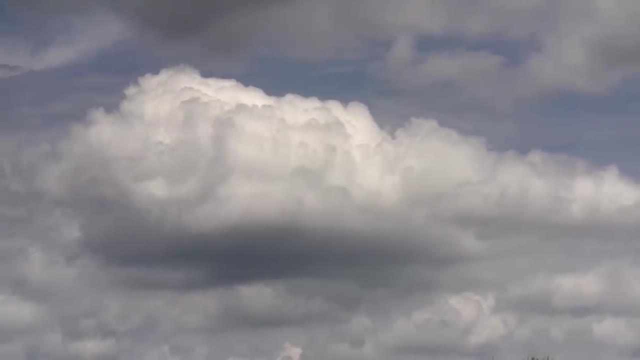 to keep their faith alive. There is, however, a part of the population who are starting to turn their backs on the Lord. 23% of Americans today claim to be nuns, That is to say, without religion. It's a historical record, but it's not like that. 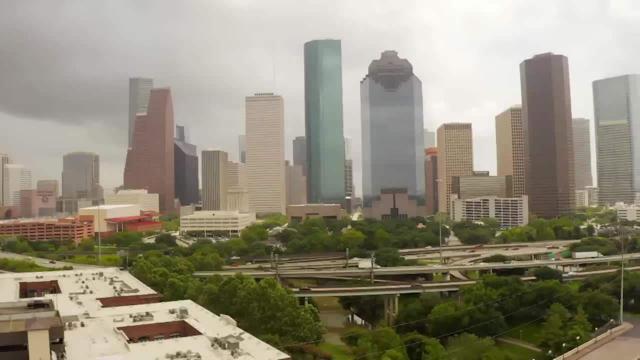 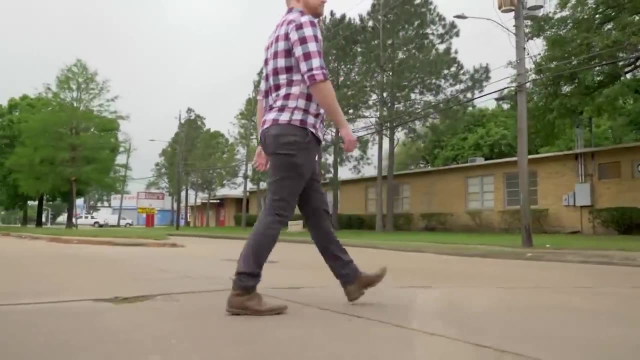 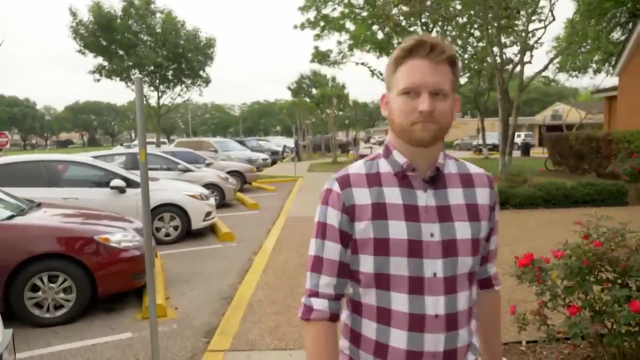 record for the US. Houston, Texas is an ultra-Christian city and it's not easy for the atheists that live there. Brian is a 28-year-old engineer. On this Sunday morning he won't be heading to church Every Sunday in church growing up, including many Wednesday night services as 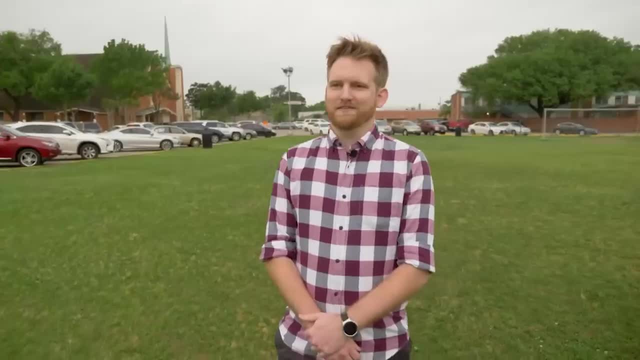 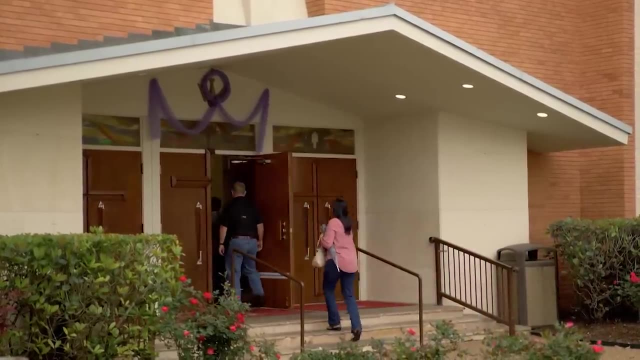 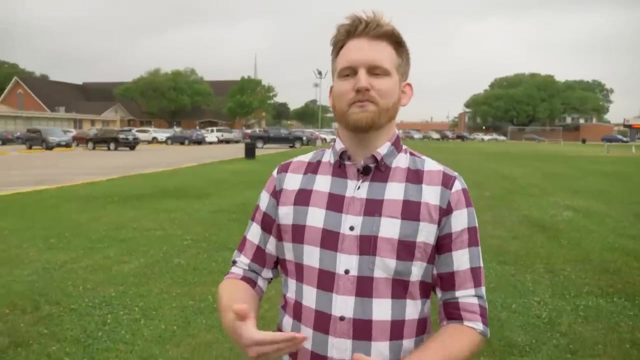 well as some Thursday get-togethers with the youth group. So it was a big part of my life. Brian also studied at a Christian university, but today considers himself a nun, an atheist. I left religion, kind of it was a few events all happening at the same time As I was learning more. 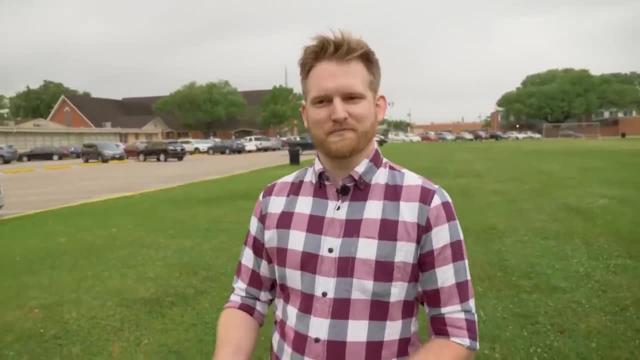 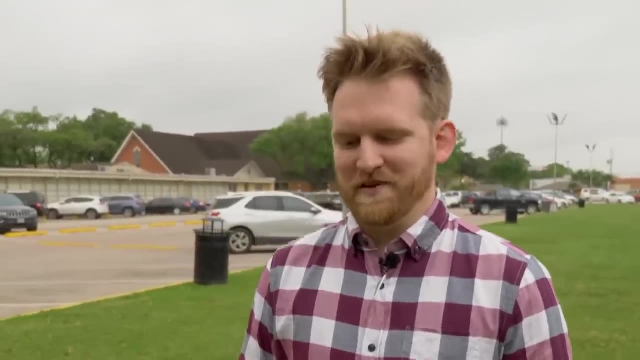 about science, I was starting to have more trouble reconciling it with my faith, And I started dating a girl and she was an atheist. And finally, as you know, my faith was getting shaky. my best friend came out to me as gay. Everything I knew about gay people was wrong. 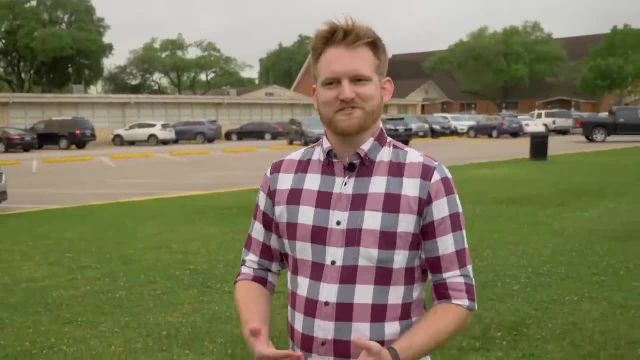 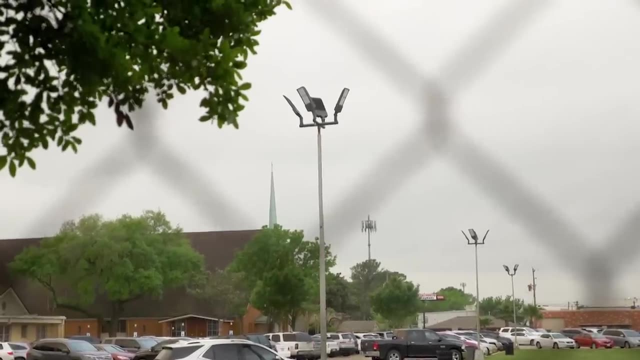 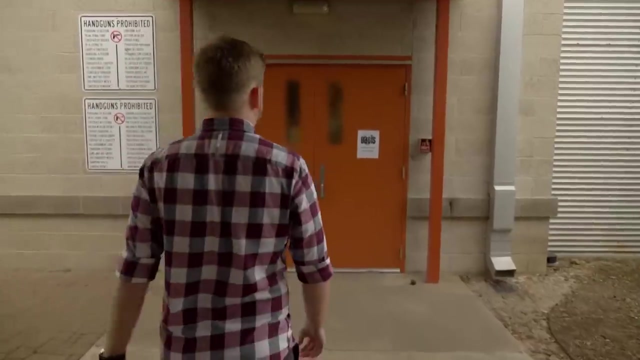 And at that point I had to kind of step back from church and say: you know, I think this community is not quite for me anymore. In the United States, religion creates a way of life, a community which atheists are cast out if they choose to give up their faith. As a way to combat this, 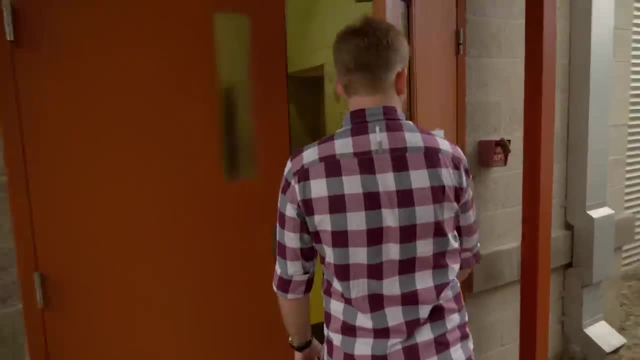 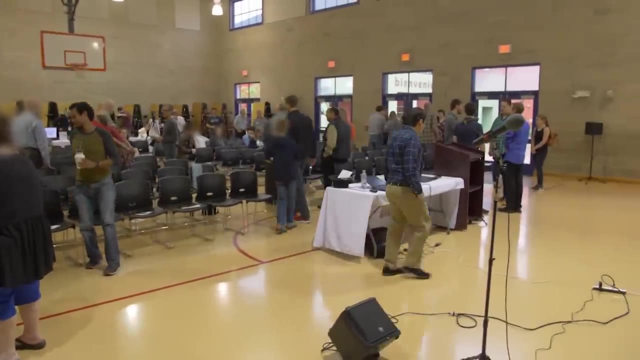 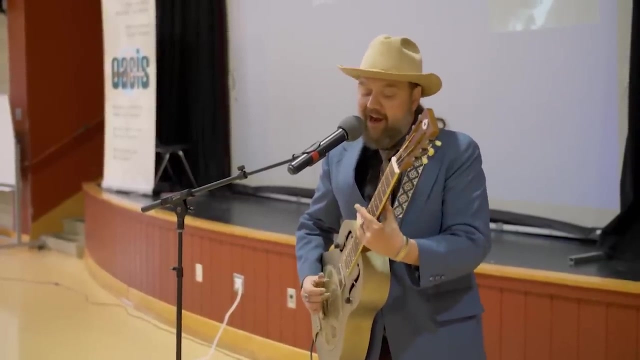 exclusion. atheists gather together at the same time as Sunday Mass. How are you? I'm good. how are you? Surprisingly, this atheist meeting takes place like a church service would Well, the Texas girl broke my heart and she's on my truck now. 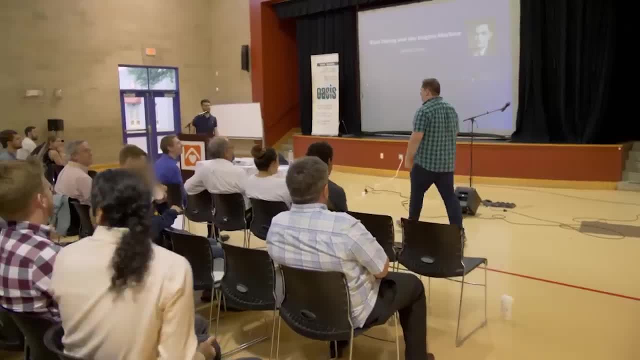 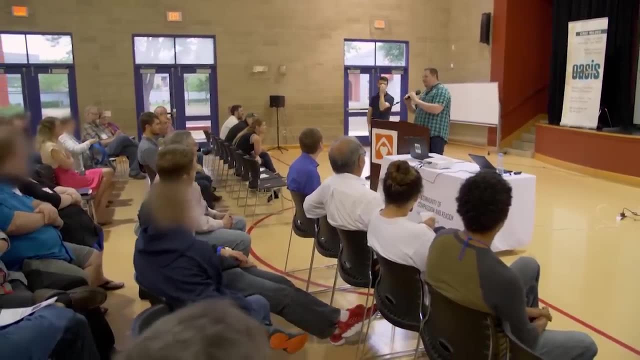 And discussions about science instead of God. The atheists even crack a little joke. It's so wonderful to be here and love that story today. It does feel a lot like a church model, and I think it's because it's what people like. 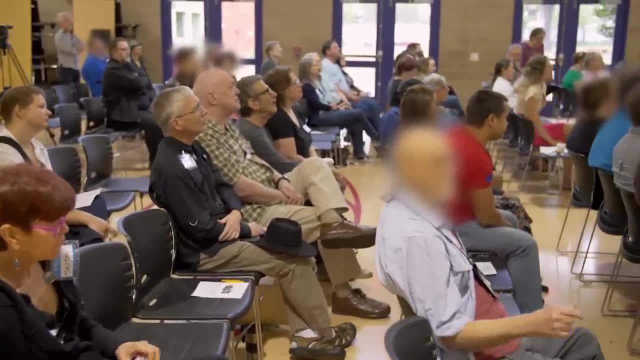 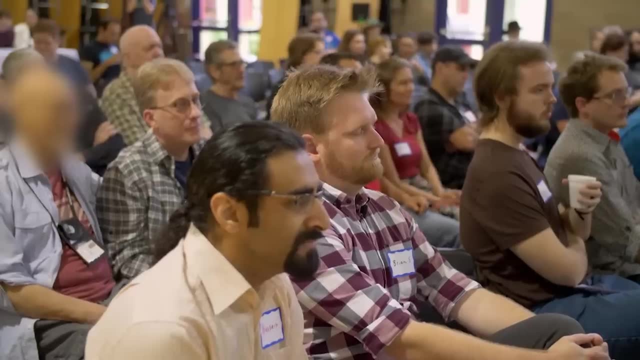 Brian seems relaxed, but a number of participants refuse to be filmed. John, one of the organizers, explains why: Because of the stigma that's still attached, especially in the US, especially in a place like Texas, to not being religious. 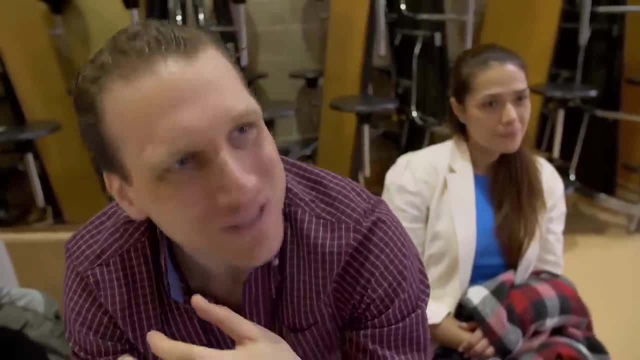 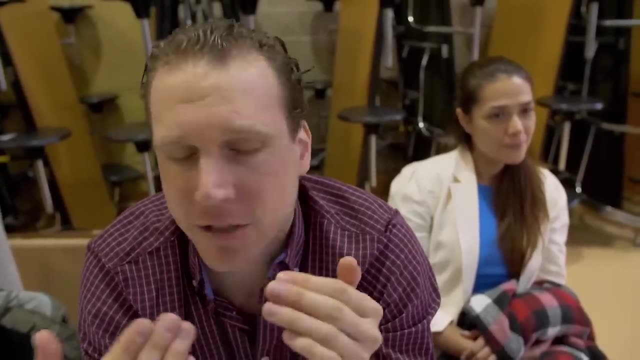 And being non-religious is sometimes almost like being gay. You kind of have to come out to your family, and people need to do that on their own terms whenever they're ready, And so for that reason, there's a lot of people that haven't even told their families. 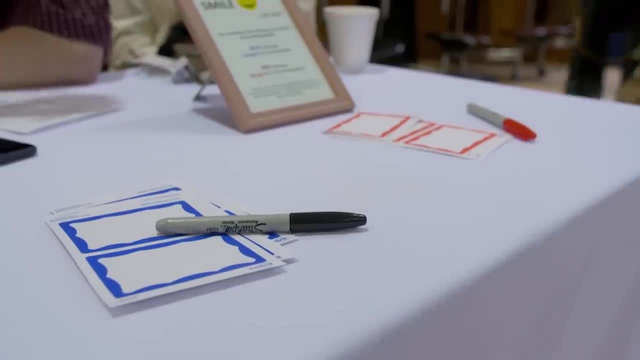 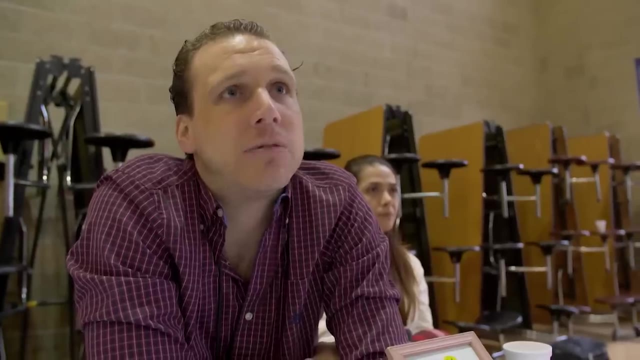 that they're not religious anymore. People are now coming out as atheist just as they would gay, But Christians employ the same punishment to both. To go and leave religion is almost kind of like turning your back on your culture. It's not just going to church. 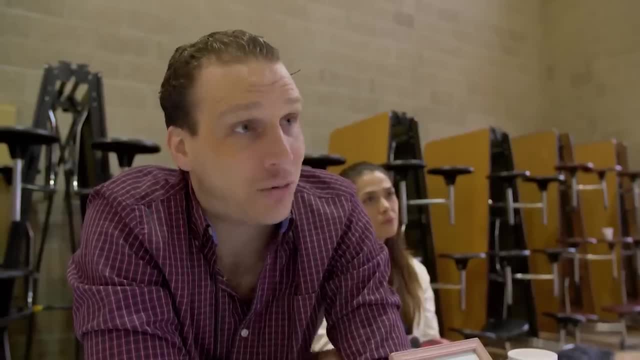 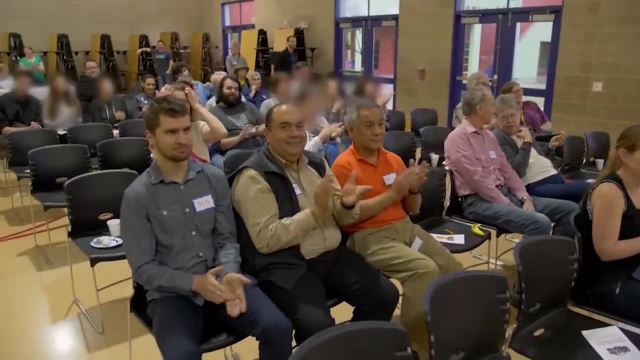 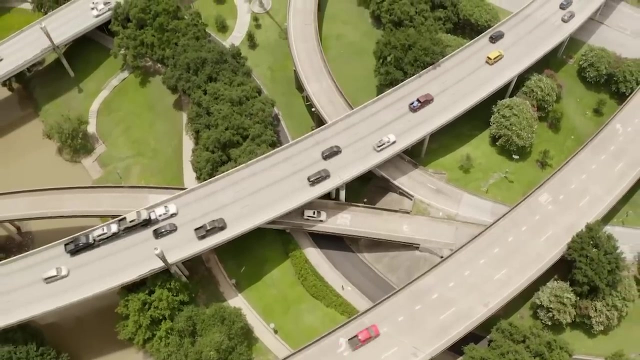 It's. you need to be saved and have Jesus in your heart, Otherwise you're going to hell. So bring something to Easter, please. For fear of going to hell, many atheists are rejected by their family. Brian had a very Christian upbringing. 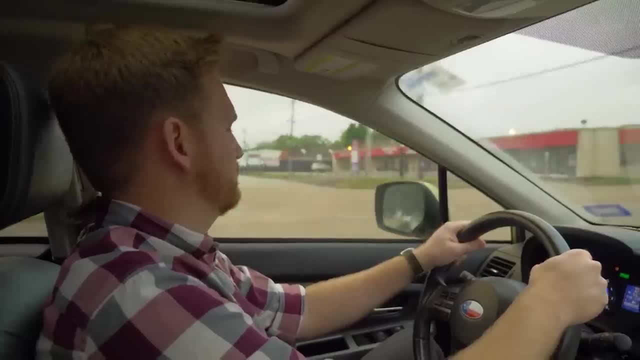 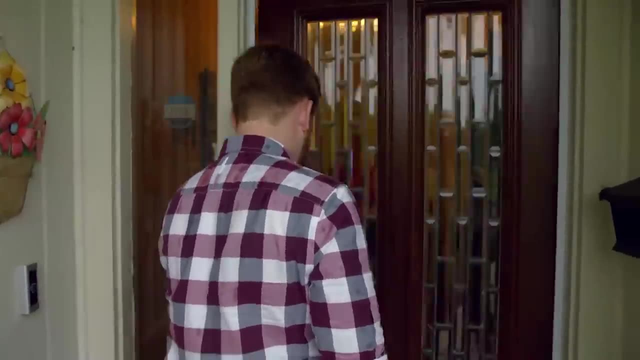 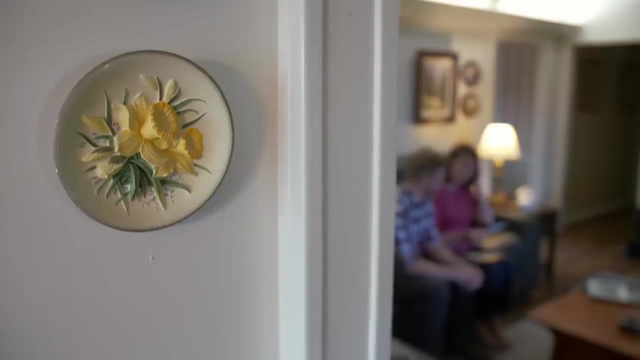 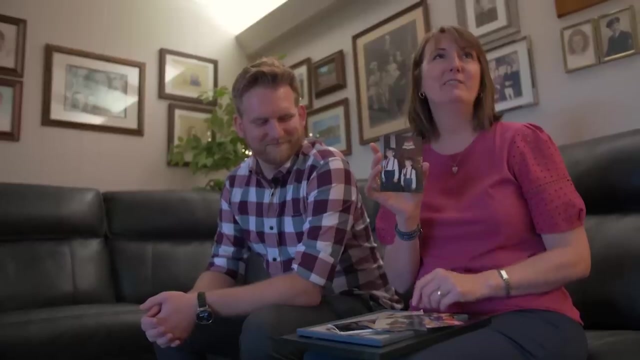 It broke his mother's heart when he came out as atheist, Although they still continue to eat lunch together every Sunday. Elizabeth has just got back from church, where she has many happy memories of her son- Look at your smile- Getting ready for Christmas Eve service at church. 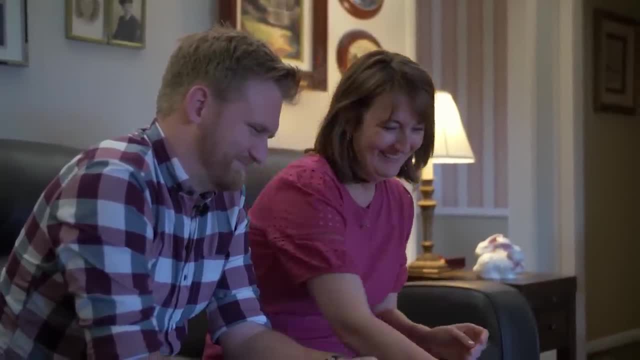 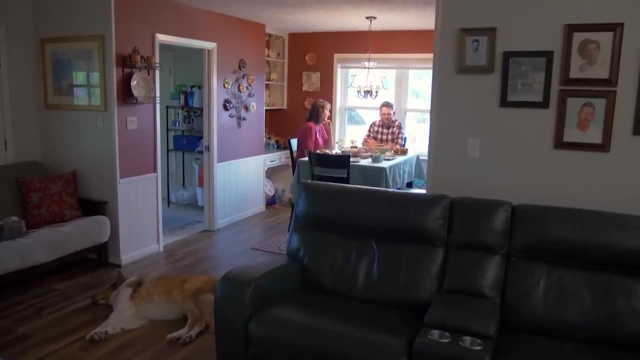 Back when he loved Jesus. Elizabeth puts on a brave face. She has exceptionally agreed to speak to us about one of the most taboo subjects in the US and one of the most painful for her. When he first told me, I think we were driving back from his college in Illinois. 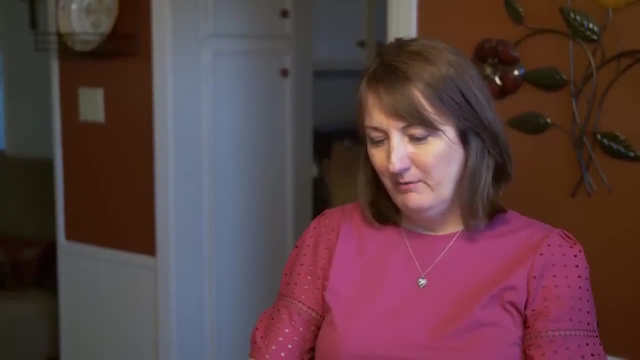 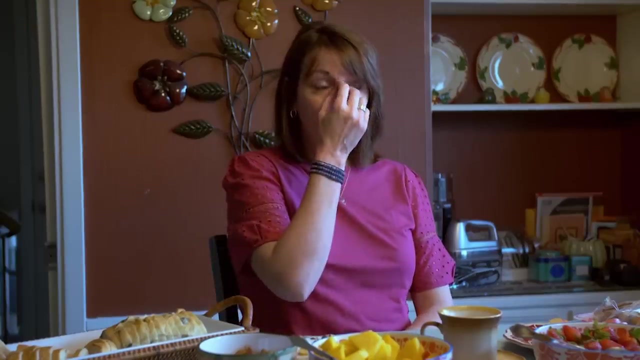 I basically cried the whole way while we talked. It was really hard to hear. I spent a lot of time agonizing over what I could have done differently, That maybe you know. you didn't spend enough time saying grace before every meal. 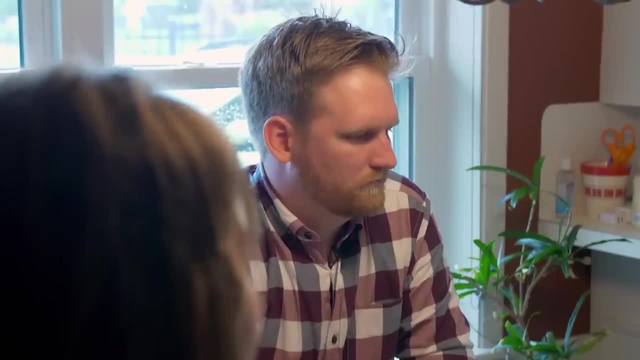 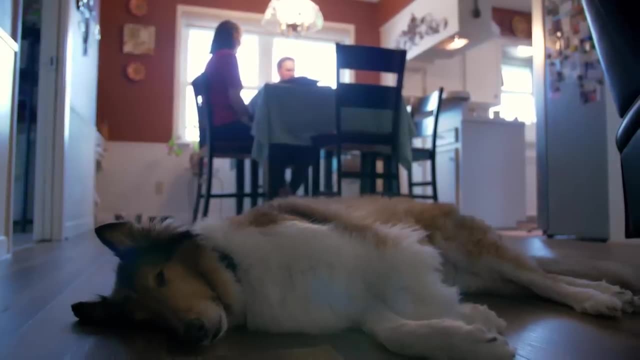 And we didn't pray at bedtime. almost all the time He was very much involved with the church. He went to a Christian college. Elizabeth's pain is palpable, but raising the subject of religion always proves fruitless. between this mother and son. 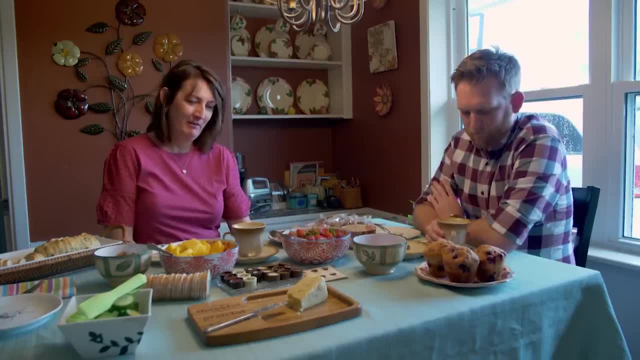 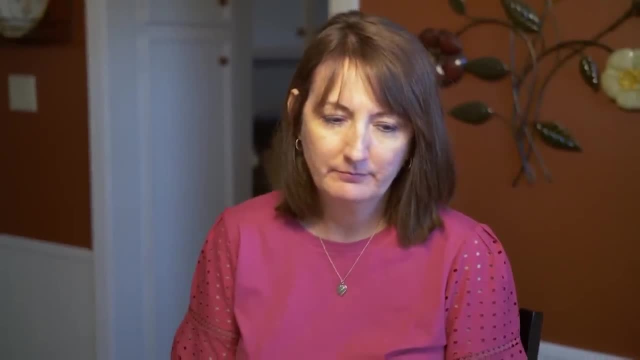 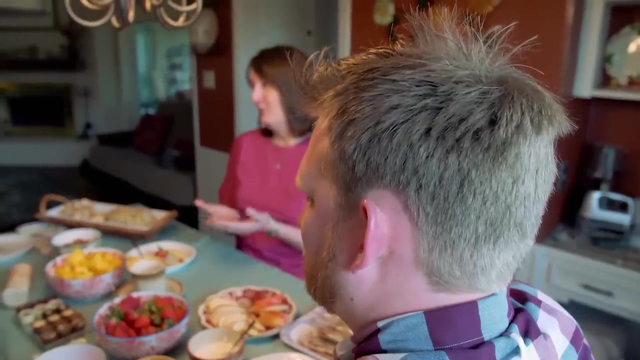 I don't know how you can study science and not see that we were divinely created. I guess the problem is, though, that, like a lot of imperfect things happen as well. God didn't make or create all those bad things, And it wasn't until sin entered the world that all these imperfections 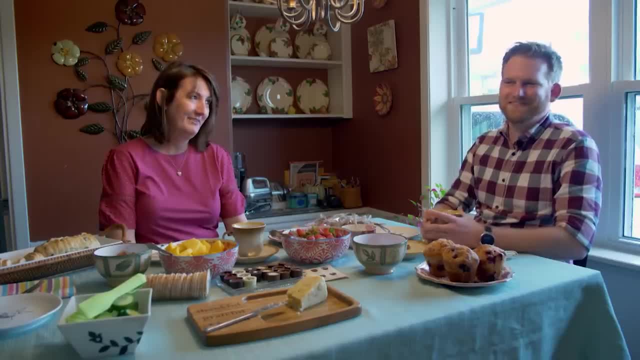 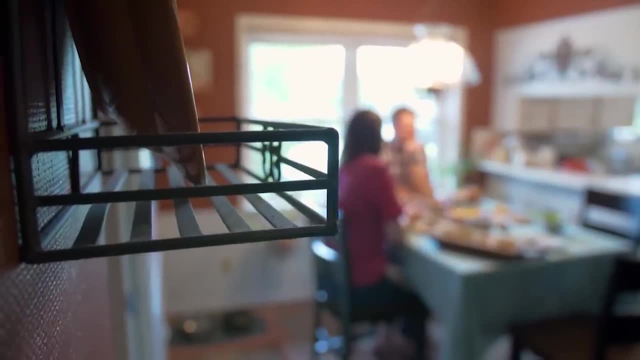 all these sins happened, But I didn't eat that apple either, So why am I getting punished for it? That's why Christ had to die for our sins. As a scientist, Brian can't seem to reconcile faith with what he has learned at university. 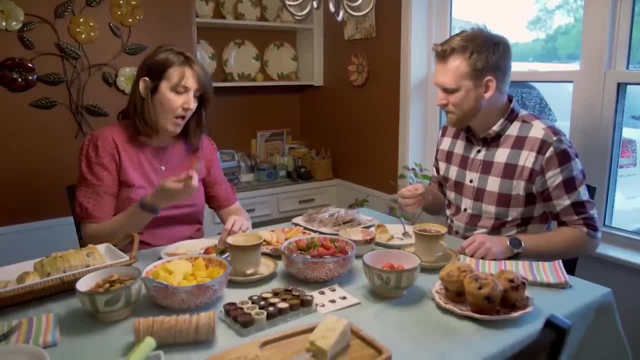 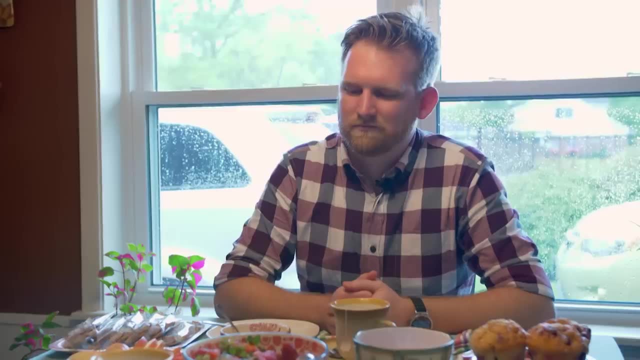 His mother shares the fear of all Christian parents when their kids turn their back on religion. Are you scared for Brian to go to hell? Yeah, that would be a concern. I don't want him to spend eternity in whatever hell is. I would sacrifice anything for him. 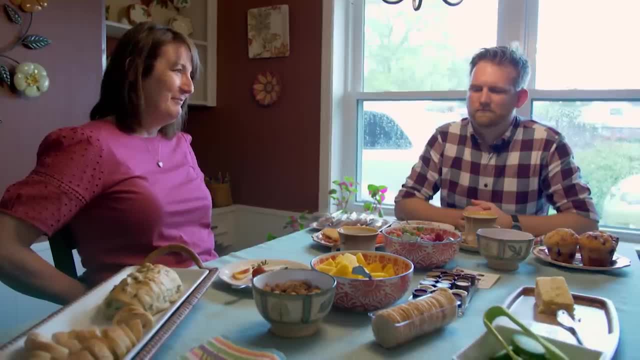 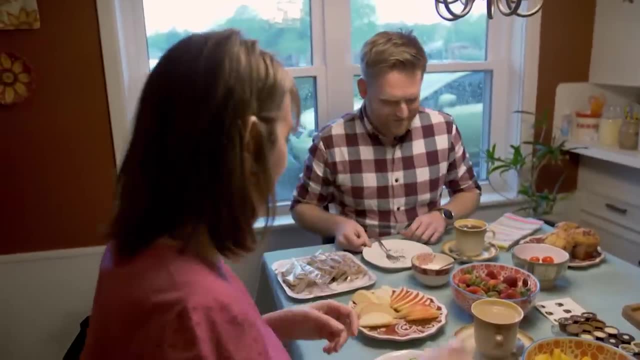 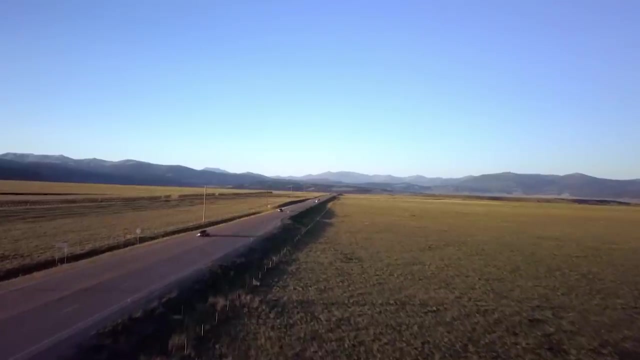 I don't want him to come back to the faith. I want it to be in heaven. More and more young people like Brian are coming out as atheists. The rising number of nonbelievers is a growing concern for one part of America. The country has never been more divided. 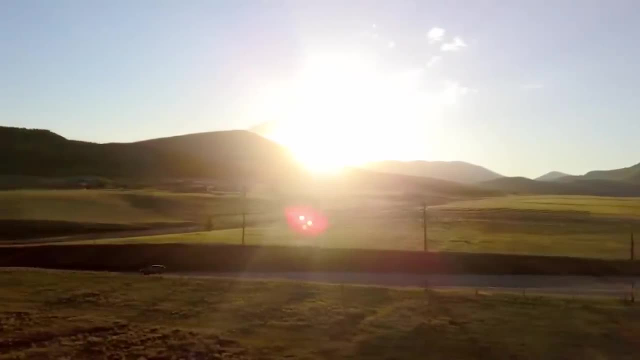 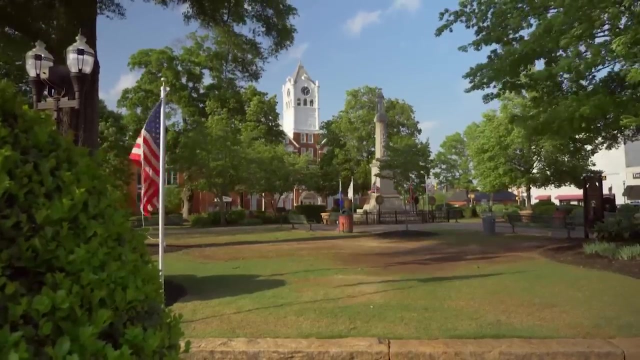 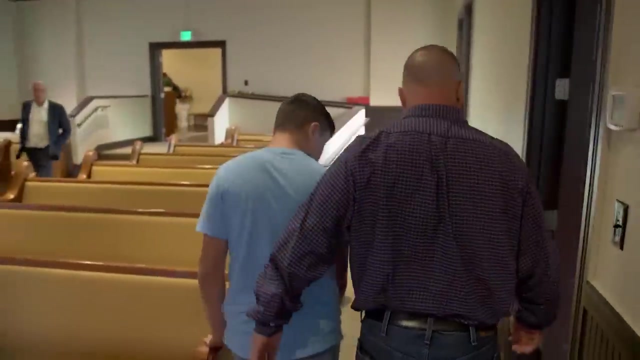 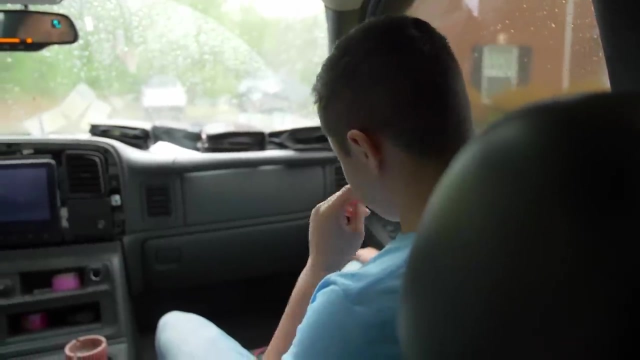 and some are even willing to use force. One example is here in McDonald, Georgia, around 30 minutes from Atlanta. Chris is a lawyer and family man. He is coming back from church this Sunday morning with his son, Ashton. And why is it important to bring your son to church? 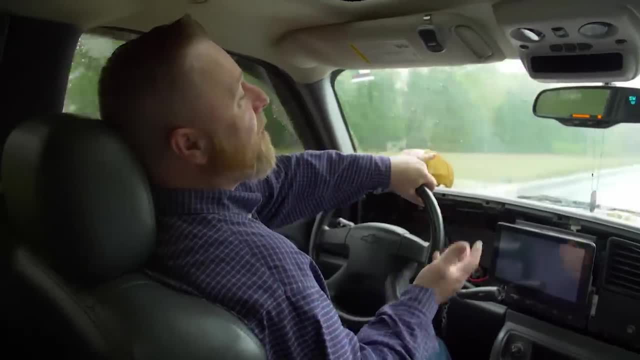 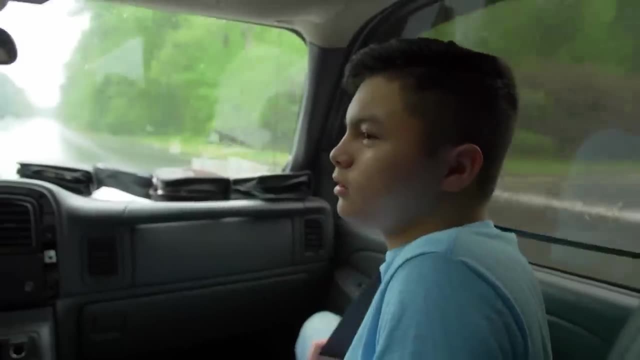 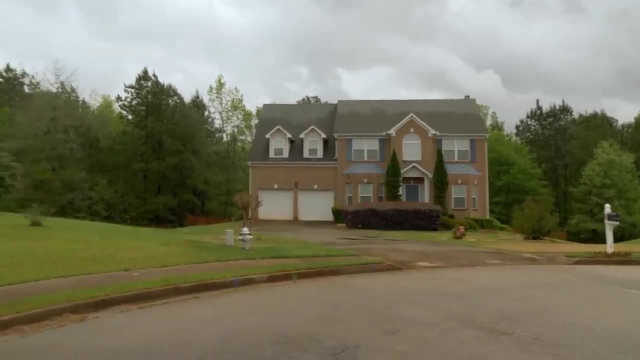 Because you know that's the order. The order is: God country, God country, family. Definitely a little bottom line. Thanks for coming. Thanks for coming with me. I love you. Chris has organized a big barbecue with friends. 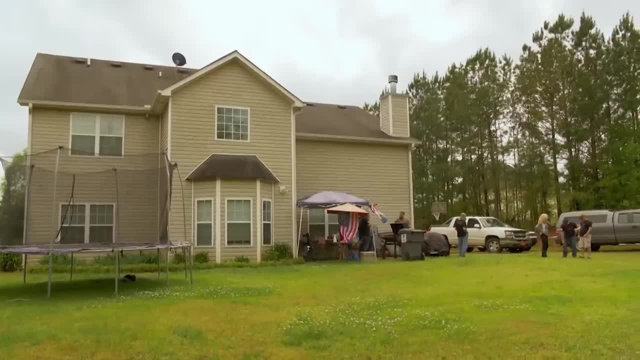 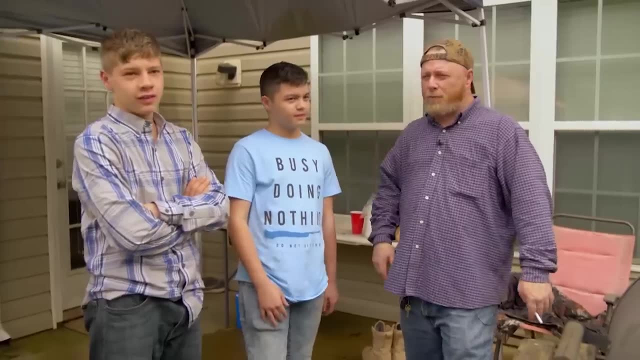 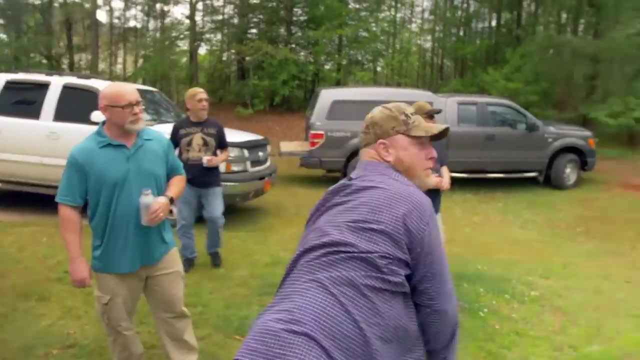 after the Sunday service: Okay, I'm gonna. I gotta ease my way into it. Holy cow, God, country barbecue, That's right. Ain't nothing more American than those three right there? right, Chris, seems like your average American guy. 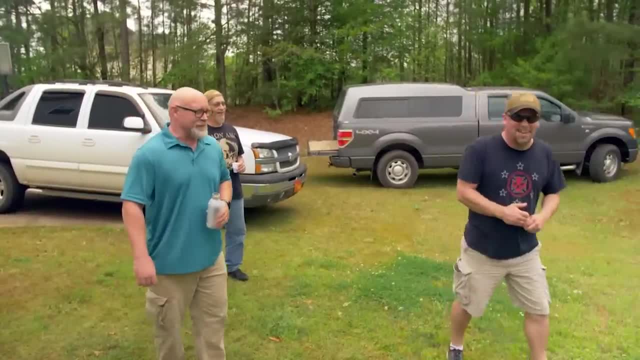 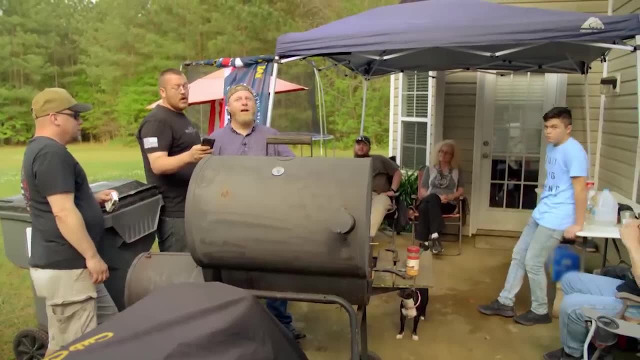 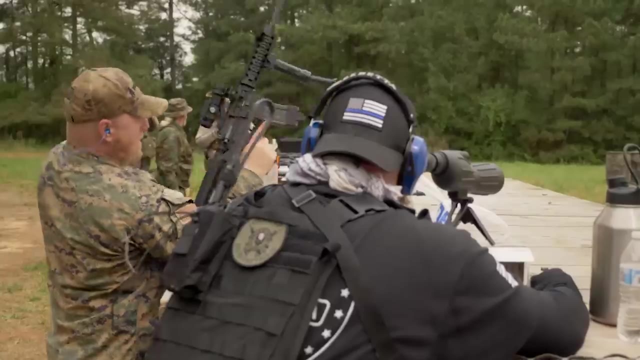 However, he's also the leader of the biggest Christian militia in the US. Everybody on site, Y'all ready? Yes, sir, Okay, One, two, three Guns up. Assault rifles, semi-automatics, silencers, pistols and bulletproof vests. 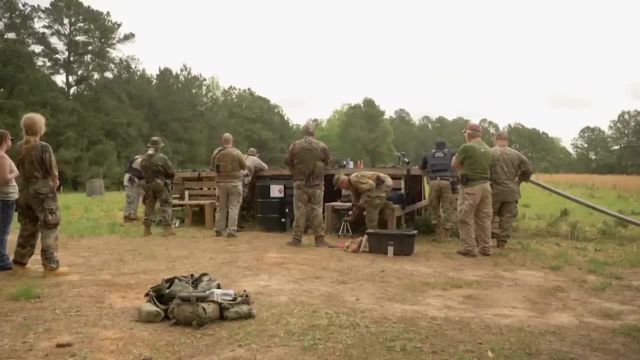 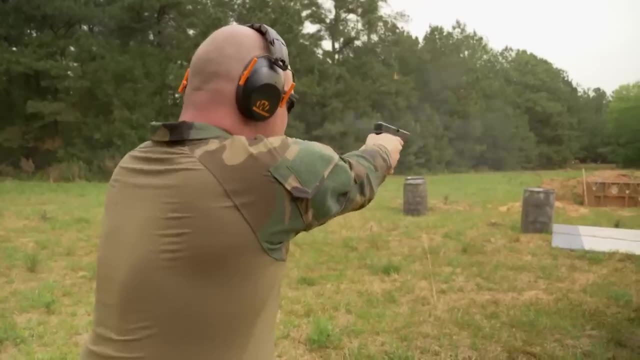 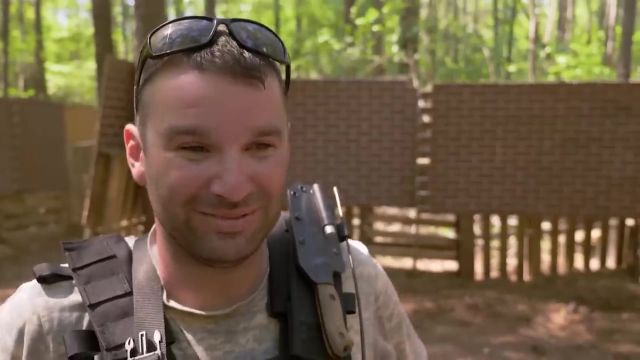 Once a month, Chris and his friends get together for military training. So sexy, Good job, baby. Yes, They're not, however, just ordinary citizens. I work at a tire shop. I'm a plumber. I do hollow metal doors and wood doors. 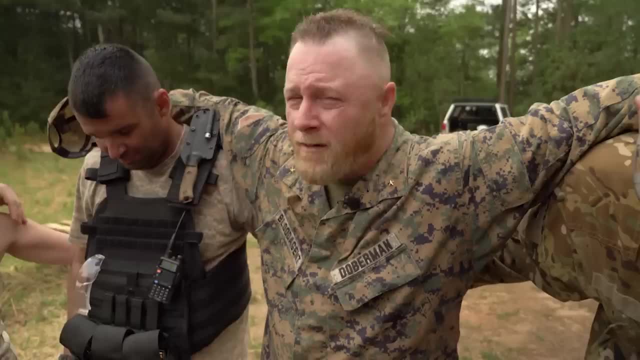 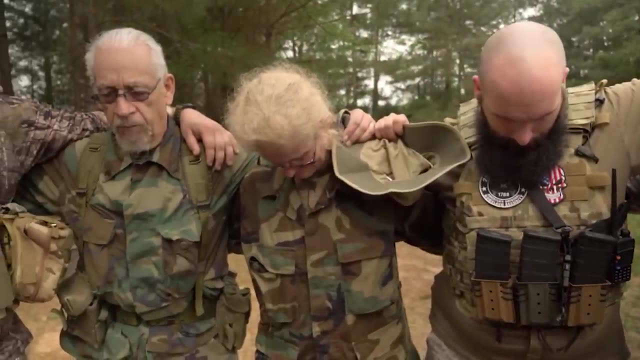 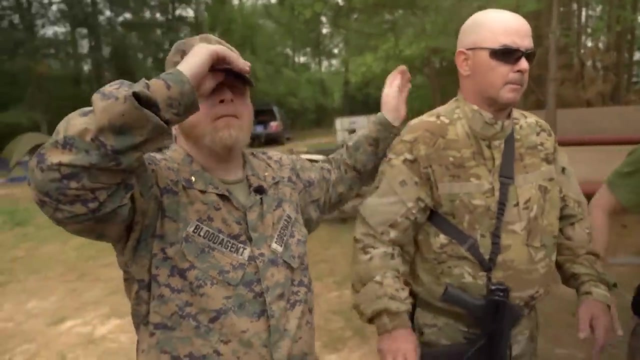 I am actually an aircraft mechanic. All are convinced their faith and lifestyle is being threatened. Look after our country, Lord, as our country starts to falter. Bring us under one nation, under God, Amen, Amen. You know, the good book says: 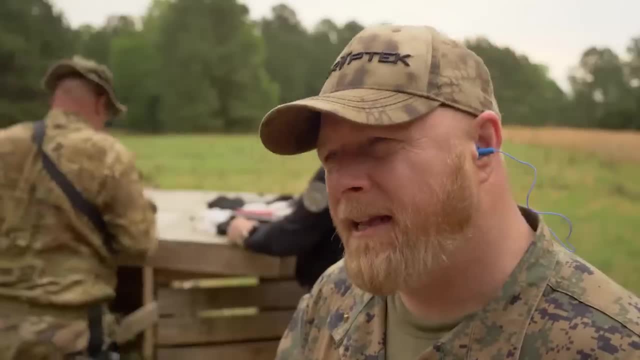 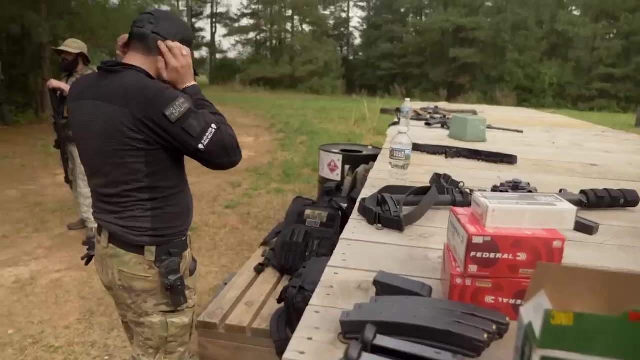 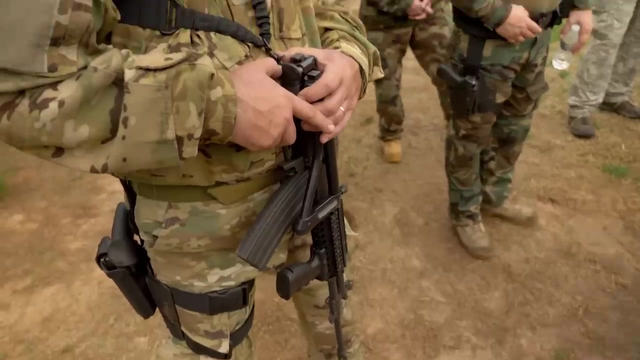 things are gonna get worse before they get better, and it would behoove us to be prudent in our preparations. So this is Bible Camp and Boy Scouts on steroids. The militia is very closely watched by the authorities. Yes, sir, There are groups like this. 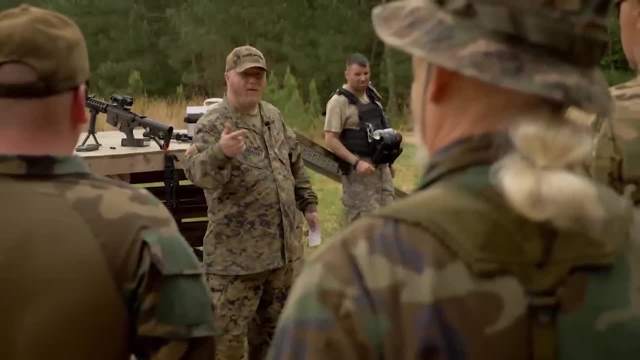 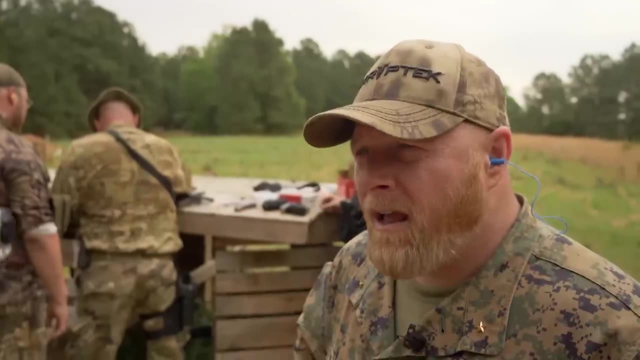 in almost every American state. We, exceptionally, had authorization to film them. Chris, however, was very suspicious. What do you think there could be a fight with? Um communism, atheism, communism- they kind of go hand in hand. 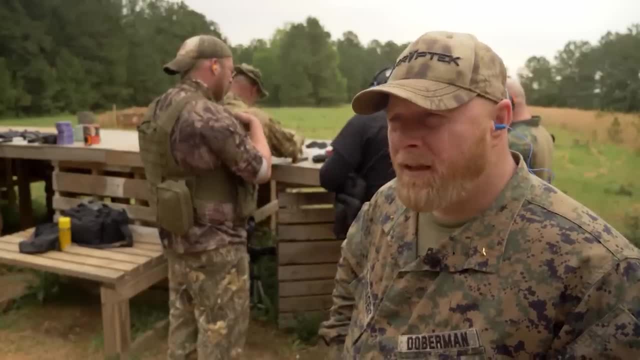 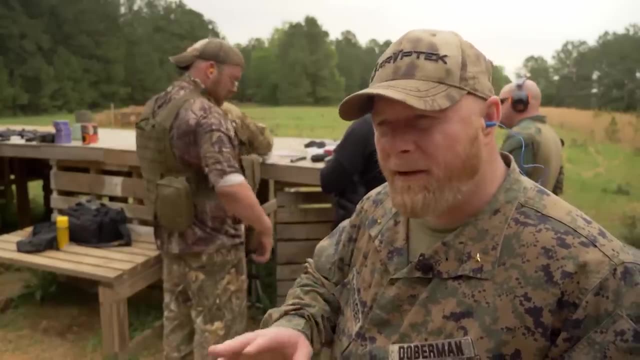 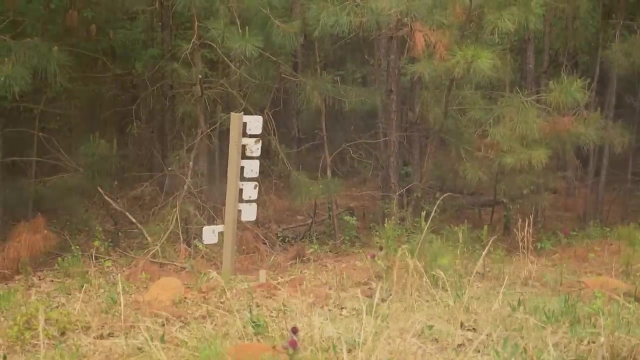 It's godless. They will shoot you, you know, for speaking freely, for you know freedom of thought, freedom of religion. They will. Communists will straight-up kill you Fire. The group trained in a top-secret location all day. 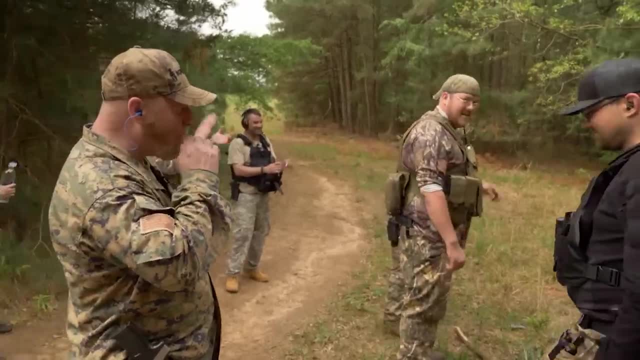 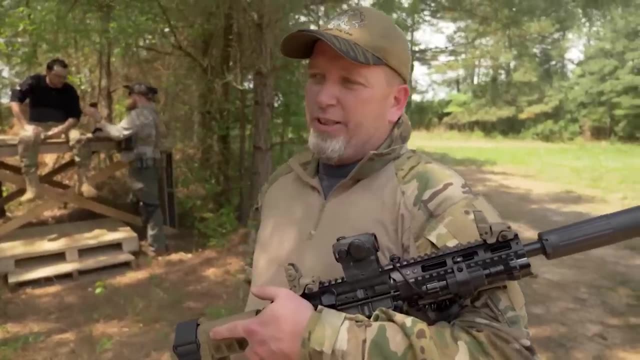 We weren't allowed to film the area surrounding the training grounds. This is awesome, Good shooting. That was awesome. Yeah, it's a Spikes Crusader lower, A customized weapon with a cross engraved onto it. Every little detail has been thought out. 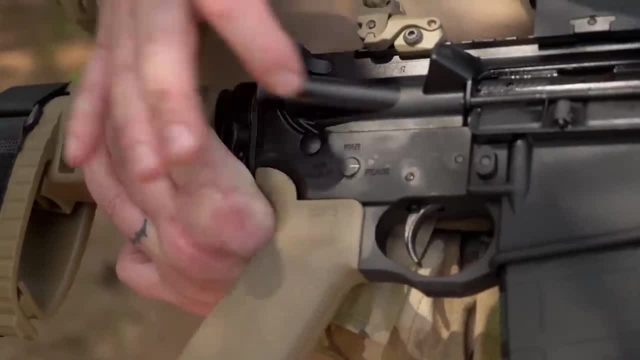 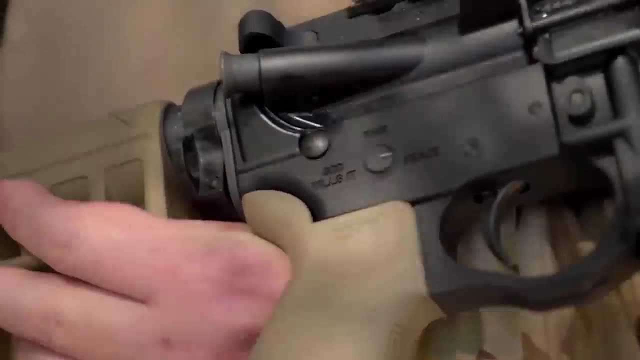 even up to the firing mode selector: Peace, war. God wills it. This automatic weapon is designed for war. in the name of God. It's the only one that requires a permit. Here's the Latin side. I'll flip it down so you can see it. 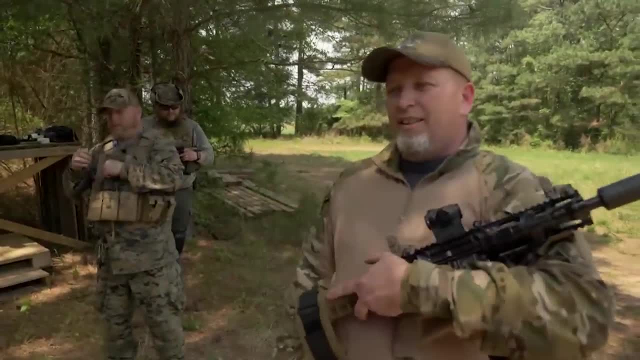 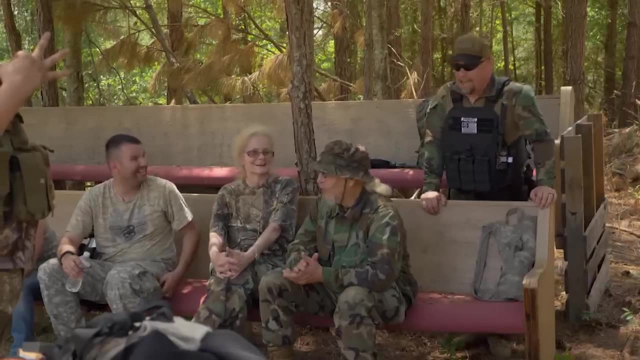 Joe got this weapon easily, as his background check was perfect: A family man working in sales. he's even a man of God. I'm actually an ordained minister. It's best if we wait a little bit. You're a pastor, I am. 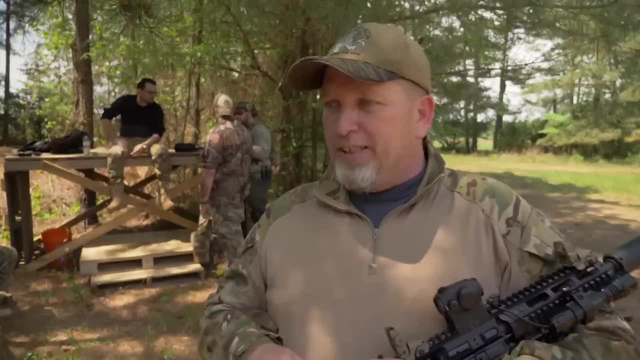 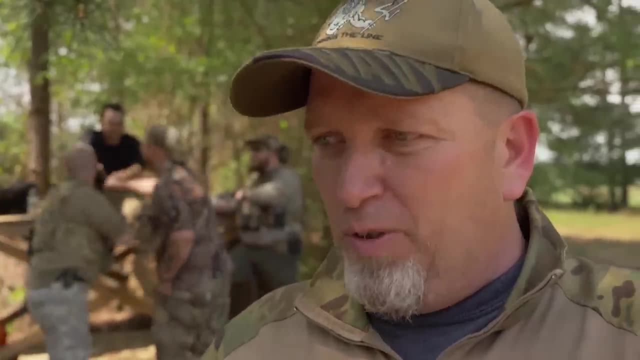 With two different churches. I can perform weddings anywhere in the country. We fight for our faith every day. You know you got the Muslims on one side, you got a lot of atheists and everybody else on the other. Where do we go? 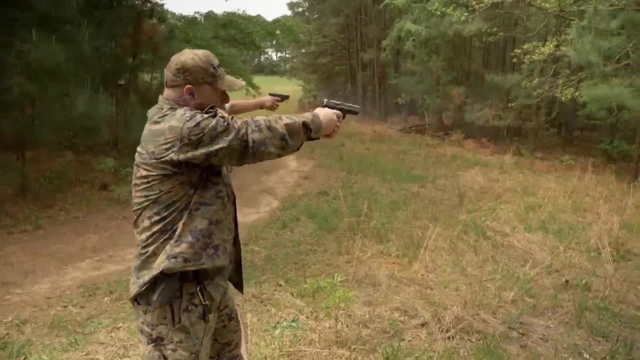 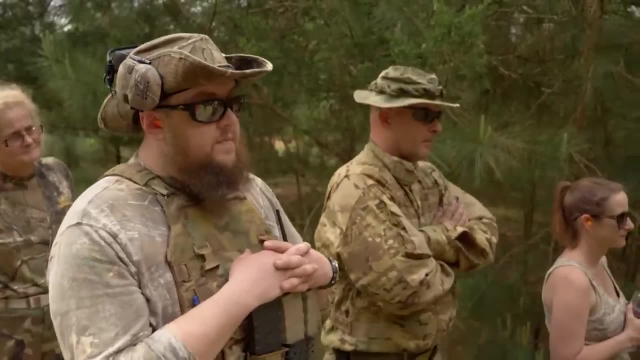 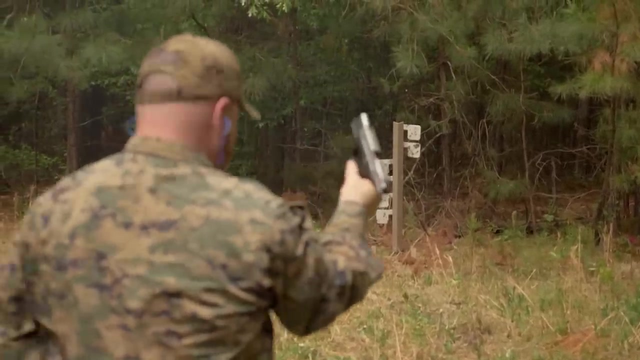 Fire. Joe is afraid of both Muslims and atheists, despite Georgia being an 80% Christian state with minimal immigration. His fears have been further fueled by Donald Trump's presidency. Oh fuck, I actually do like President Trump. I voted for President Trump.